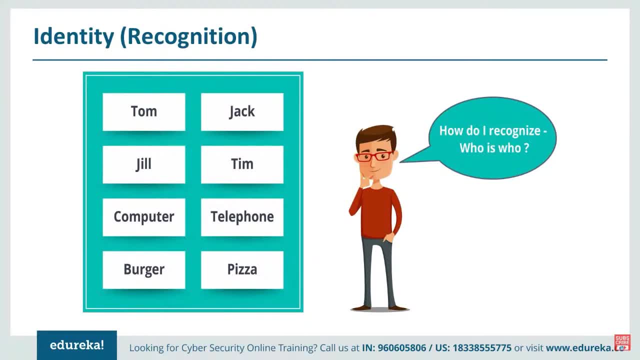 us, even the computers, is just to recognize user from an object only by a name: a, a, a to. we'll also discuss on the common naming conventions. so when someone with the username of jack or tom or jill or anyone, because there might be obviously a possible of having multiple- 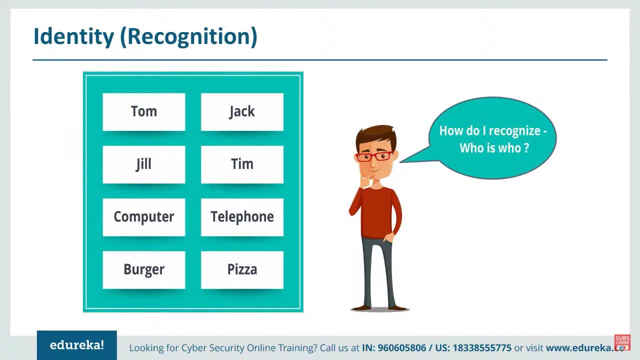 toms, multiple jacks, multiple jills, or i mean multiple a's, can be in a simple organization. so what will happen is: whenever computer generates a object, we call it as an object. even username or user account is an object. computer is also an object. telephone, the index is also an object. so every time when an object is created, a unique security identifier is. 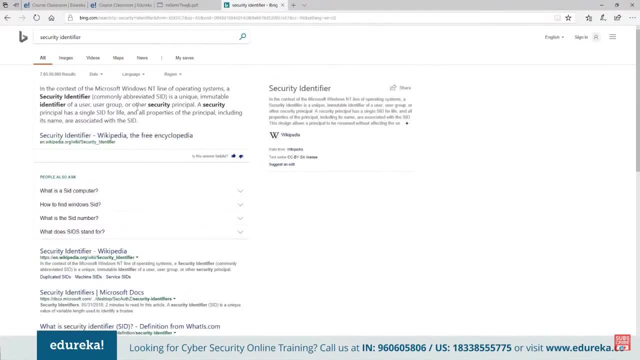 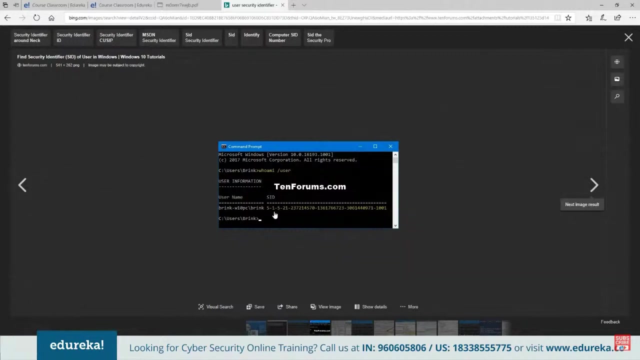 generated. the security identifier will be like an alpha numeric string. it actually likes a, not only with the names, any name, user security identifier, for example. do you see the text in yellow? it's s hyphen 1, hyphen 5, 2, 1, hyphen 3 and so on. it's a combination. 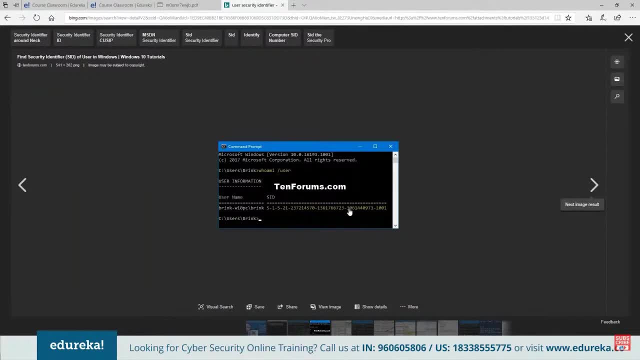 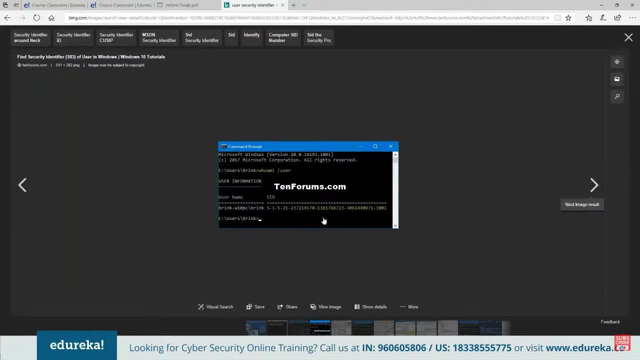 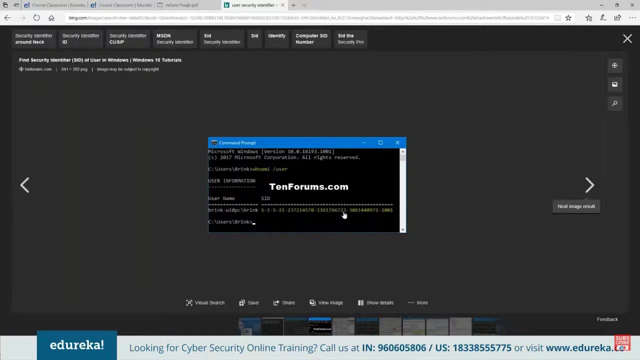 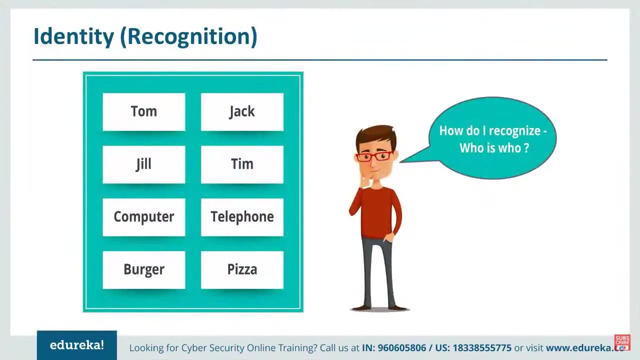 on example of username brink. the username brink has a security identifier of sid of this value, so whenever the same sid will not be assigned to other jack or other brink or other jill, it is unique and it is more static. it will not change often because when an account is created, 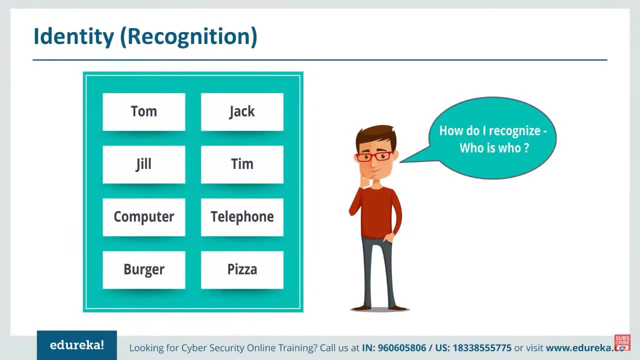 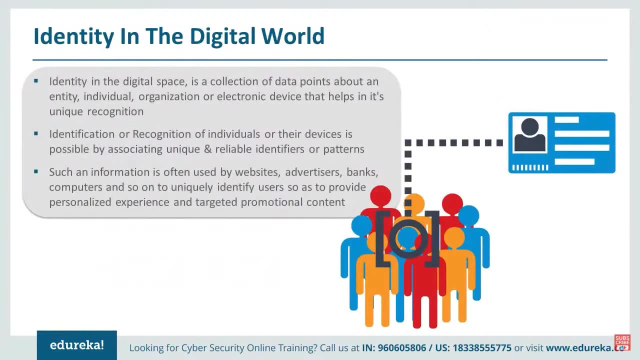 It will be assigned particularly for it and it will be removed Once the object is deleted. in computer terms, the security identifier is generated, and also for physically recognition, We have multiple real-world scenario which comes in the physical security, the ID cards which we always you used to access the doors. 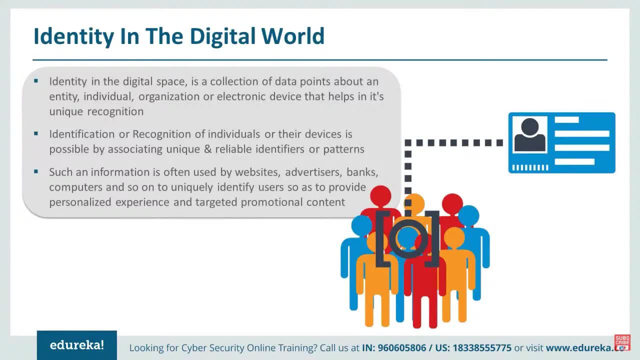 that are near field communication. What we also have it is in the debit cards, the latest access cards which are enabled with NFC, which can be accessed only within a range of four to three. I mean three to four inches. So when we go beyond that it will not work. 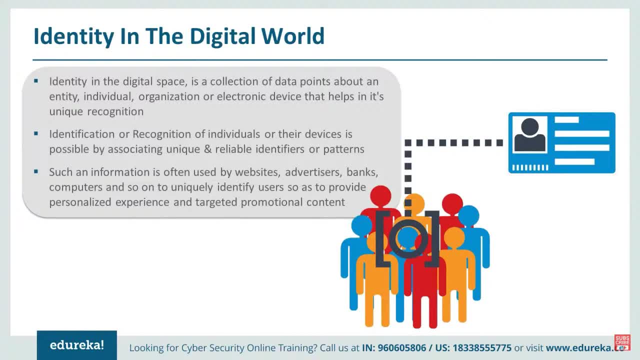 So the identity is not only for users object. any software- I mean any hardware or any kind of service account or any object which is inside a digital world- will have a unique ID. Those will be also called as GU ID or you ID. The databases are stored in a key management system. 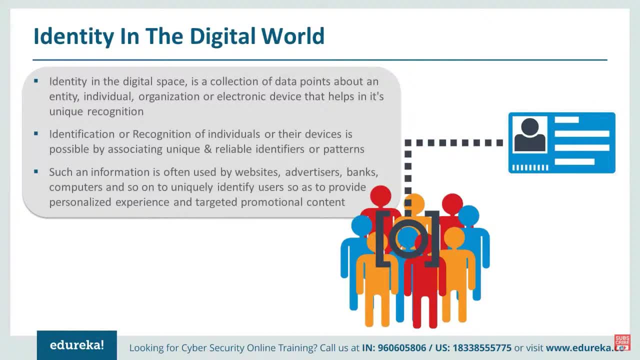 Actually That's a key management system- will be encrypted zone. Most of the password stored in the key management walkie-walkie will be in the hashes. It will not be a plain text or a directly encrypted text. It's a hash value. 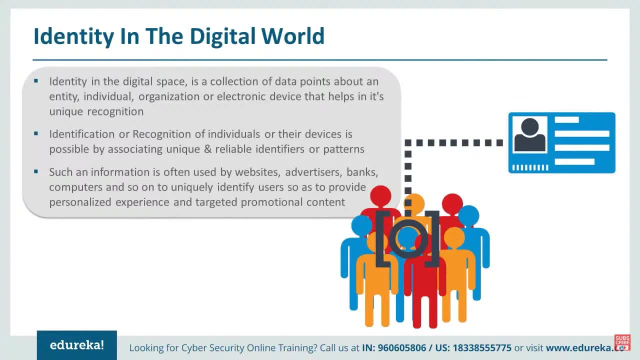 It may be a passphrase or it may be a complete paragraph. The password maybe are even a few few characters. when the password is digested It will be generating a hash and those hashes will be initially managed. I mean that will be used To verify whether the user is giving the right password. 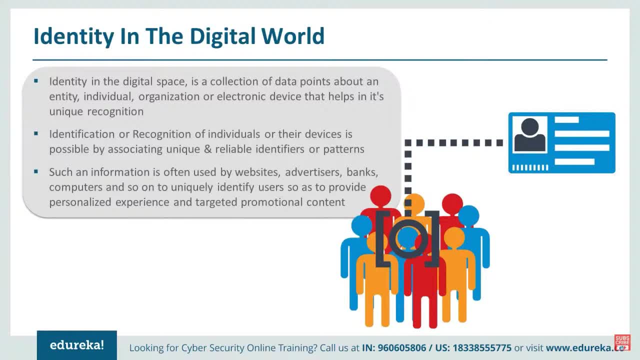 or not, but the exact password which is stored, created while the user during the users actions, that will be highly compressed and that will be also encrypted and store. the actual encrypted password, will not be accessible over the network or directly by accessing the physical machine, Even when hacker technology 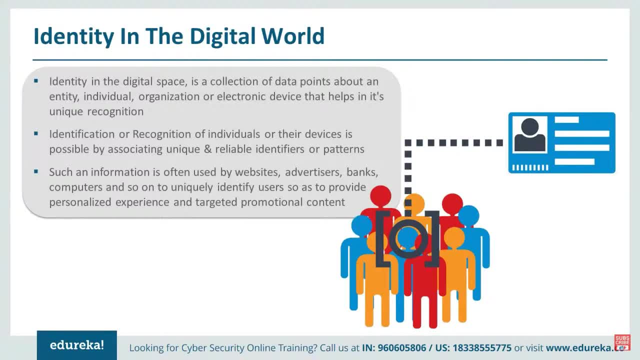 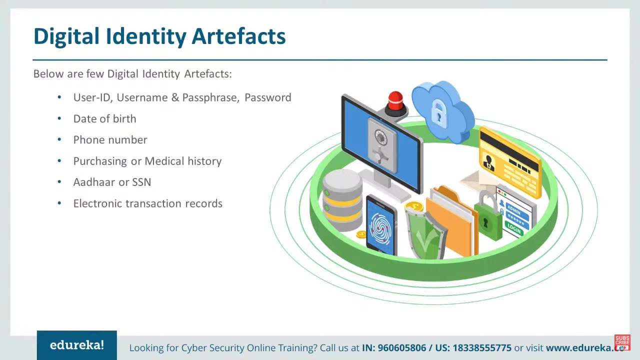 which Microsoft right now uses its care Bros, and it's much more secure. and even when we have direct hands-on The Kerberos, we can have the hash values, not the passwords, directly. So what are the digital artifacts? So artifacts are any result of a particular action. 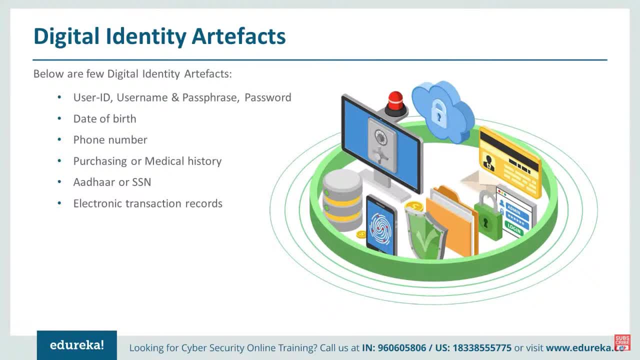 by particular training thing or a particular object. What are the possibilities? or what could be a digital artifacts? or when we create a user account, we obviously will create username. We will be providing a option to create a passphrase, So obviously a unique identifier for the object. 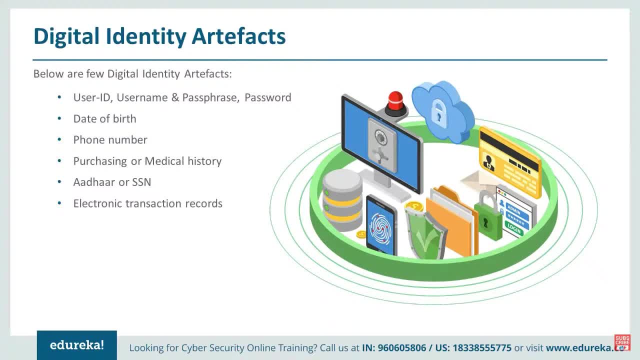 So digitally, even a date of birth, phone numbers, your other card numbers, your social security number, your transaction IDs, anything and everything which was generated in digital means are called digital identity artifacts. So when talking on the SIM, any even generator, on the SM, 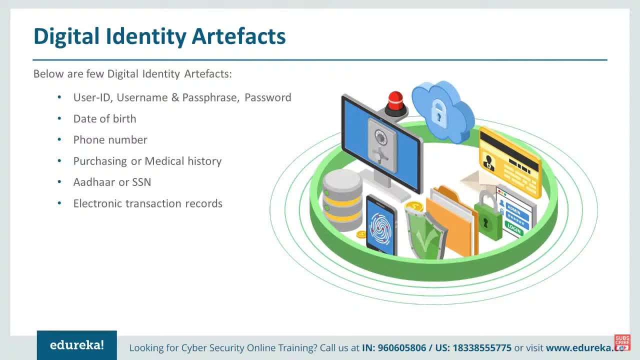 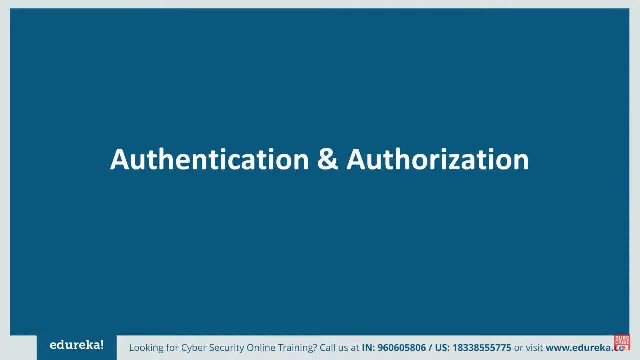 that also will have a event ID, So any transaction should obviously have a identifier for it. So authentication and authorization. authentication is means validating whether the user is actually available in the system or not, And if the user is available in the system, whether his credential 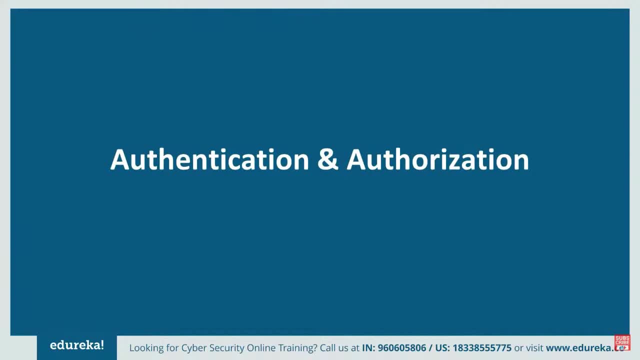 or authentication method is successful or not. The user may have a single factor authentication. that a single factor authentication just by using username or a password username, a pin number, username and passphrase or username with the OTP. OTP, That's single factor. multi-factor authentication is nothing. 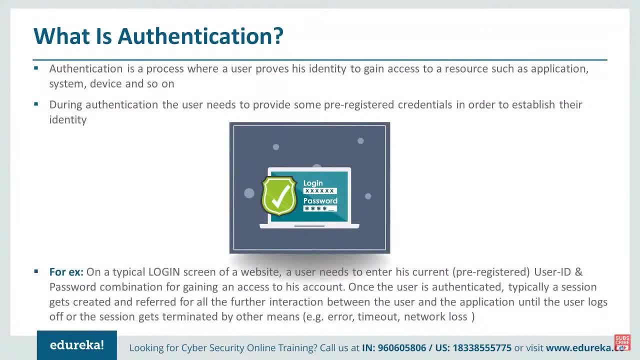 but using multiple combinations. as I already told you, what you know is a username and password. what you are, It's your biometrics: your iris scanner, retina scanner, your palm scanner, fingerprint scanner. These are what you are. You are actually what that is called a one of the other factor. 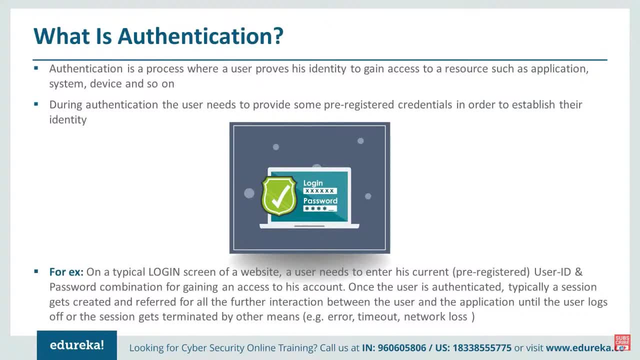 and what you have would be your access card, your smartphone for receiving an OTP and where you are, which location you are, what you do. that will be your signature, your speech recognition, voice recognition. These are the multiple factors can be included in a combination, So with two or more factors included, 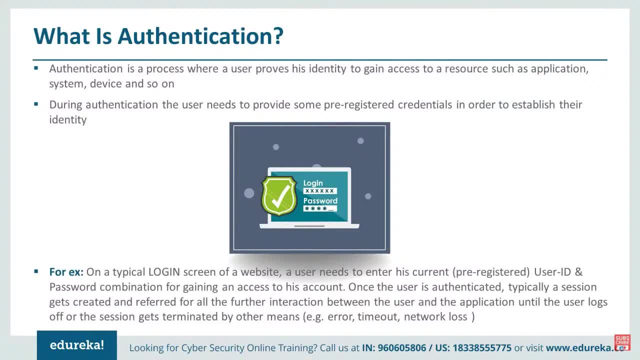 for a single authentication. It's called multi-factor authentication. So the authentication process, initially to identify which object or which user is trying to authenticate into the system, initially just validates whether in the existing record if the object is available or not. if it's available, whether the input and password or authentication authenticator. 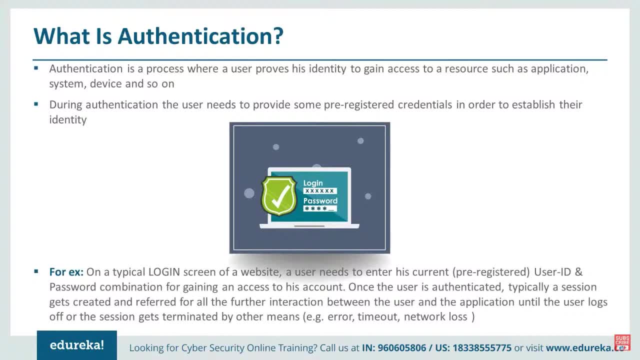 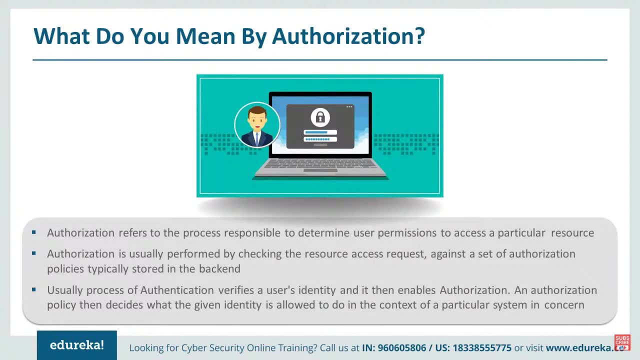 is valid. if it matches, it then moves on to the authorization level. So what do you mean by authorization? This is a question. what we did so far: we identified, we verified the person, verify the identity of the person as a network administrator or a security professional. 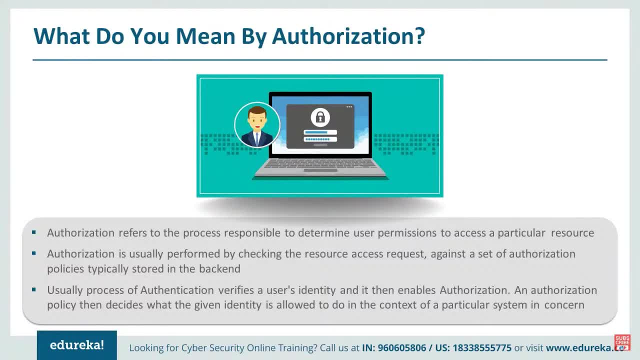 What is the value add he can do apart from relying on standard operating system and application password? password encryption instead of using a single factor? authentication using a multi-factor or combination of factors. That's one of the good practice and always nowadays, the passwords which are used inside the network- most passwords. 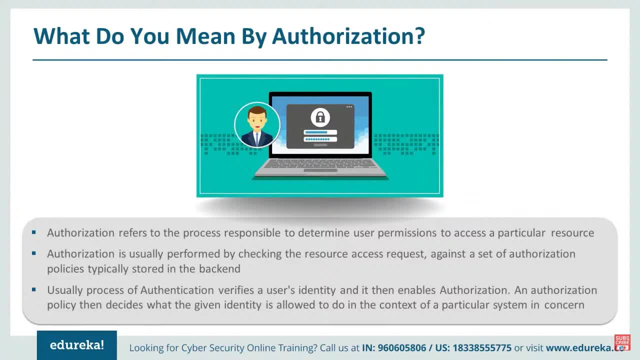 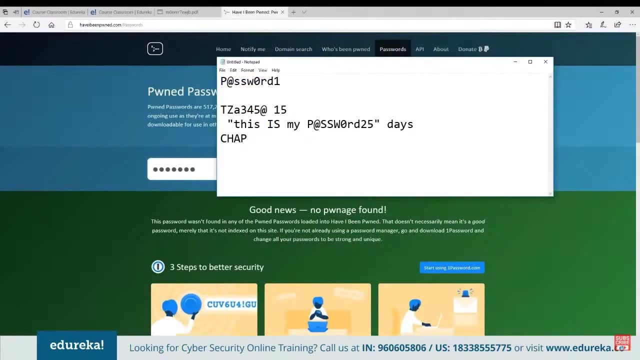 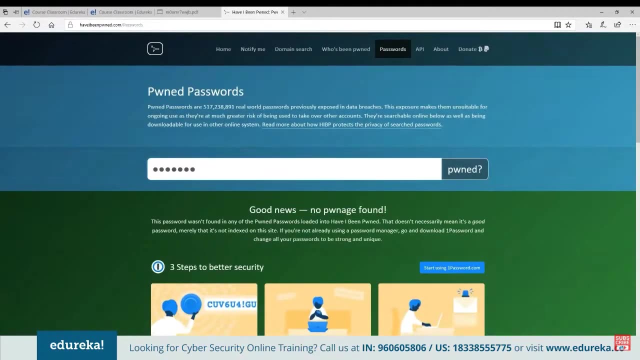 and sessions are becoming tokenized, So nowhere we are laying on passwords. For example, we can talk about heap because there is one of the challenge has to let me get the list, So I'll explain you. What are the protocols? What are the protocols it used for authentication? 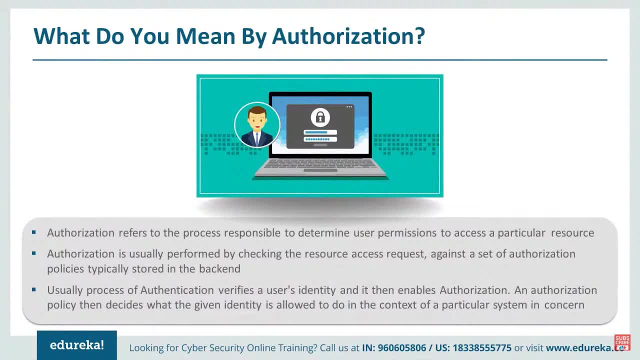 There are plenty multiple, so authorization Is actually once the person is identified and he's authenticated. authorization is the face where we decide what are the rights a person poses and what are the object he can access and what are the actions he can perform on a particular object. 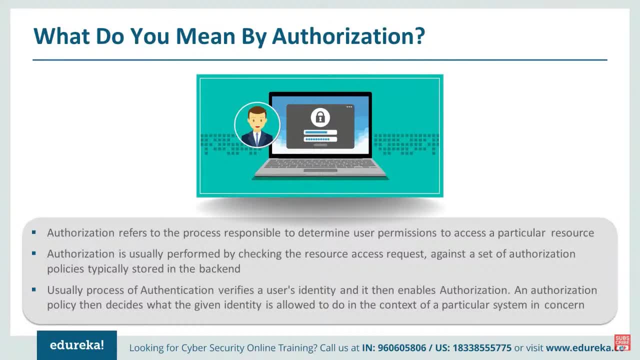 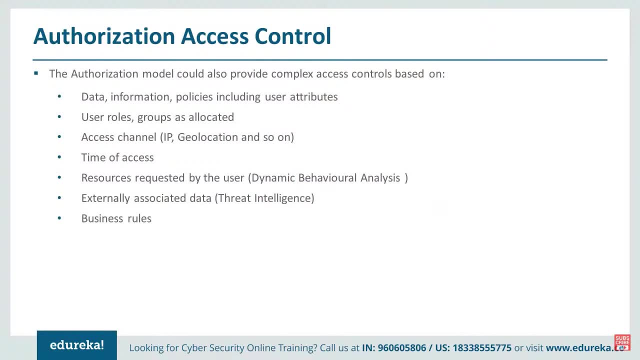 So everything will be determined and assigned during this phase. This is called authorization, So the authorization control can be also based on multiple factors and multiple controls or multiple Attributes to be taken in the consideration. So when a user logs in after business us, we can decide what time. 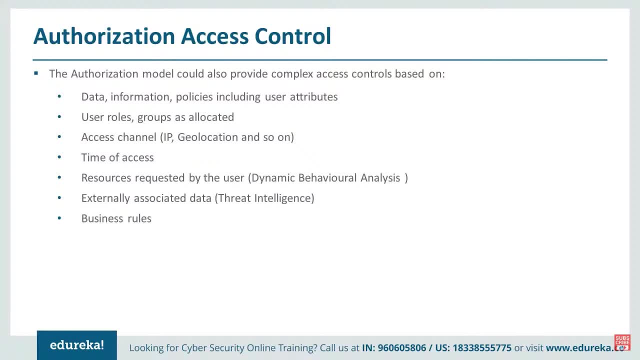 the user needs to be provided authorized. He should be authorized to access the computers. when a business is functioning from 8 am Or 7 am In the morning till 5 or 6 or even 7 in the evening. The user can able to log in user only from the 7 am. 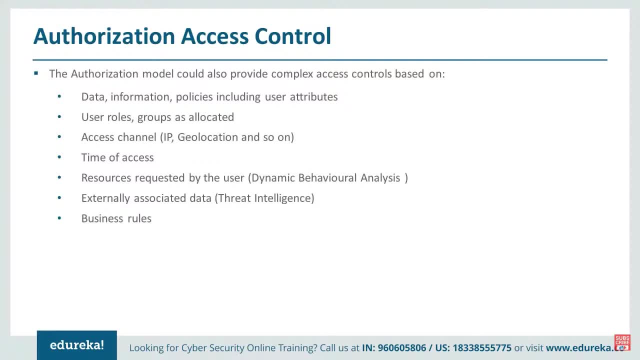 To 7 pm. If the user tries to log in beyond the business, as we can set a configuration, the user should not be accessed. So the initial the authorization phase will be over, because it will obviously reduce the amount of time as security event. 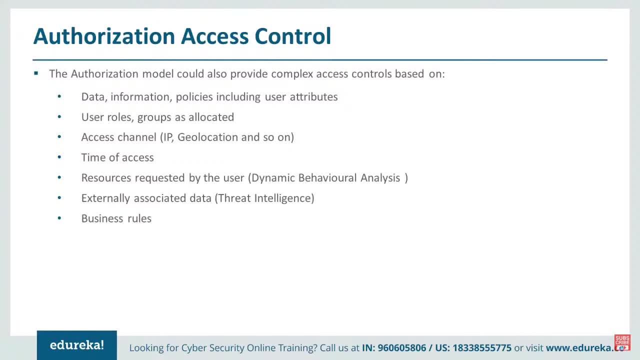 I mean event analyst, will put into if an user is not logging into the system post 7 or post business, as there will not be an event which are created by a user and which should not be suspicious, and when the user is not active or active in the system, only the regular. 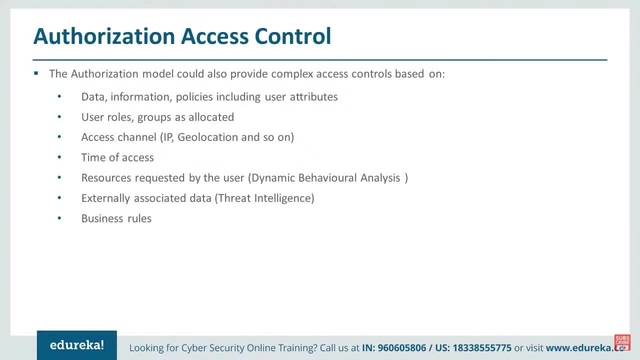 functions are any scheduled task or scheduled backups or scheduled updates That will be running in the system and that will be at the amount of logs which are generated during those system will be. those time will be lesser, So the lesser number of logs to be analyzed- and obviously this is one- 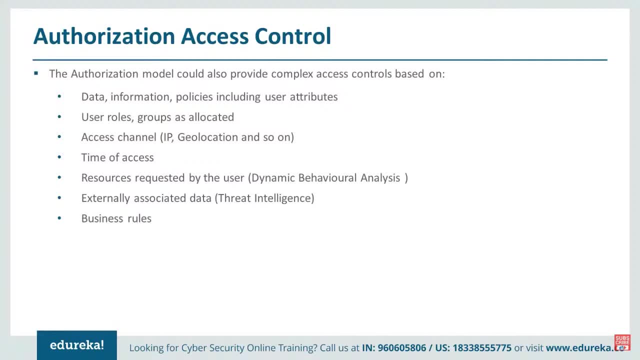 of the way we can reduce the amount of logs into the SIEM, and also based on when the user is trying to log in. for example, if a user already logged into a system and he wants to try logging in from a multiple system instead of accessing multiple, authorizing him multiple times from multiple. 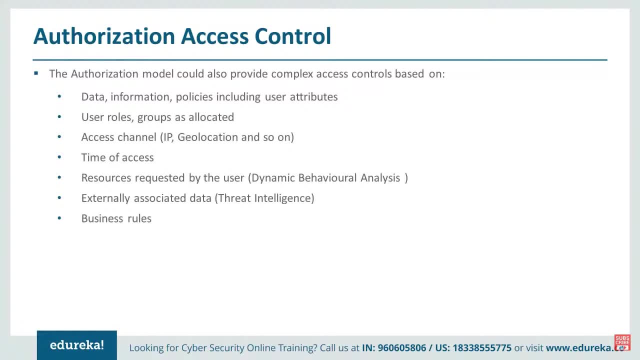 computers. He can decline or deny access from simultaneous sessions or multiple sessions, or is just terminating the one session from one computer and giving access back to the latest computer- I mean most recent computer which he tries to log in. these are simple controls We can implement into, so the authorization factor is up to the security. 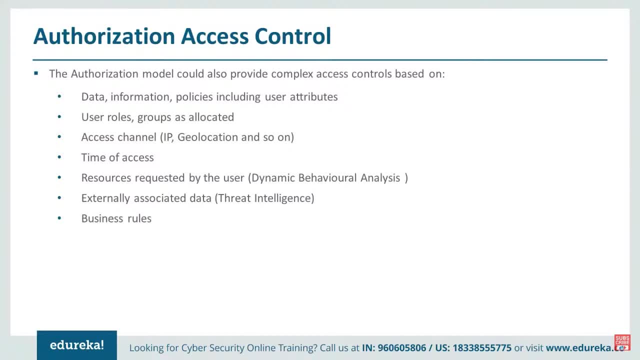 administrator and the security team and even a system administrator or network administrator who gives access, he can follow the simple practices- I mean best practices- prescribed by sans or nest, even from, I think. I'm not much into the network devices, but I think I have seen somewhere in fire. 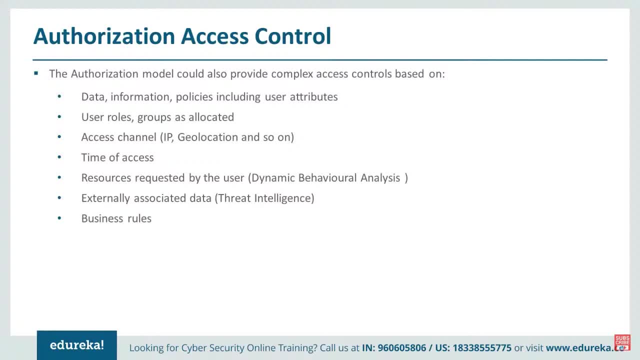 I based an article which I think I read, that also gives the best practices, what we can follow on the network devices or network based authorizations, and also setting up the access channels just to all of access only when a user tries to come and connect from a VPN or from a particular geolocation. 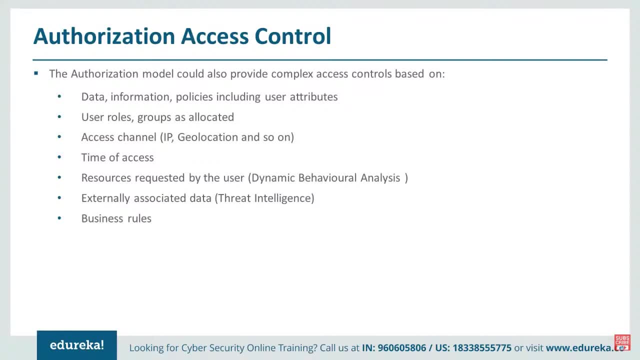 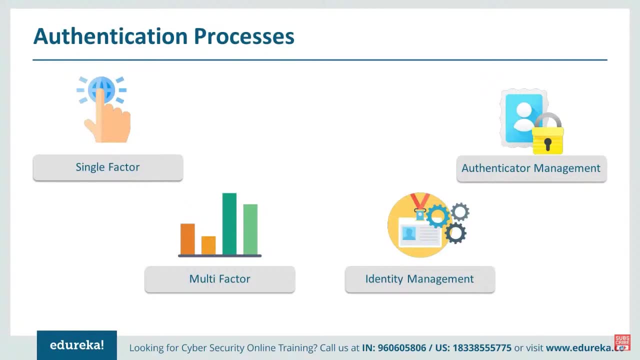 So the access controls can be Crafted as per the requirement of our business. So what are the authorization and authentication principles? What are we implement? We use single-factor authentication. multi-factor authentication- I mean combination of multiple authenticators- is called multi-factor. 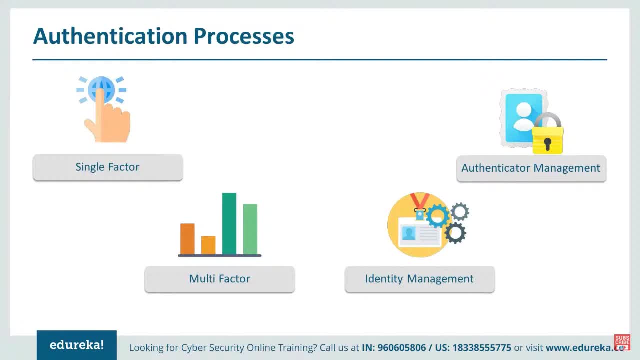 authentication, the authenticator management. the authenticator management will come into play. the Kerberos LDAP radius, tachax, tachax plus diameter, Etc Multiple will come into play. These are the things which help us in managing the proper authentication and identity management suites. 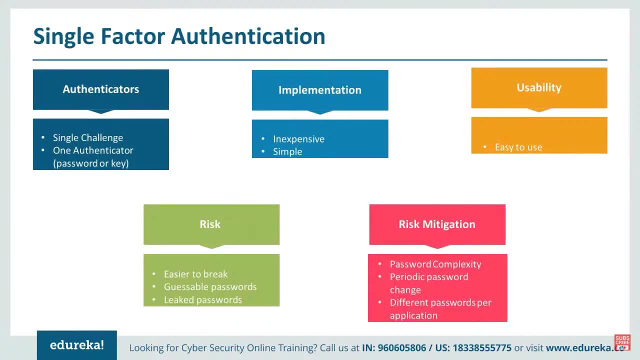 So this explains the same single-factor authentication. What is a single-factor authentication? a single challenge or a single password? What is the implementation cost? It is very inexpensive and it is simple to enable and simple to use. There is no additional configuration needed. 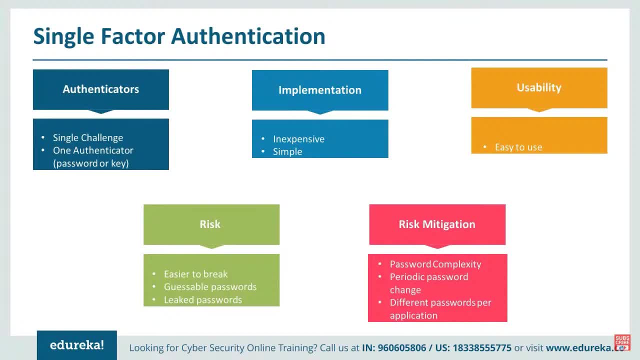 It is easy will do, but what is the risk actually involved in it? the password can be easily guessed, or the password can be easily eavesdropped, or it can be even viewed from the- I mean shoulder surfing- to be saying obviously people can see what passwords you type in are basically. 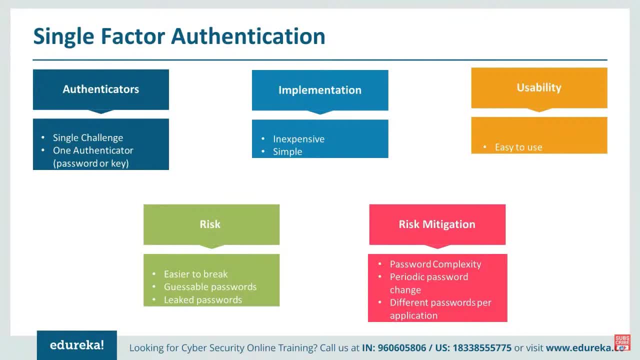 people will have predefined at pre-used passwords. Some people even forgot to change the password once they receive them, and every enterprise or every organization have a habit of providing a unique password or the same password to multiple any and every user password one, a default one. 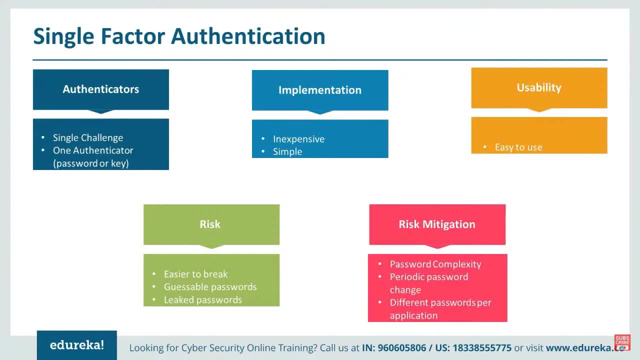 User 1, user 13.. These are common passwords which will be given on to all, but what happens when a user forgets to change the password after he receives it? It is easily guessable and any, even his, one of his colleagues could try logging in. 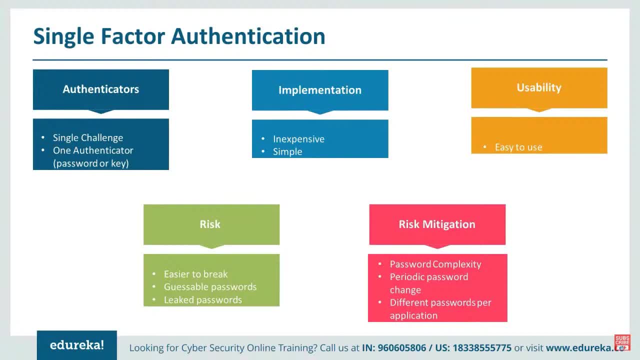 So always is, best practice is to change the password when, once we receive it, and not to use the default passwords. It's a rule. We have to take it as a rule, Even if it's an interactive, as a basic router, switches or be whatever it may be any device. 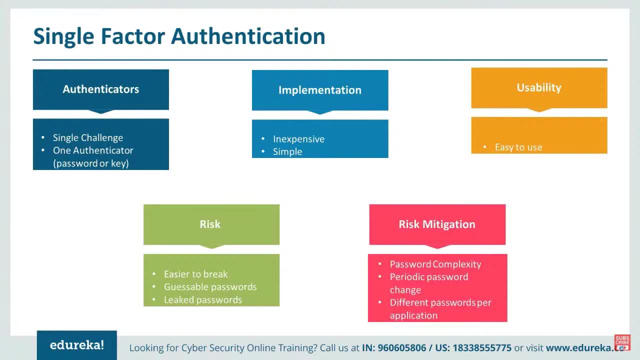 which comes with the default password. Please change it when you start using it. So the risk mitigation: what are the things we can do just to solve this? we can have a complex password. instead of password, We can have a passphrase. a passphrase is nothing but multiple words, or even a, if you're okay. 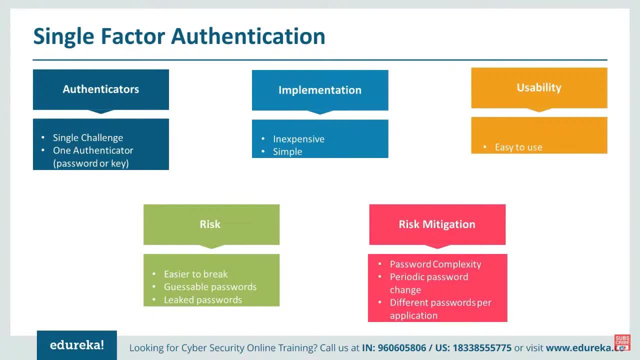 to type. you can have it a paragraph. So the periodically changing the password, how often you need to change the password? a single password can be used for 30 days or 60 days, maximum of 90 days. I did not I've seen a scenario which a password is allowed to be used more than 90 days. 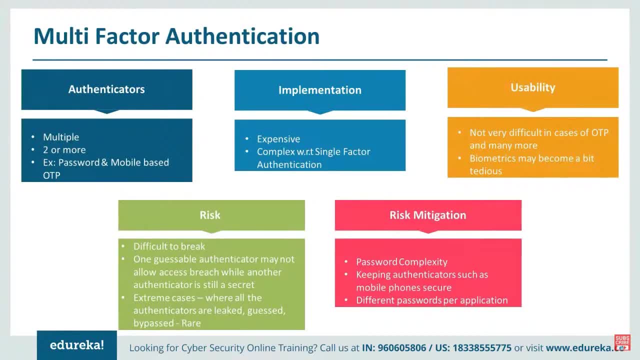 So multi-factor authentication? multi-factor authentication is using multiple factors, multiple authenticators to grant access into the network. What is the implementation cost? the implementation: It's expensive because we need to implement any third-party applications. We we need to configure additional server for providing a two-factor authentication. 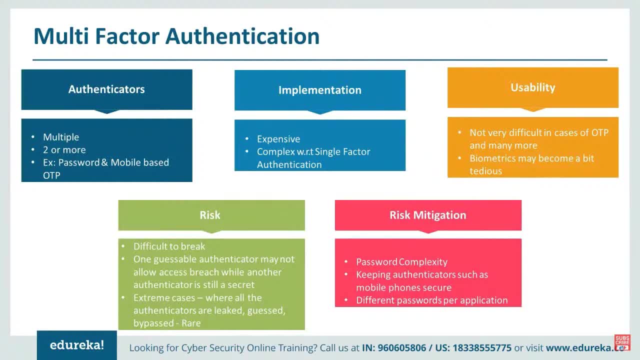 mechanism to function properly, So there is a bit complex. then, using a single factor authentication, What is the examples of usability? So are you mixing up with your biometrics along with your passwords, receiving a one-time password? So what is the benefit of having a multi-factor authentication, benefit of multi-factor authentication? 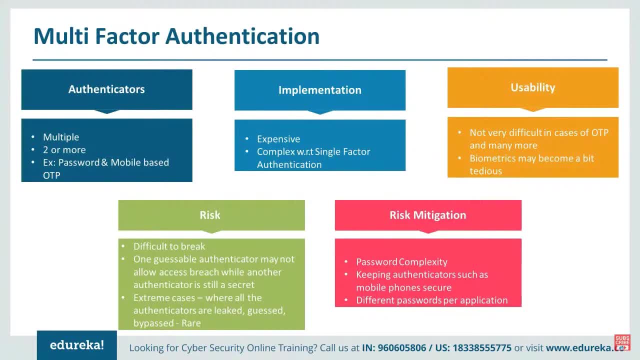 is. it is difficult to break as you have multiple factors included for authentication and also guessing of the password Can be happening. I mean guessing of the password will happen anytime in one day or two day, even maybe a week, and password could be broken. but breaking the password in combination to other factor. 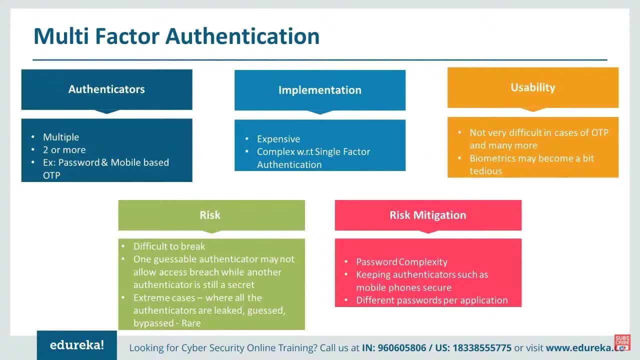 It's obviously hard. you may able to find the password at particular number of time. At least you might try it: 35 lakhs time to get a password. You succeeded receiving password, but you need to have the other factor in combination, So that would be a really tougher task for one to guess. 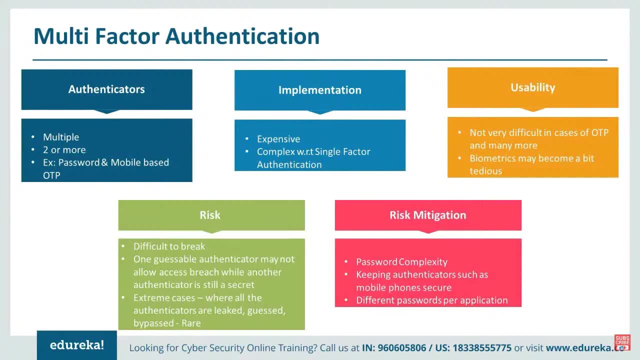 Both the factors at the time. So the same goes here. What are the things? how we mitigate the password exposure? I mean revealing the password just to make sure. have a complex password. always try to include numbers, special characters, alphabets and lowercase and uppercase, and also maybe a longer one, 20 or 30, whenever. 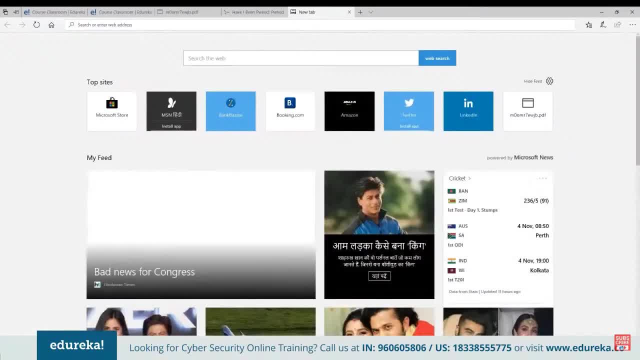 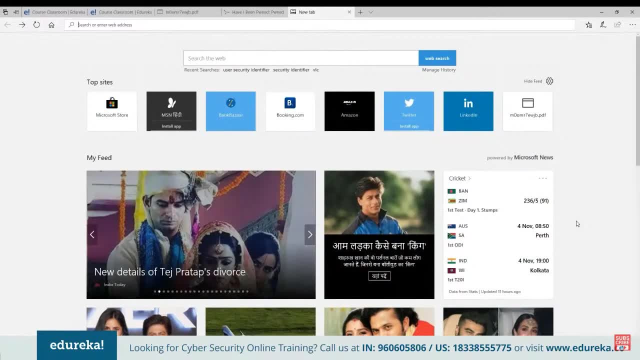 you log into a simple examples and a simple concept. I can teach it to you. previously You might be seen a yahoo emails or some other Email accounts will come up with the option of using pictures when you enter your. I'm not sure whether it's working. 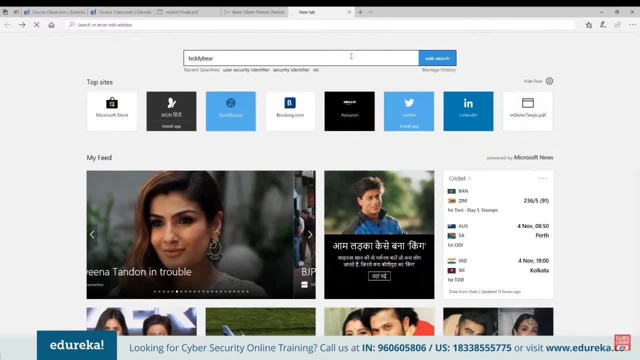 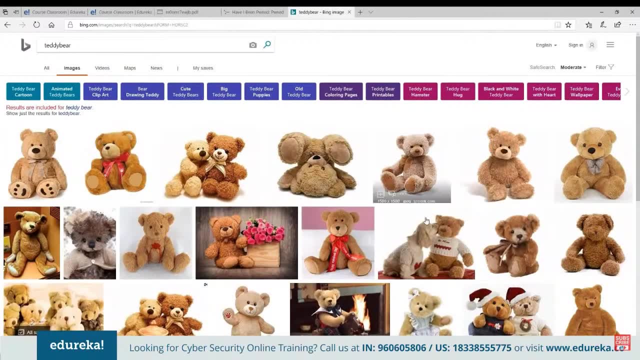 or not. Now Yahoo is having or not, So what I do is I'll be having a teddy bear. This would be my account image, Yahoo image or Facebook image or any other social media account image. What usually people will think when I have it as a profile picture. 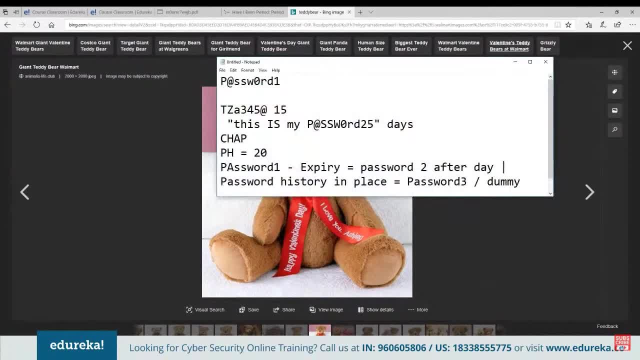 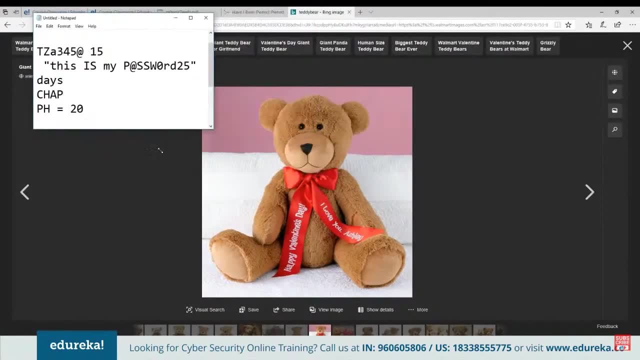 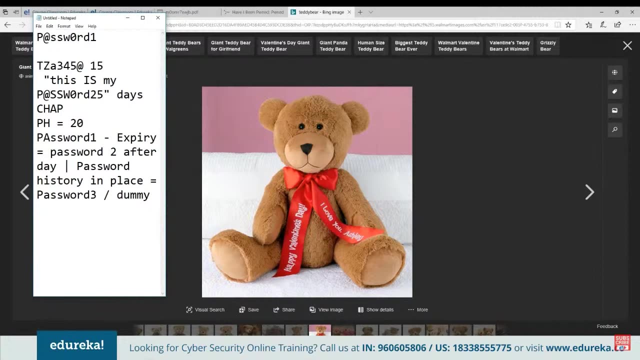 This makes no sense to other people. This is obviously just a teddy bear, what I have Used as my profile picture, And what could it really mean? So in case of using a longer password or passphrase, you might obviously have a tendency to forget it. 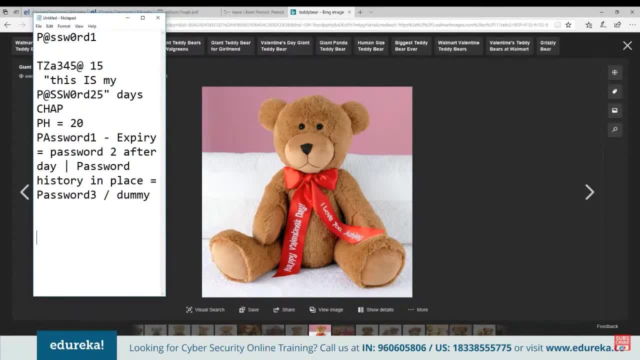 So you can generate a pattern. It's what the teddy bear is actually doing. It's sitting. so in user sitting, Teddy, with a bow, I call, or a tie, I call. So this is just a passphrase creation, So just making you to remember it, always having a flow. 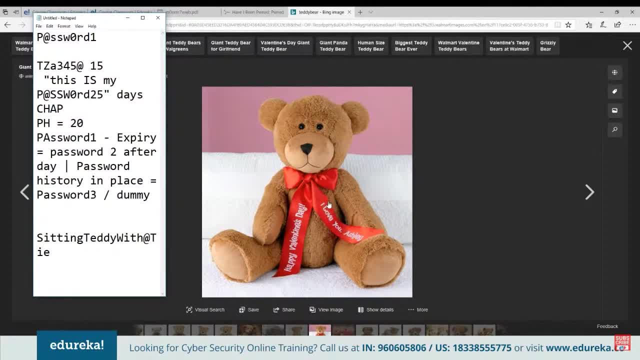 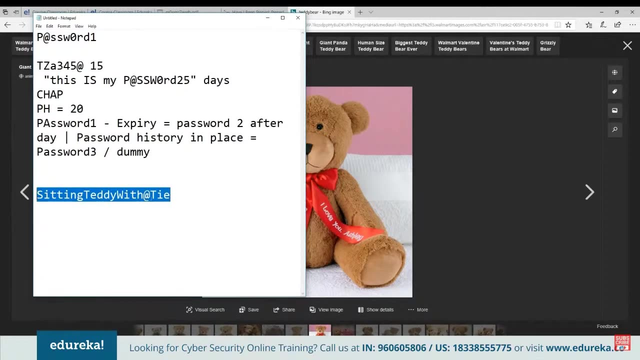 It is not goes only for the teddy bear. any image which makes you remember your password or passphrase It's obviously good. It's just a small suggestion from my end. I just used plain text. sitting teddy bear at one sitting. teddy bear with a tie instead of a I used at, so you can use combination of it. 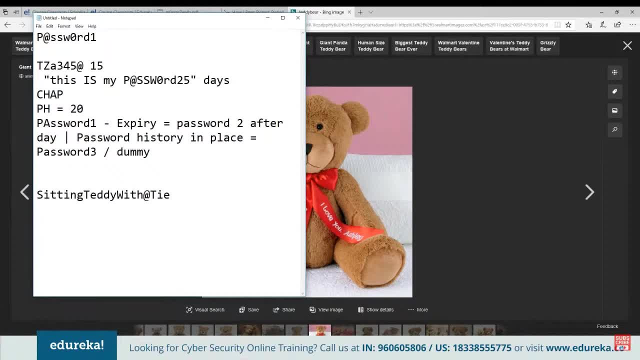 So people will have a some more tendency of changing the characters. So instead of I, so instead of yes, people will use a string character. People use string instead of why people have exclamation mark, So TT exclamation, So he can be replaced with three. likewise, whatever combination which works for you. 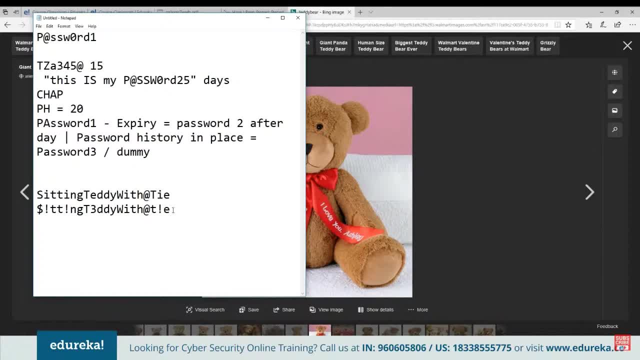 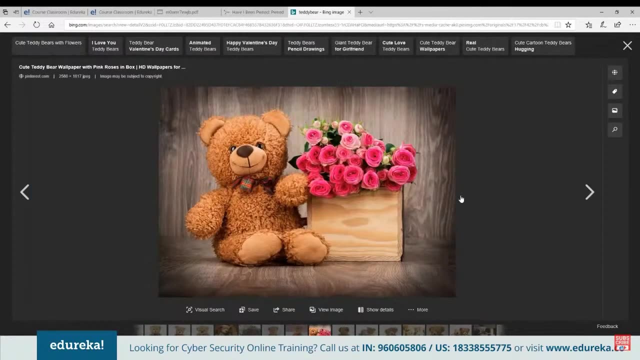 You can modify it. So this looks something weird. So for breaking this password it takes some more additional time. So it's almost 20 characters. mix it with alpha. numerically It has got 20 characters. So breaking it It will be bit complex than the regular password. 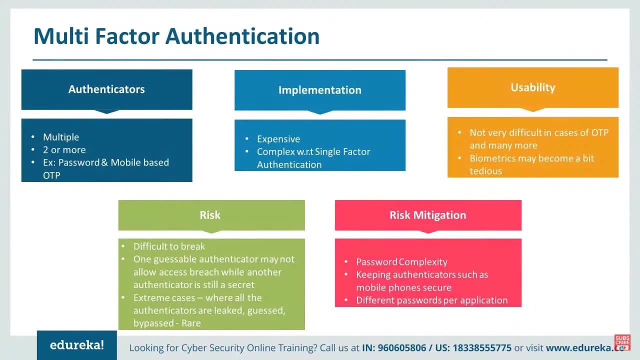 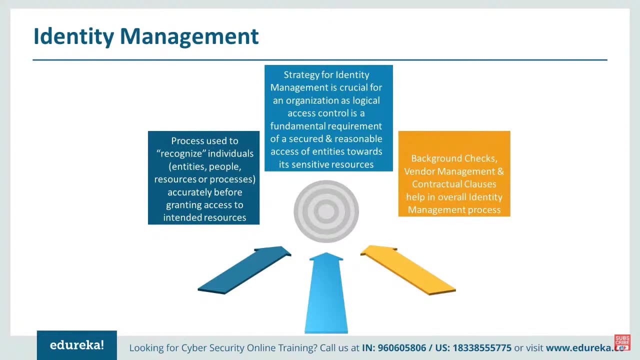 So I always make sure that you use a different application for a different password for application. usage of same password for multiple applications will obviously get other accounts to compromised when linked to. so the identity management. What is an identity? We already seen that identity. in the digital world, every object and every user or every resource will have a unique identification. 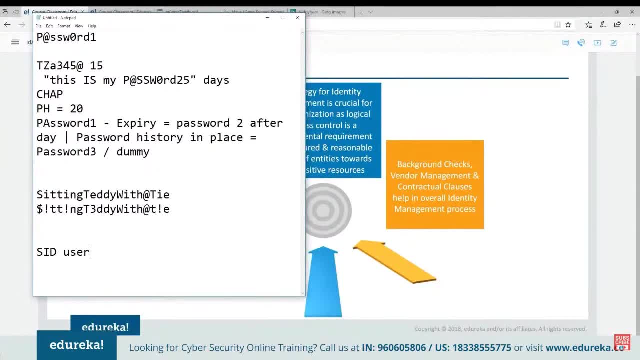 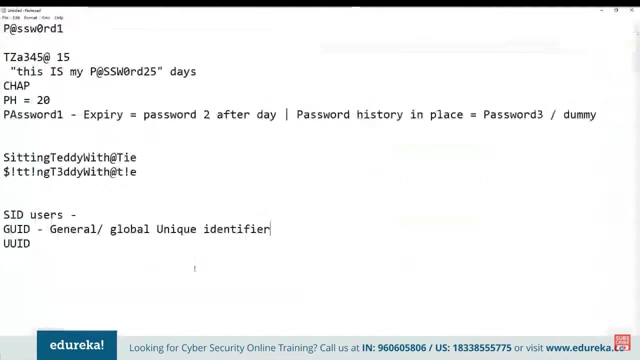 So security identifier SID is for users In Windows environment and not only Windows environment, even in Mac and Linux environment. but the unique identifier pattern will be different, So the objects in the computers are called will have a separate GUID. GUID is given for hardware. devices inside your computer is called general or global unique identifier. 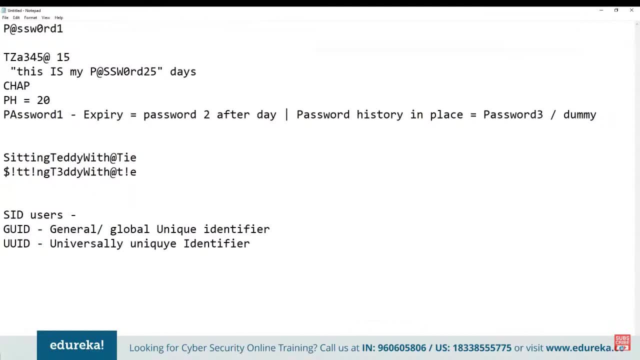 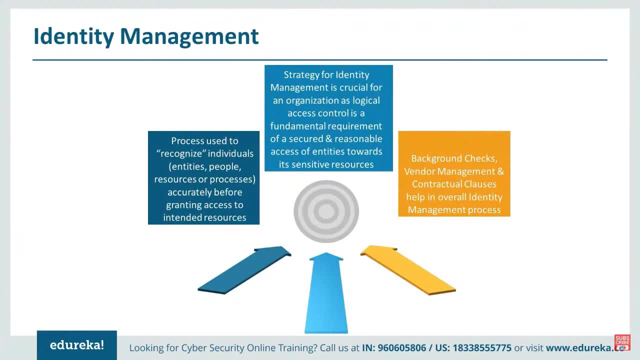 This is universally unique identifier. So SID, GUID, UID- These are the identifiers for identifying Particular object. So what this slide says is this: to just to recognize the resource, the unique identifier, It also the point in yellow I can. now, given contracts most of the time, many companies will have full-time employees and usually it's normal tendency or normal pattern in any of the organization to have at least 20 to 30% of contract employees. 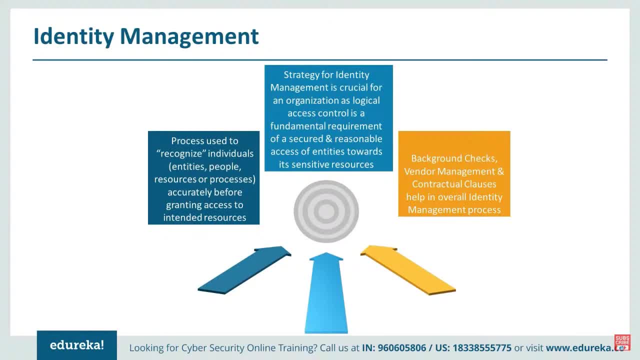 So whenever they need, they'll get them in and whenever they don't, they'll just end the contract. I mean terminating the contract just before the tenured deeds obviously common, so that will not be a big impact of the business. it happens. So it also helps us identify who are the contract employees and what are the term, when was the contract is getting and what was the contract class? 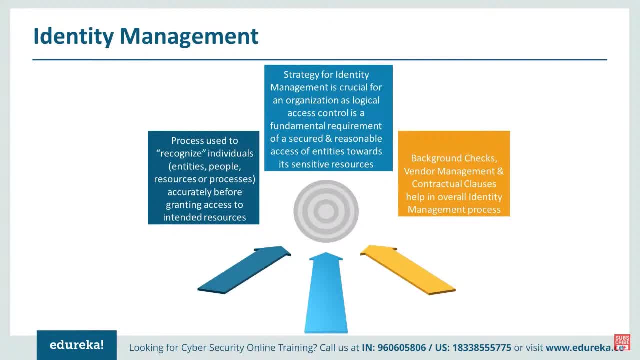 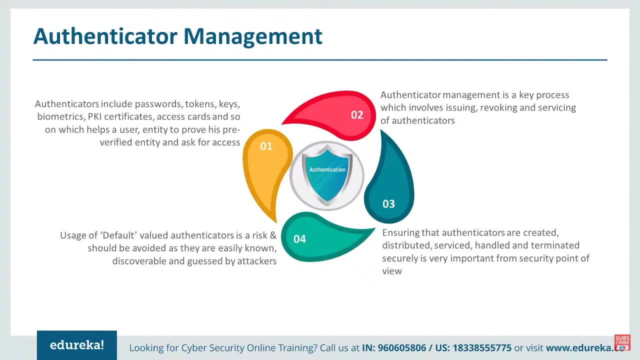 We actually use it, using it in multiple factors. also, We can identify or create a policy or procedure to authorize the user for particular object or particular access, particular resource, Particular resource in your environment. So what is an authenticator mechanism? So authenticator, authenticator is nothing but your password, your soft token or anything for authentication. 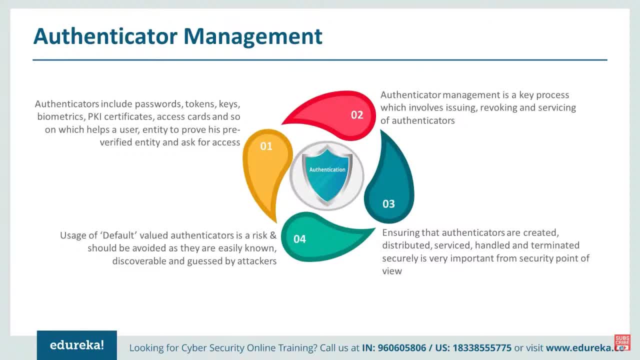 You need the authenticator. what it could be, It can be a PK, a certificate, or it can be a token, or it can be a passphrase or password, which you already know that. So, as we discussed before, for authentication the authenticator is required. for authenticator management is the important concept. what it does is 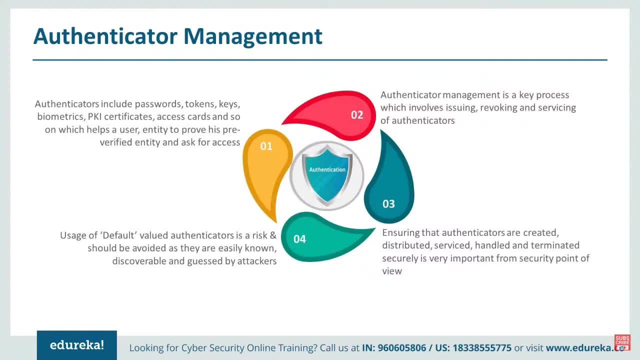 It will invoke, it will issue, it will revoke the service for the authenticators. So when a person passes in username and password is a authenticated, the authenticator management is the key object or the key service which will create the token or create the session for it. 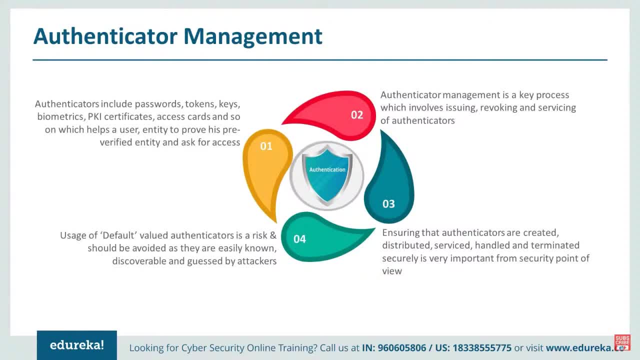 This lets when the user is created and when his expiry date is and how long a user can be accessing the environment. So the session management determination that will be created by the authenticator Management. So, as we discussed before, as the point, using the default authenticator mechanism or using the default configuration or default setting is always dangerous. 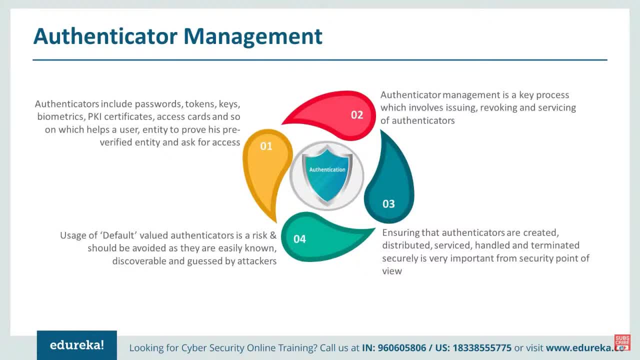 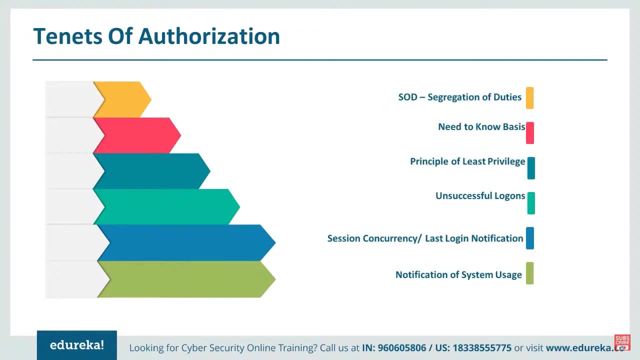 I will just change the setting or configure the services as for the business requirement. So what are the tenants of authorization? tenants are nothing, but they are the integral parts. are tenants can tenant? There is no rule for having all the tenants are placed. We have a few in place or mix it, combination in place or all in. 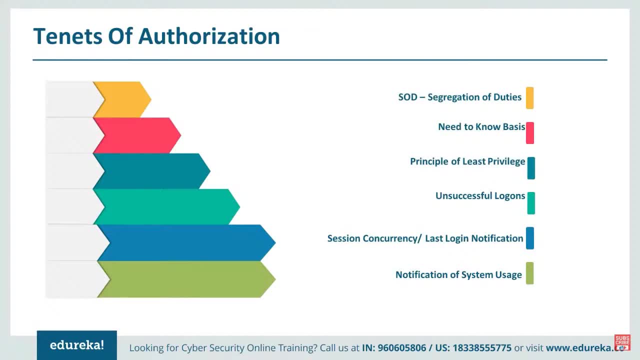 When it required to the business. So we discuss about segregation of duties because we already know that what is a segregation of duties. need to know basic. just reading out the headlines will explain. explain you the topics in the back principle of least privilege: unsuccessful logins, session concurrency. 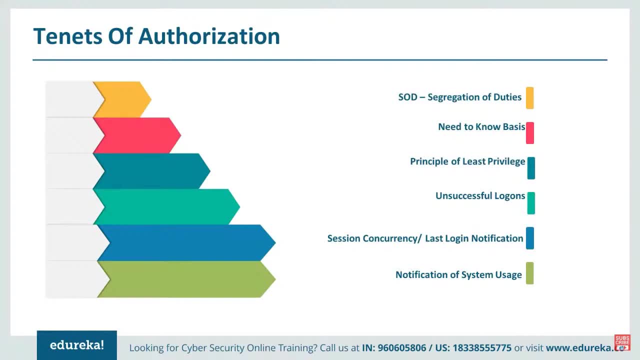 We already discussed notification of system usage. These are the different attributes, or we can also call it as a tenant of authorization. So these are the points which are considered while authorizing a particular Object. So let's see the segregation of duties. What is segregation of duties? 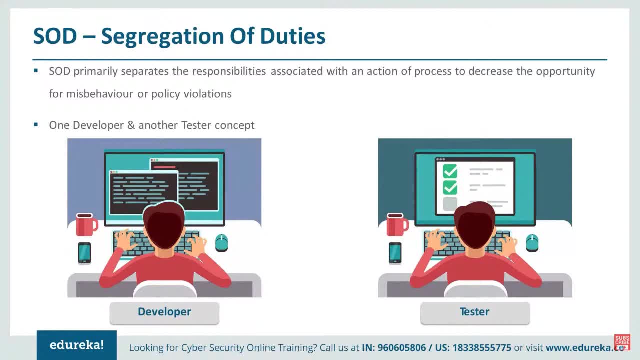 The picture below shows two different uses, what seems to be looking similar. They have a similar coffee cup, similar keyboard, mice and the monitors They even look at resembling similar. But what actually the duty separation is? the developer will have a set of access, the tester will have a set of access. the tools and the files which was accessible by the tester cannot be accessed by the developer. 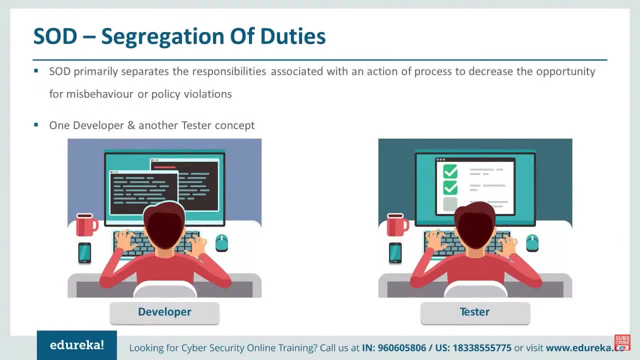 The tester will have a set of access be accessed by the developer, and it's vice versa. so these people, they both on the same environment, they both on the same network, they both work on the same enterprise, but the access and the privilege will differ from user to user. this is segregation of duties. even if it's a system administrator, he 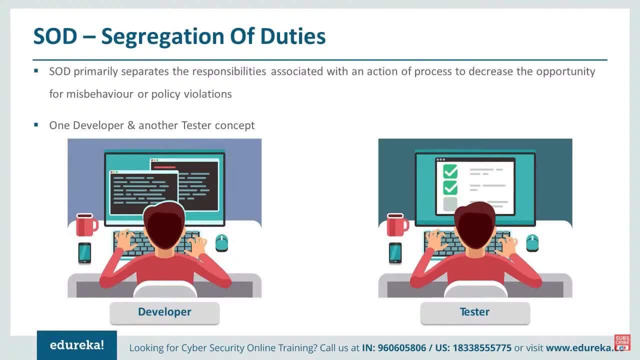 will not have the access to network administration. he may be a system administrator or he may be a network administrator. he will not access to the security operations. so wherever a user needs access, only then, then and there the access is provided, and that to the we'll be saying what are. 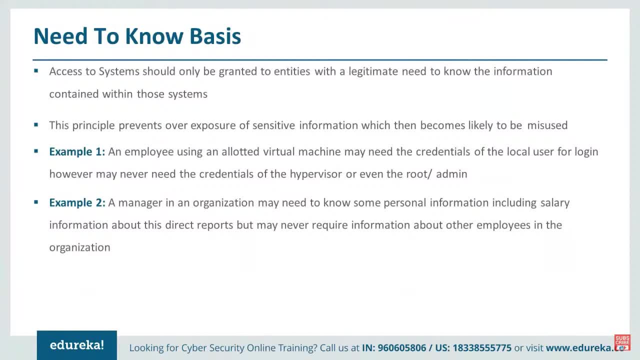 the guidelines to be considering before authorizing a particular object. and this is one of the other concept: need to know basic. i mean need to know basic italy. it is just like saying this is the minimal requirement for a particular person to carry out his everyday activity. so when a user 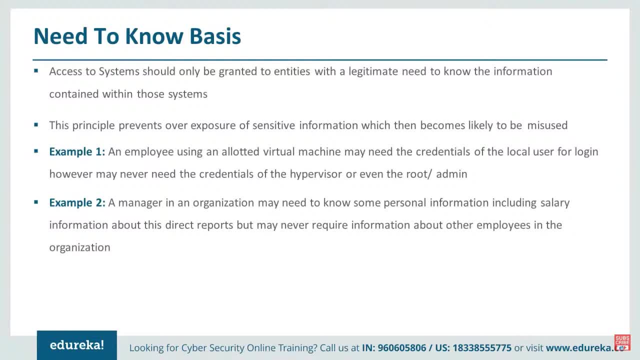 needs access for some other thing, obviously he'll be given access. if it's a regular employee or a filter employee or a third-party contract employee. the basic information, or very least acts, will be provided to him based on his role or as per the contract. so what is the example here? for example, 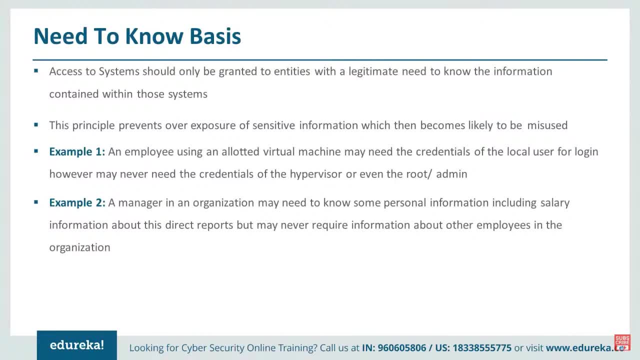 an employee using an allotted virtual machine may need the credential of the local user for logging into the computer. okay, when a user gets access to log into the local virtual machine, he'll be getting a standard user account, but he will not be provided access to the hypervisor or even to. 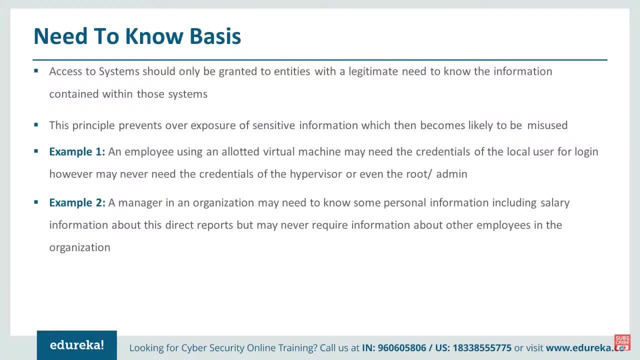 the root access or he would not have the domain access to the domain, access to the domain, access to the domain administrator, even the system administrator access. he'll be provided with the basic user access. and the second example: the user, for example a manager, needs to know the salary of his employees or his subordinates. he might be provided access to view the salaries. 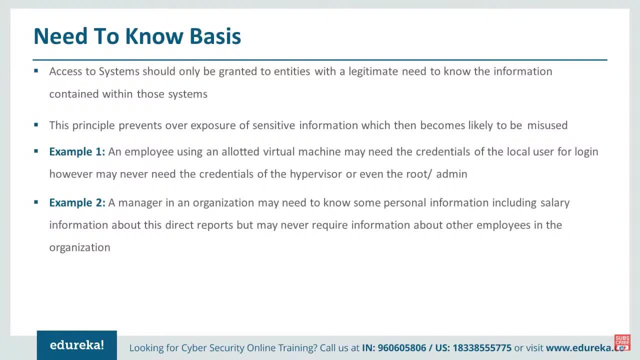 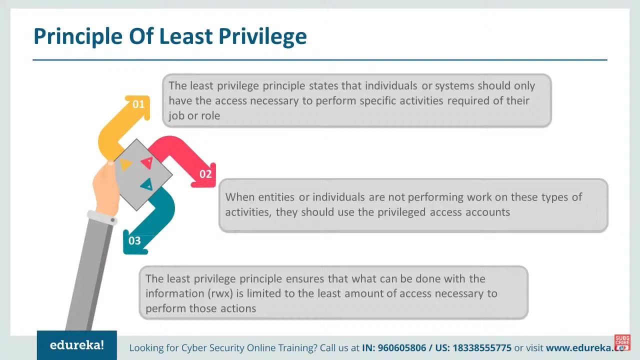 and how much is the package and how much he takes home, but he would not be having access to the other team members. these are two examples of having the need to know the basics. so also the second example is the principle of least privilege, principle of release privilege in the previous 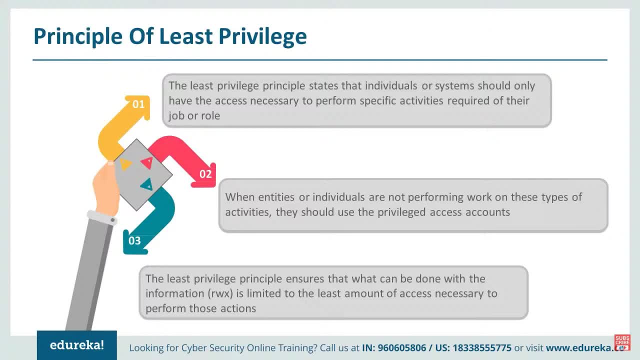 slide we seen the least access to know the information. i mean like just a read access. he can only view the information and or he can just know the information about it. the same thing goes here is the privilege access. what are the actions he can perform, what are the ways he can? 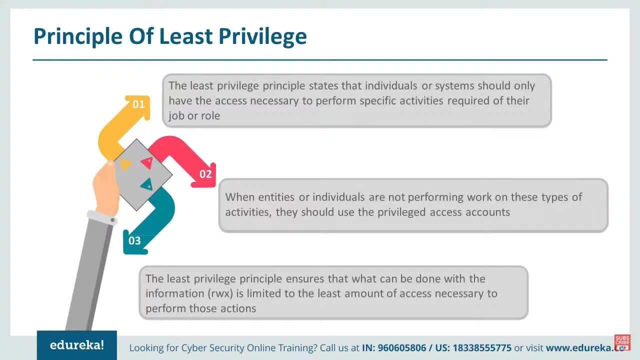 be controlled in the environment, whether he can able to write a for write to a file or read to a file. modifying the file, renaming the file- what are the things? can be assigned to this member the same set of privilege as we see on the first slide. the tester will have some set of privileges. 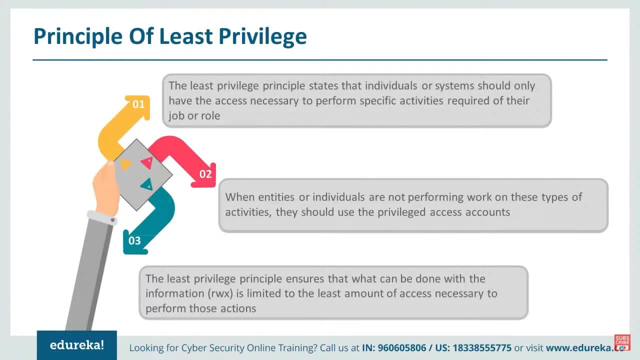 and the developer will have some set of some set of privileges, but both will have the certain level of privilege only for the task which they are intended to. if they need to run visual studio for programming a developer, he can run it that too, as a standard user, not as an administrator. 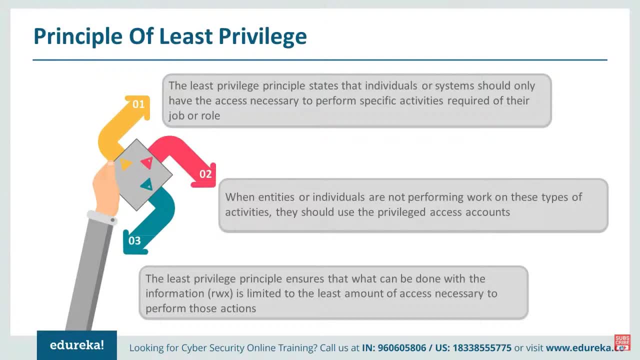 or with an elevated privilege. so this is the concept of providing least privilege, or providing only the limited access for the user to continue or carry out the everyday task. if there is any superficial access need to be provided, that can be provided based on the exception, and that too. 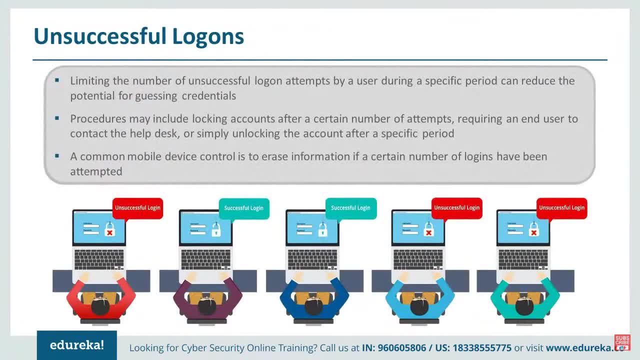 time-based and that would be reworked periodically. so this is also a factor. unsuccessful logins: what we call unsuccessful logins when a user tries to log in for multiple times and he's not able to log in properly, but actually he's a trusted user, he does not have any intention to break into the computer or his does not have any. 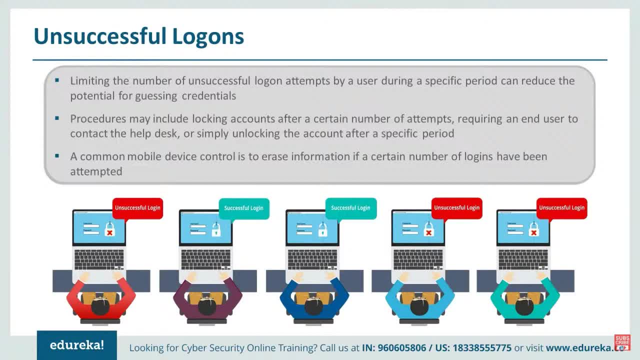 intention to log into other users account. there may be multiple factors of getting failures in the login. we also take it as a consideration of number of unsuccessful attempts. what are the ways we can mitigate? we'll set account lock down when unsexual login for three or four times the user. 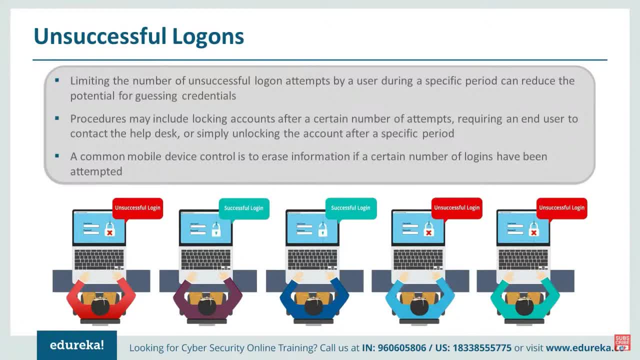 will not be able to log in again for next 30 minutes or for next 24 hours or continuously until the user calls on to the customer care. I mean the user calls on to the customer care service desk or he logs into the self-service portal to unlock his account session concurrency. 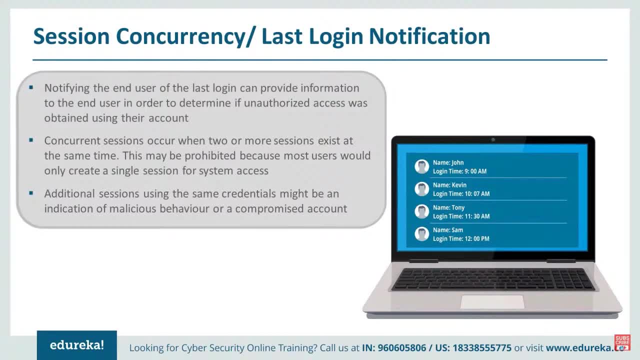 we already seen that the session concurrency. whenever a user authenticates and gets authorized to enter into the network, he, every login, will have a certain session created and every session will have a expiry, as we already be aware about it. so when a user tries to log in from multiple 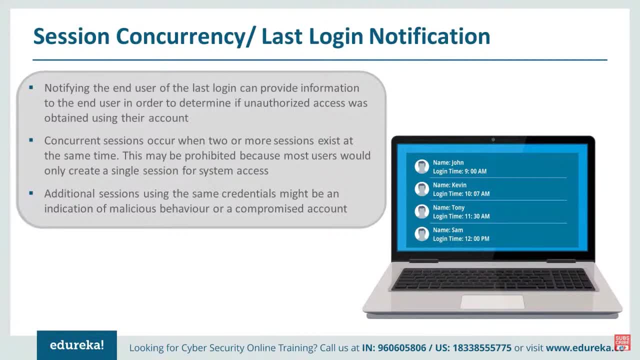 computers, we can eliminate whether concurrent login is enabled or not. if he really- uh, I mean managerial user or executive level user, if he needs to work both on his workstation and laptop, we can provide multiple sessions and that too not required. but if, in special exception, we can provide concurrent login or we can just pass on the previous login to the 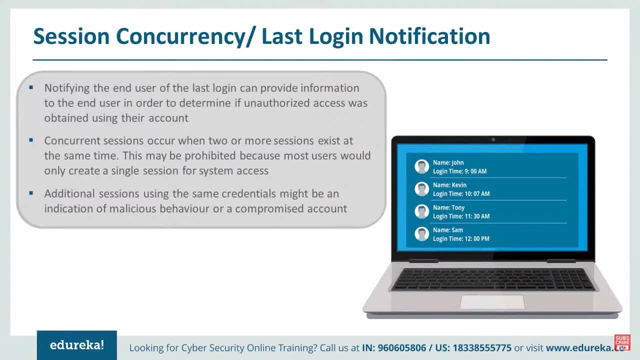 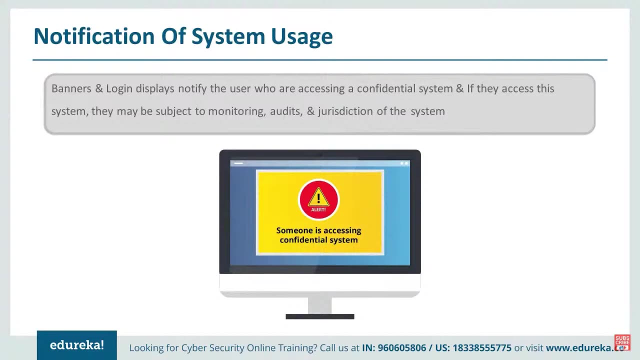 current computer which he tries to log in or completely terminate both the sessions. it's completely up to the management who to decide what kind of authorization procedure or policy we need to include in it. notification of system usage. this is more common whenever you try logging into the corporate environment. 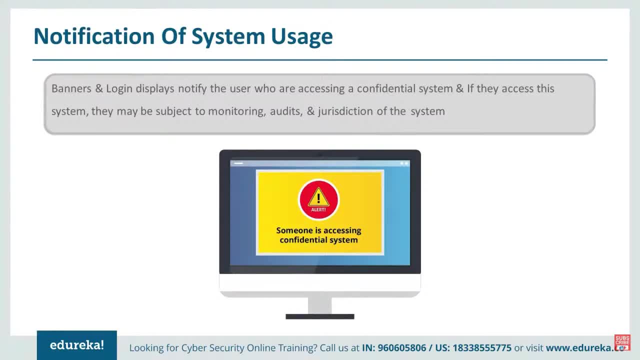 it may be a virtual machine or a laptop, or it's a desktop. even before key typing in your username and password, there will be a system message that shows this property belongs to particular organization and usage of particular resource or authorized materials. it's only for the business. 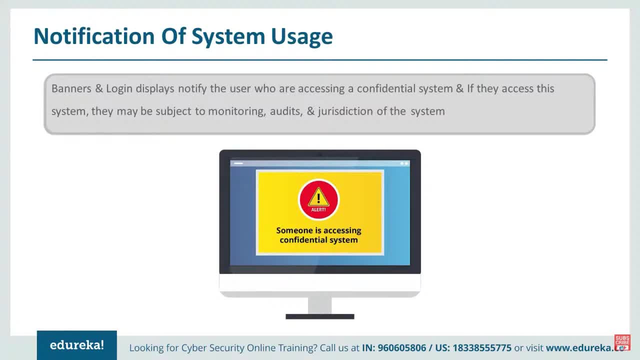 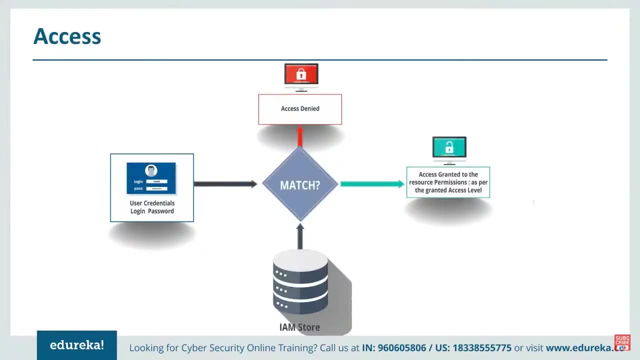 purpose and it's just like NDA, non-disclosure agreement kind, or if it's a statement, legal, which prescribes the legal term and conditions of usage of the particular resource. this is common on once you access the environment, regulation of access. this is a simple diagram will explains so what happens in the left when a 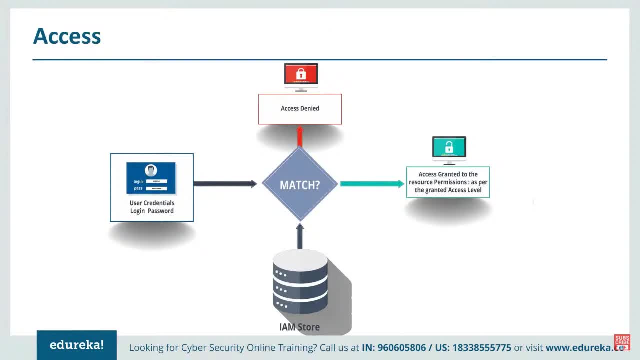 user uses password, the username it matches to the IAM store. IAM store is also has the list of usernames and hundred percent of the IAM stores will have the password hashes instead of passwords. so even the password hash will be encrypted and that will be sent to the IAM store in a 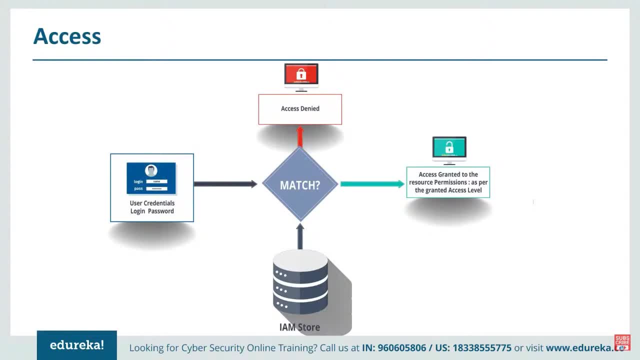 encrypted banner. so no more plain text in even intranet or anywhere. so the encrypted hash will be matched along with the existing value and so that the person will be verified whether he's he got the privilege or not. if he got, yes, he'll be granted access. he'll be sent to the authorization. 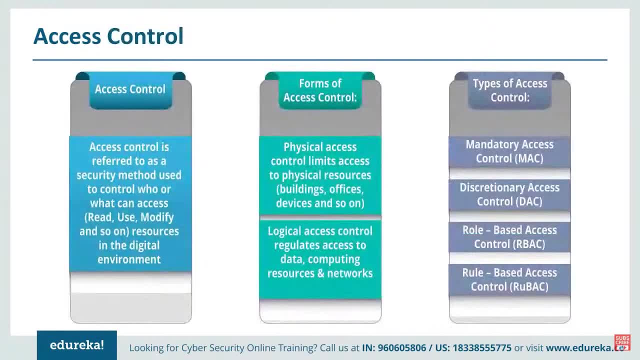 phase. if it's not, he'll be just sending it denied. what is an access control? the access control is nothing but restricting or providing access to particular reserves or an object. what are the forms or access control? it may be physical access control and both logical access control, whatever. 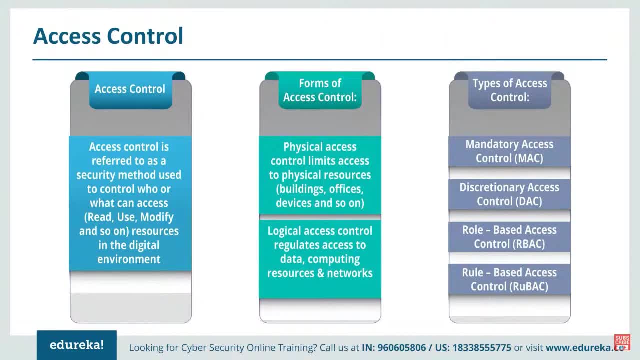 we provide rights or limitations or restriction inside the computer. it's logical. and what's interacts to the physical world, it's physical. you might be coming across the server rooms which are locked separately. those needs, the separate access cards, separate password management, separate access restrictions. so those are called physical, not even just before entering into your corporate building. 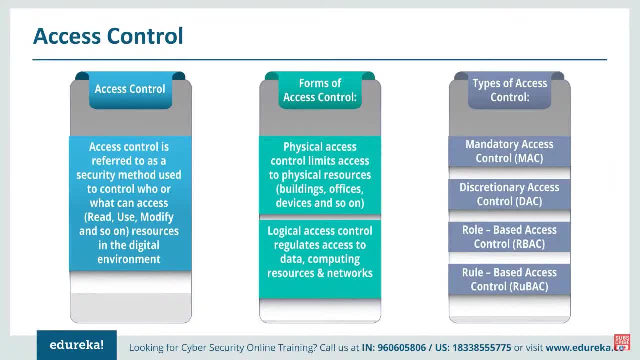 you need to have your id card to the same amount of access card just to get into the system. so what are the types of access control? so there are four different access control there. to be precise, it's five. fifth one is missing here i'll be explaining. that is uh. first one is mandatory access control. 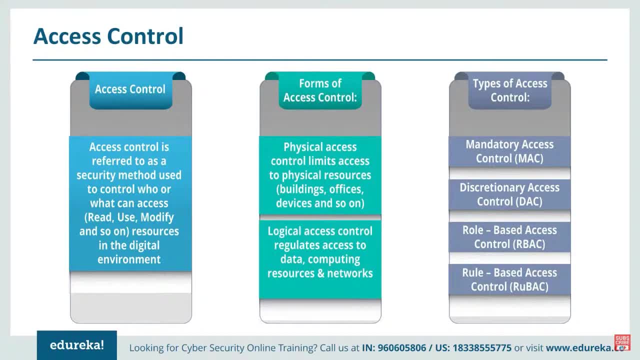 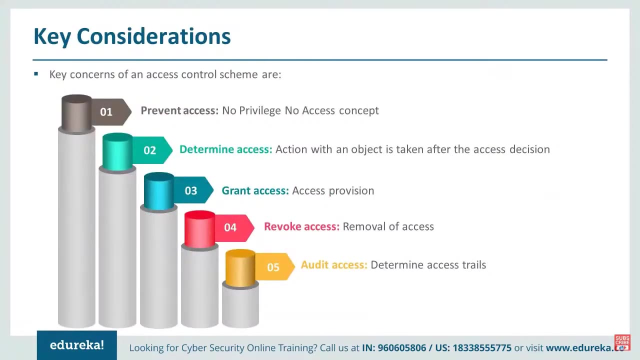 that is mac, discretionary access control, that is dac, role based access control and rule based access control. along with it we have one more access control called attribute based access control. we'll be discussing further on it. key consideration of providing an access. what are the things we can consider? so the initial thing: 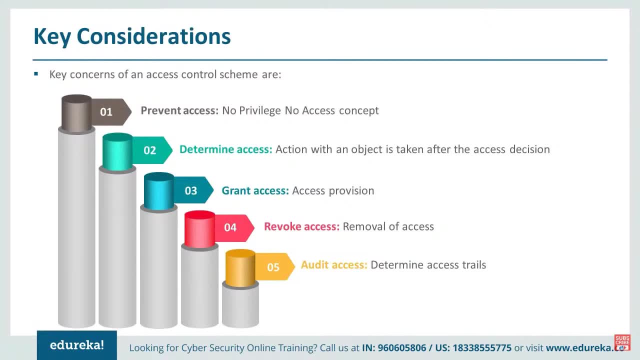 is to not to provide access to no one. no privilege, no access concept. so when a user account is created or it can authenticate, the authorization, first phase is no privilege, no access. it can also add in a layer by layer we can create the access. so after blocking it, we'll add certain objects to it. 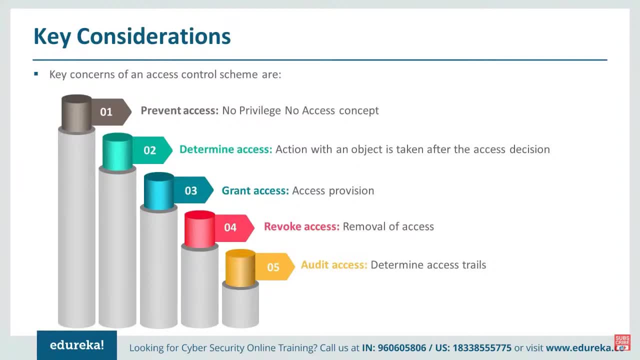 and only the certain objects can be accessed by it. so after that we can. if there is any special request or special exceptions, we can provide access and also after a particular time of expiry or particular time of approval we can revoke the access and periodically we need to audit and determine whether this access is necessary for. 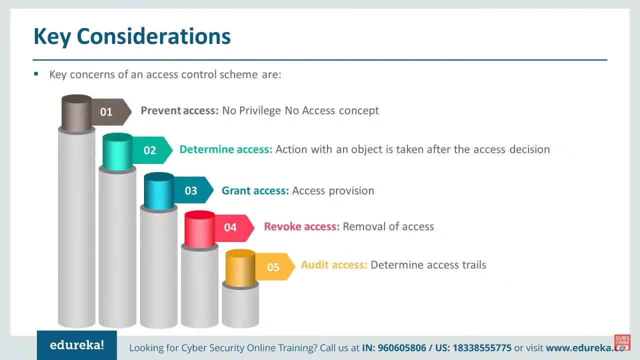 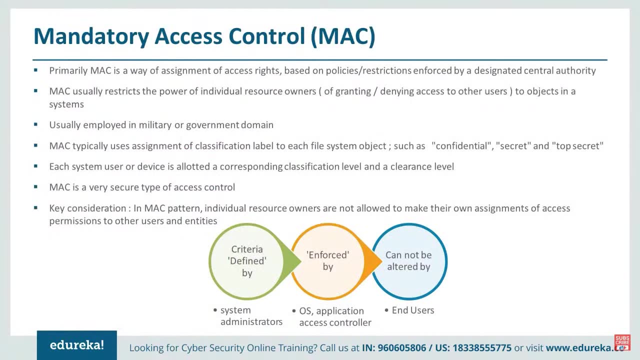 this role or for this user. these are the considerations we need to have in mind when assigning or allotting access to a particular user or an object. so the mandatory access control it's global. i mean what i meant. global it's mean the complete infrastructure, the complete enterprise. 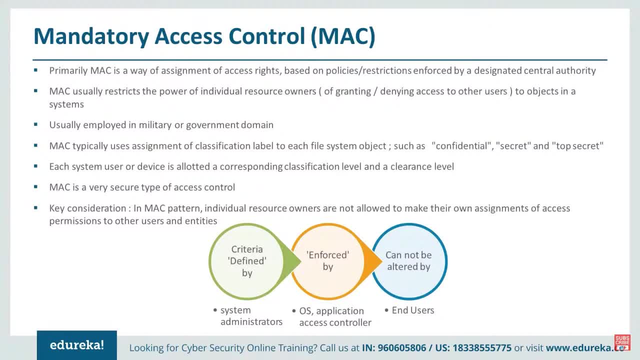 usually this will be happening on military or government agencies. even nowadays, top corporates will have the same technology. i'm saying same access control. the mandatory access control is designed or created in global wide and this will be enforced by the operating system, the application access control and this decision tree or the access rights or administration rights or whatever. 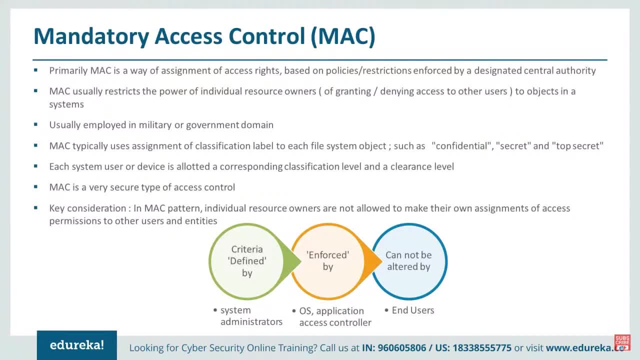 privilege will be given that cannot be changed by end user or even anyone. so what is the purpose, or what is the main reason of having the mandatory access control? in military or in government agencies or top enterprises? the mandatory access control will have the ability to classify the files. in the previous session we 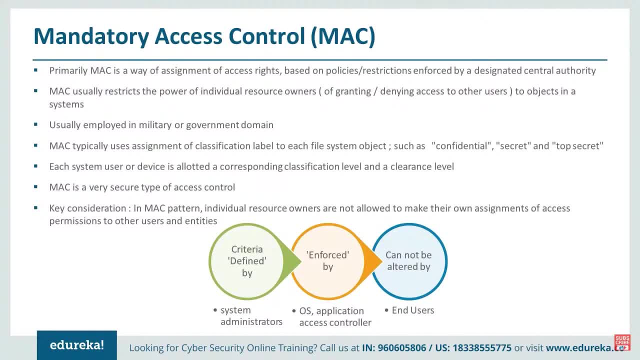 seen about data classification, how the data to be confidential or top secret, or to be public or general. when we have mac in the place, we have the ability to assign data classification for any object and every object. so based on the objects data classification we can allot rules. so even for a single file, resumedoc, that can be classified as a top secret. 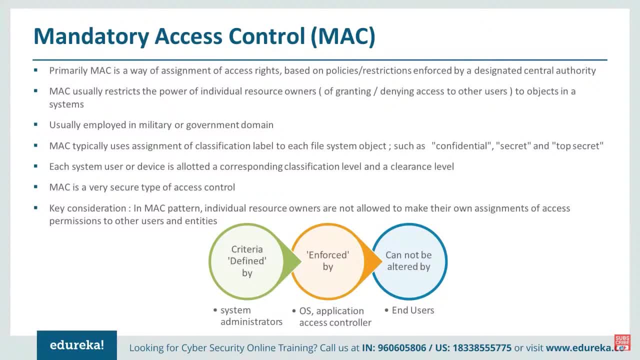 so those simple file can be available on any file system it may be for available on a file store, any shared location. any people can see that there is a file but nobody will be able to access the file. so this kind of mandatory access control is a very important part of the data classification. 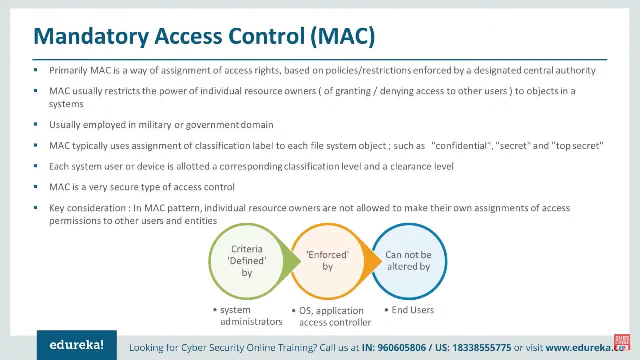 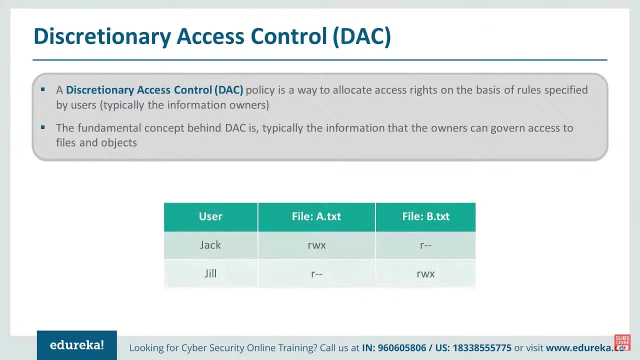 highly important because we can classify any object, not only the data object, user object, system object, resource object. any object in the digital will be controlled and classified and we can create customized rule for it. discretionary access control: this is also a type of access control where a user provides access to other objects. he will be having the ability to change or alter the. 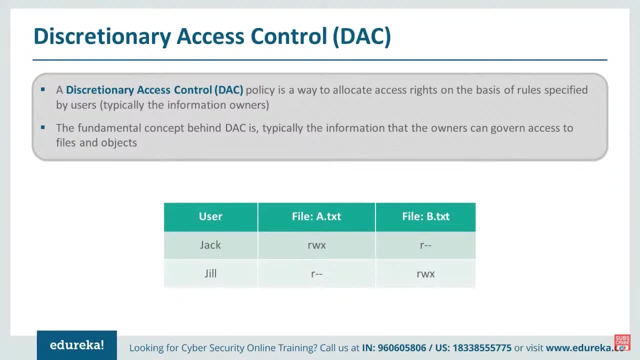 attributes or alter the access controls. for example the user a on the user a on the user a on the user a. in the file a text he got the read, write and execute access. so but for the file B he got only the redirect ses. likewise the user Jill will have only the read access on the file aid or text. 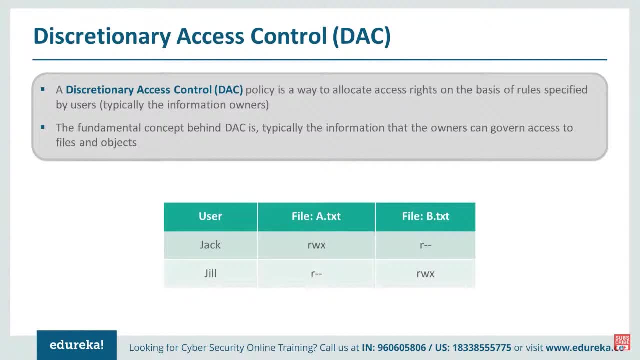 but he, you have got the full access. he can write or read an exit. so this is just a simple example. likewise, the object can be altered. here the user is. the object has been provided access role based can be altered: here the user was the object has been provided access role based. 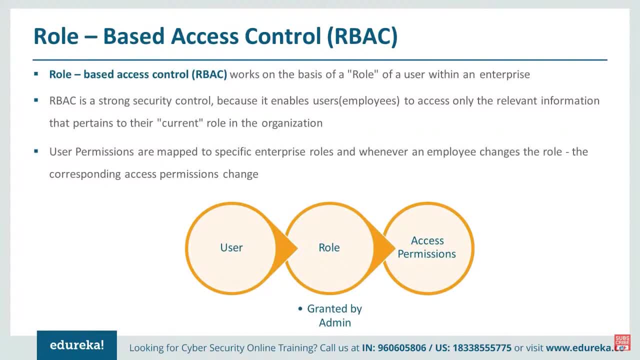 access control is most common role. when an organization is created, hierarchy is decided and based on the hierarchy every designation will have a particular set of roles. role and particular role needs particular privilege or particular access to for a particular object in the computer environment. so this will be: 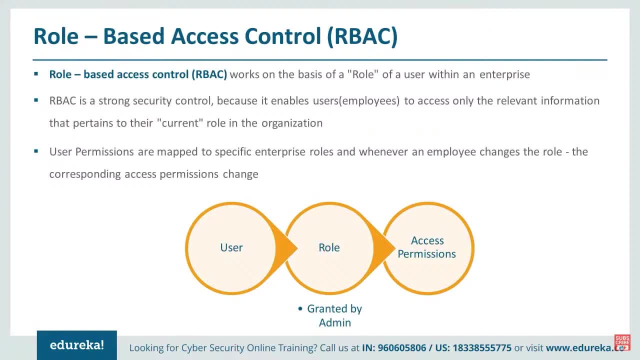 based on the role of an employee. for example, I'll be creating a finance group, the object under the finance group, I can assign the rights. the finance group can access folders to finance. the finance group can access to financial applications and they can visit particular website as particular banking. 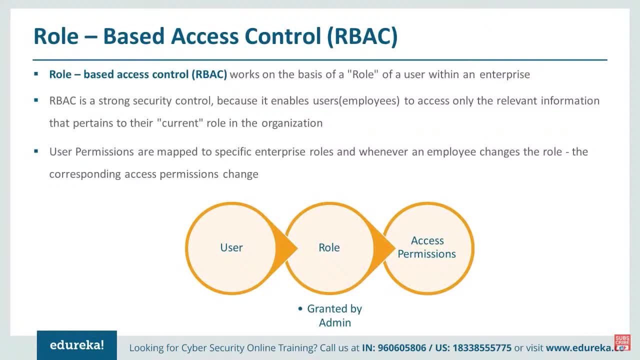 websites or particular domains internally to log in to the financially. so these are some of the example of access. I'll be ascending to the finance group when a new person comes in, when a new employee comes in or when you lean newly depleted to the finance team, we will be assigning the person to the. 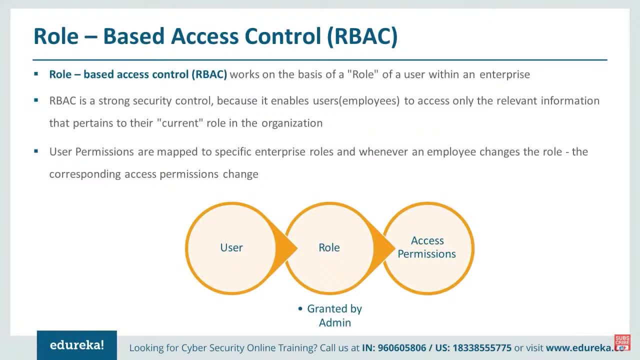 finance group which is particularly specific, created for the role finance. so when we add to add them to the particular group, obviously he will be having the access of financial software's, financial application and financial data. so what happens when the person is not applicable and for finance and he'll be moved to the HR, will be removing him from the HR. 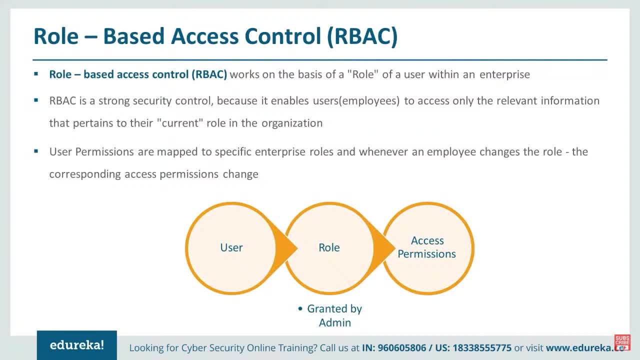 group- I mean finance group- and adding it to the HR group. so the group changes, the role changes as per the access he'll be having the access for HR folders, HR applications and HR data. so, like was for every role, we'll be having the segregation- I mean duties- and the access segregated. that will be provided only. 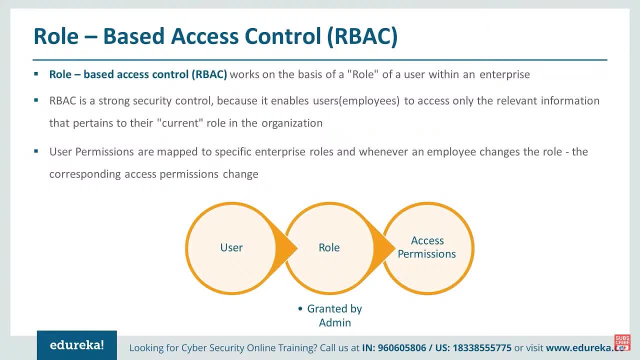 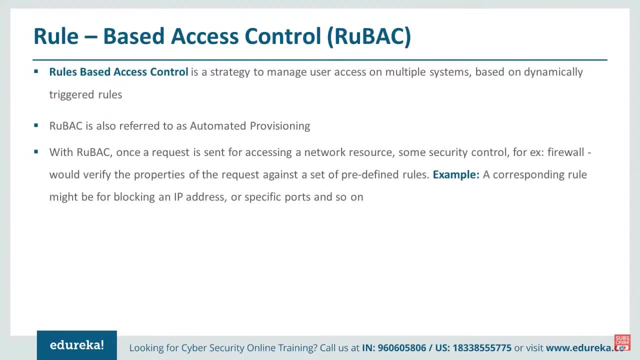 based on the role he plays in the environment. I mean enterprise. the role based access control is not as close as the role based access control. the rules can be customized. it can be customized or specific application level or specific object level. this rule where I can combine, for example, I was of when a 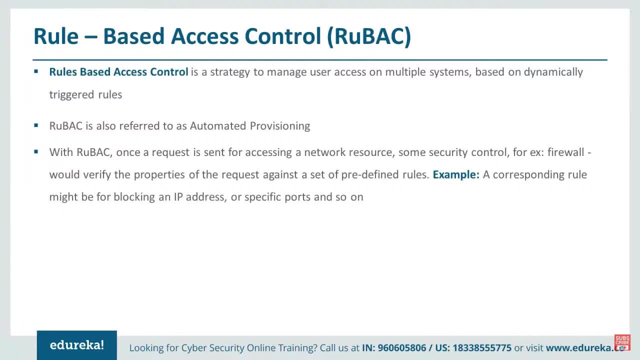 user needs to log in from the finance group. I can log in from the finance group. I am a remote computer. he needs to access a VPN connection. so the VPN connection needs particular set of IP range. so only the power we configure a rule, only the certain range of our piece can enter into the corporate premise. so 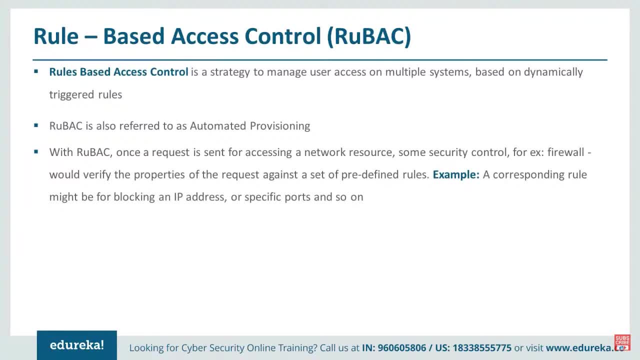 we can block it. this is one kind of rule: without ID card the employee will not be permitted inside. that can be a rule after business, our suppose business as the user account should be automatically logged off. if it's fine in the evening, the computer will give a notification and it. 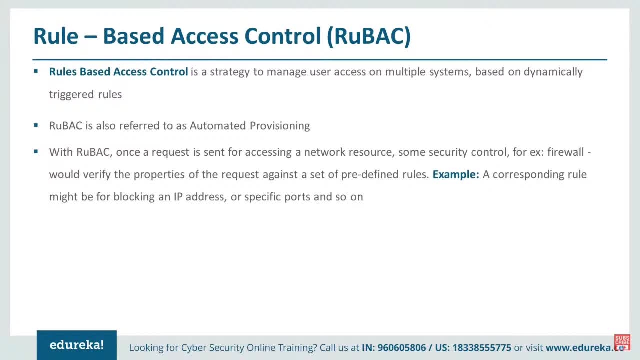 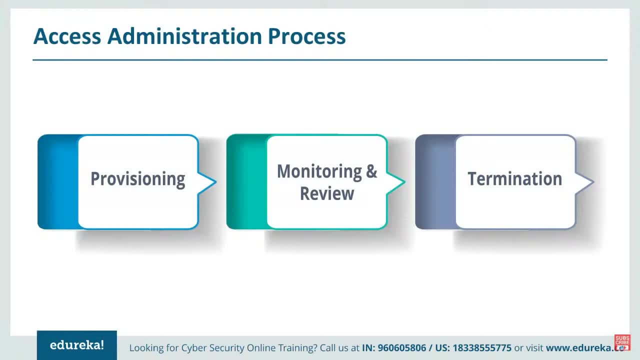 a automatically log off. this is one of the rule, so the rules will be customized and that can be assigned to any object as per the requirement. so the access administration has three subcategories. provisioning this is allowing or creating, initiating account access- the important term as like the other objects. 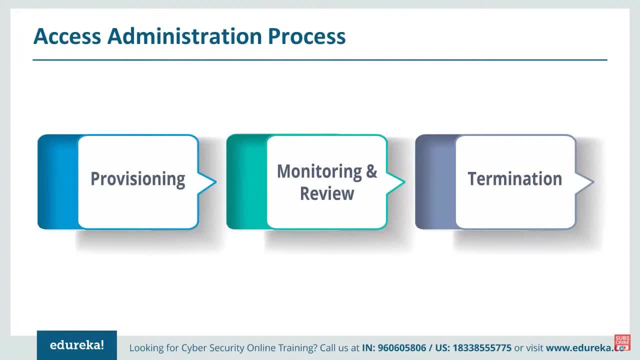 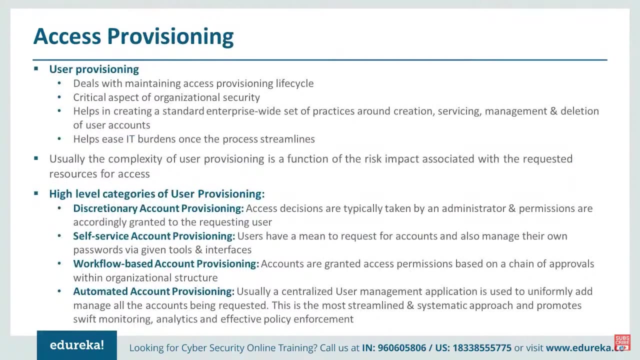 it's monitoring and continuous review of the activities and the changes and the effect of the particular access. and the third step is terminating when the access is no longer available, when the object is no longer available, how the termination will be taken place. so what are the topics, what are the things we? 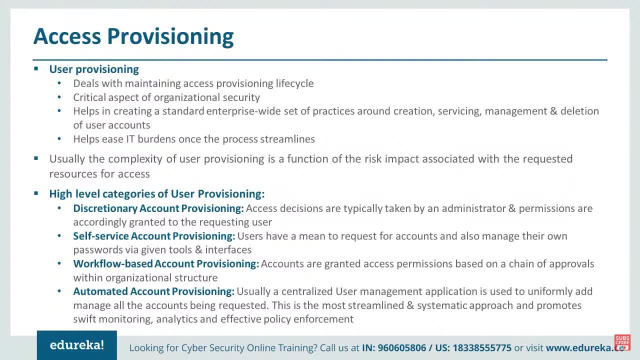 consider when we provide an access. actually, this deals with how long the access needs to be in the system or how often it has to be used in it. we need to think about the organization's security consideration before providing the access. so the provisioning of the access is. 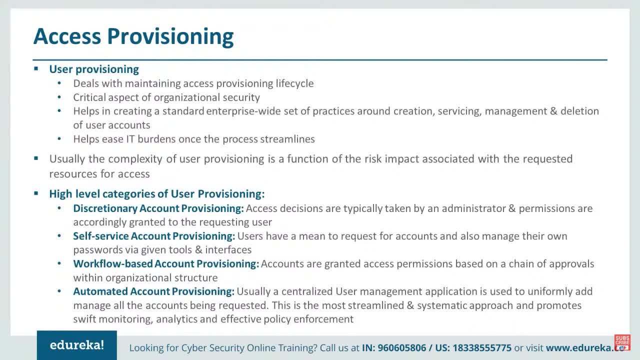 not provided by the system or the organization. the provisioning of access: when it done during the creation of access or creation of the object, it will be easy for IT team to segregate or streamline the processes. so also the high-level categories of user provisioning. one is the discretionary. 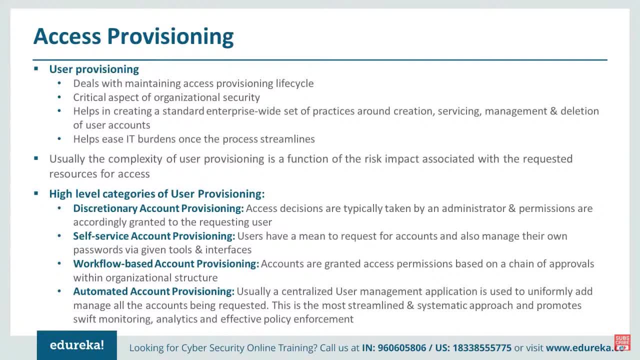 account provisioning. this is actually done by the system administrator. those are the people who will be deciding who needs to be given what access: self service account provisioning. that is a way. the nisself name explanation. the user can raise a request and automatically, based on his previous 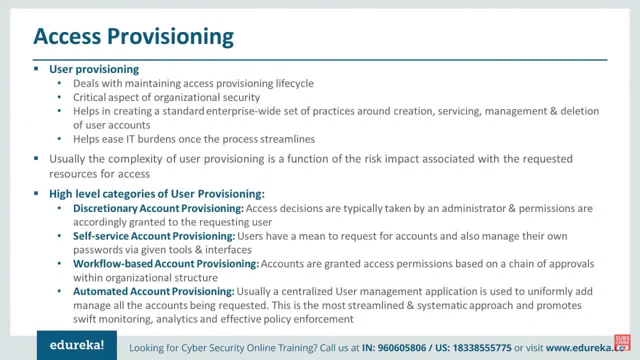 existing criteria, existing configuration. the software decides whether to provide the access or not. a temporary access. he can obviously get it so workflow based access to account provisioning. a simple example of self-service account provisioning is creating your own guest Wi-Fi. you can log into the page. I need a. 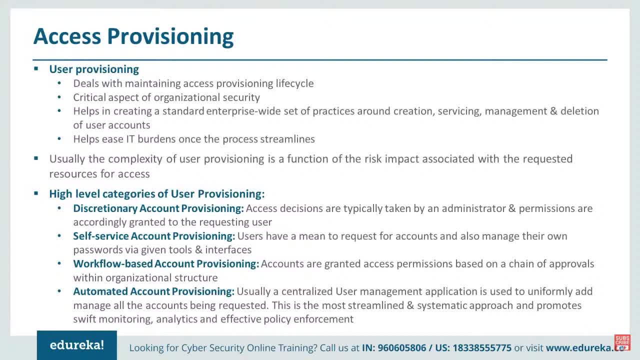 Wi-Fi account. you'll give a request in the second or less than a minute. you'll be provided with the temporary username and password for just using the guest Wi-Fi access. so workflow based account provisioning. it's not only involves on the single work role or single duty or single 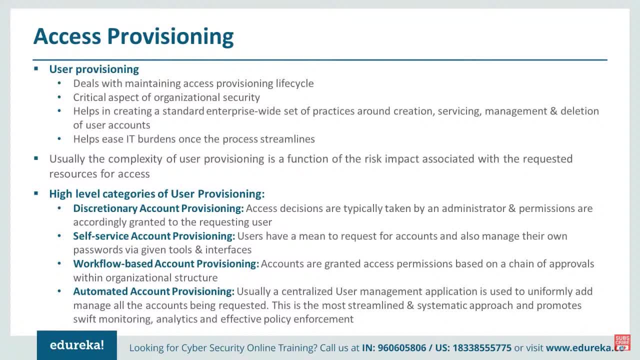 responsibility. as long as the duty or responsibility of a particular account needs to be extended or needs to be involved multiple segments, it will be added. so, for example, if a person from my IT team, he got access to the particular set of privilege and access to particular set of doors, but what happens? 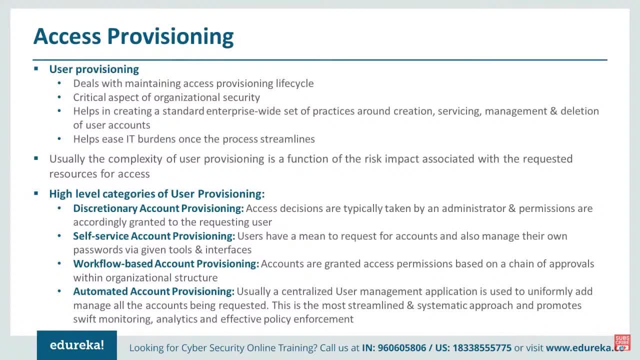 housekeeping when the business closes, obviously they need access to get into all the cabins because for cleaning or maintaining purpose. so the access restriction will not work as, like the IT or other department people, based on the areas they need to go, the access differs, and that too we can trust it. what time? 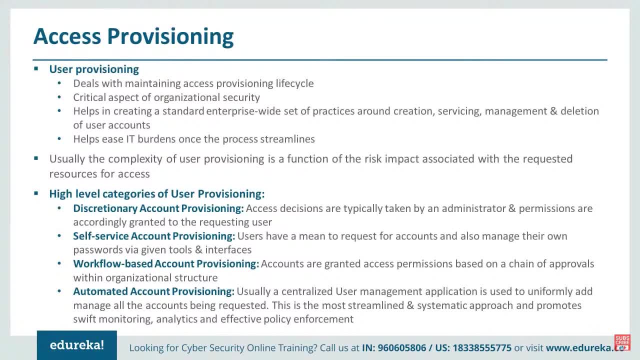 they can access it if it's available only during when the IT people are available. they can come in or beyond the business hours. they cannot access into the certain cubicles or certain room, certain meeting points, etc. automated account provisioning is a predefined stream process where the set of data or set of rules are previously. 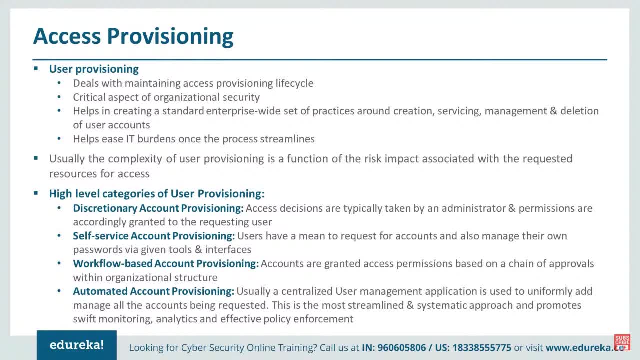 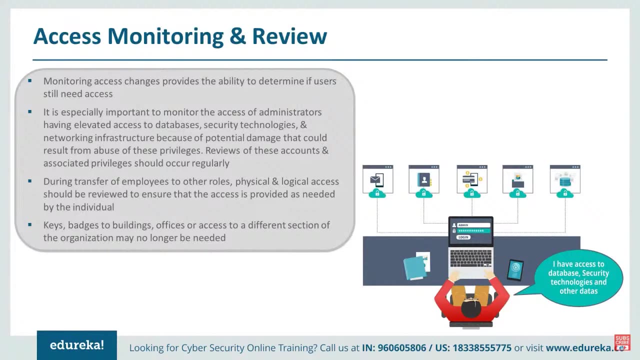 configured. those will be assigned when the new account is initiated. so most of the time the discretionary and automated account provisioning is more common in generating the account type. so the access monitoring and review. access, monitoring and review- it's not only the provisioning, the duty will not stop at. 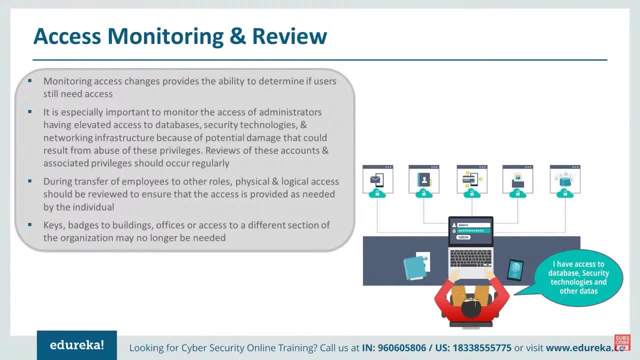 the phase of provisioning it, monitoring each and every transaction. on any transaction of the account, the service typically any access. for example, what is the regular type of behavior? what time the user actually logs into the computer? will he be on time? that can be dropped if the officer starts by 10 in the morning if the user regularly access. 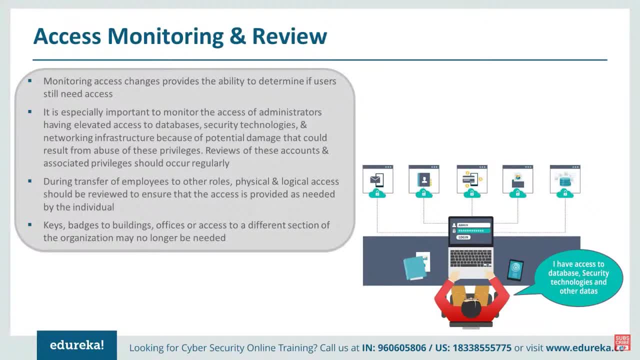 by 11 in the morning. he's obviously late or he might be for your 10 months prior to the business, as we can identify with the login patterns or easy, usually login with the same ip address or unique ip address. what is the physical location or global location he? 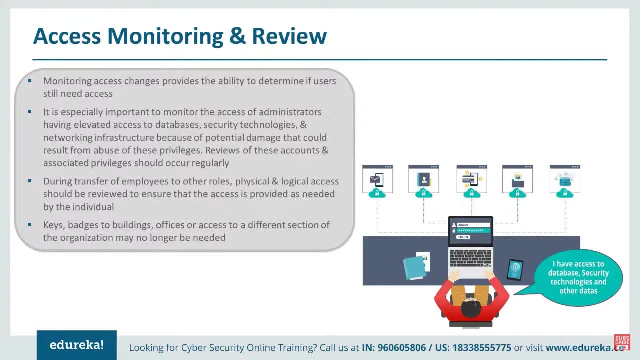 logs in from? what are the applications he access? how long he's be accessing the application? what are the files he created? what are the amount of time he invests in network? what is the total network bandwidth he consumes on a typical work day? is there any excess? i mean anomalies for 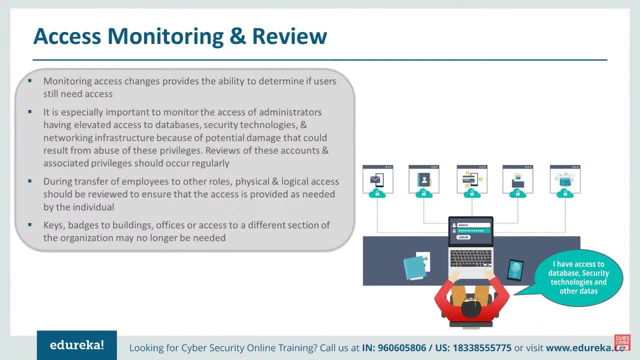 example, if he uses only 500 mb or less than a gb of data a day. in some times, if it's exceed 3g, 2 gigs, 3 gigs, there is obviously an anomaly. it means that the data is somewhere moving, maybe internal data or external data. when it crosses beyond the baseline, that should be nullity. 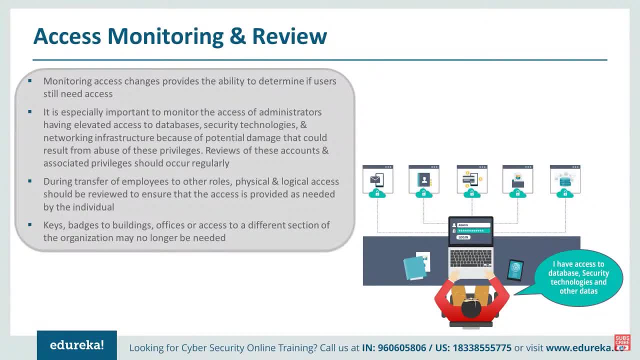 so also, like physically, we can check what are the cabins his physical card is accessed and what are the places he visits and what are the devices he connect to the carpet and one. anything and everything will be monitored. he may be trying to log in from his personal computer on the user. account, which is probably not a good one, and then he will be trying to log in from the computer and the user account, which is probably not a good one, and then he will be trying to log in from provided by the corporate network. I mean company. 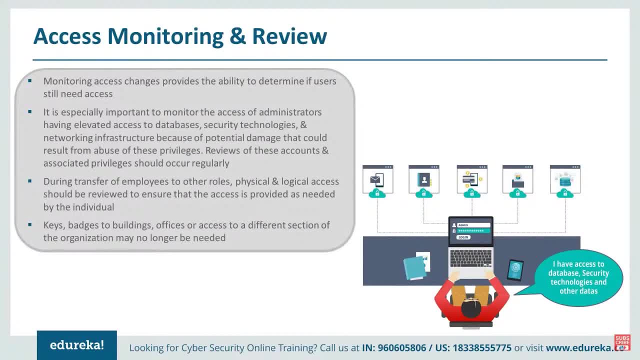 Those are the examples. Any and every activity and every transaction will be monitored and reviewed. This is a continuous process. And also the fourth point: when a user is transferred or moved to, physically or logically inside a subcategory, the appropriate roles and rights will be assigned to him. 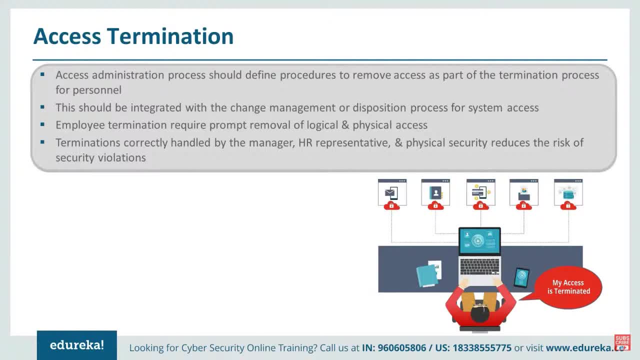 So what is the access termination When an employee leaves wantonly, we'll be conducting a survey- I mean proper exit survey- why he needs to leave the company and what are the access was provided to him. Was the IT assets provided to him collected back? 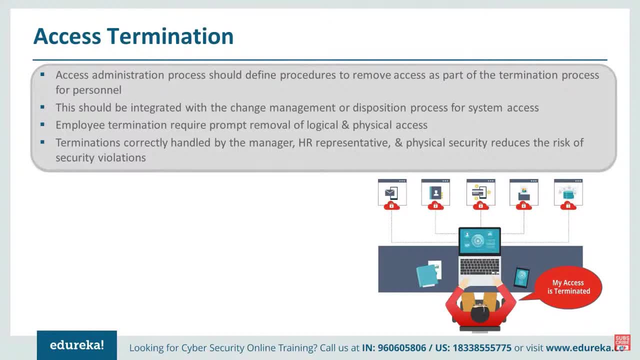 Was the assets damaged? Was the data tampered? Those things to be taken into consideration And if the employee was terminated for some cause, so before termination reason, we'll be investigating further on the recent activities. What are the activities he does? 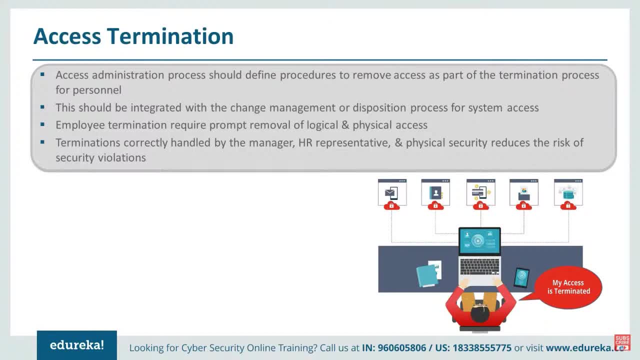 What happened and what made the company's success. So, before terminating him, the background check and the cost analysis that will be happening. And one more point I need to notify is when an employee is getting terminated or contract ends, the user account will not be deleted. 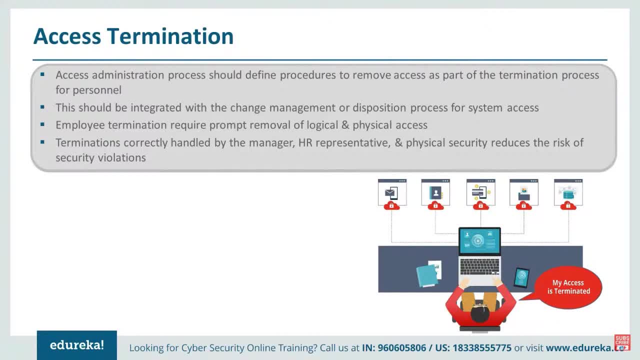 because, as a best practice, as a security practice, when we delete the account, the security identifier will be automatically removed and the security identifier will be enabled- I mean included- to each and any event or any transaction belonging to this particular employee. When the account is deleted, the SID will differ. 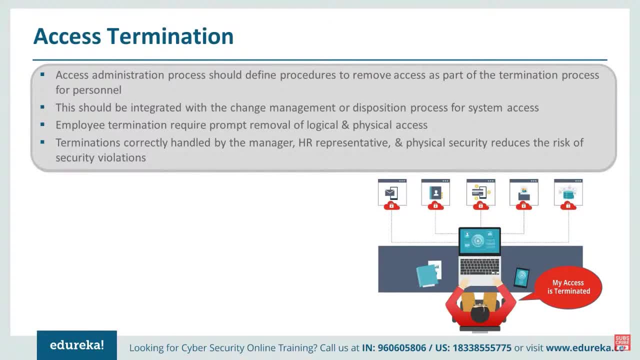 So when we recreate the same username, same account, it will not give the same security identifier. So it is always a best practice to disable the account instead of deleting it. So anytime in future, if things needed, we need to dig back into the logs. 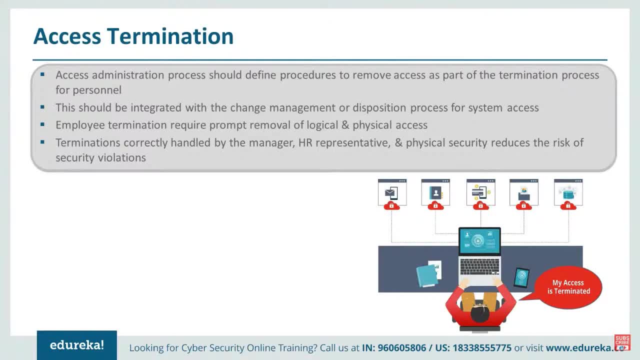 which were more than a year. Obviously, if we need to find what is the leak or what was the severity, the severity of the damage, we need to look into it. we need the complete information. So most enterprise will have the best practices. 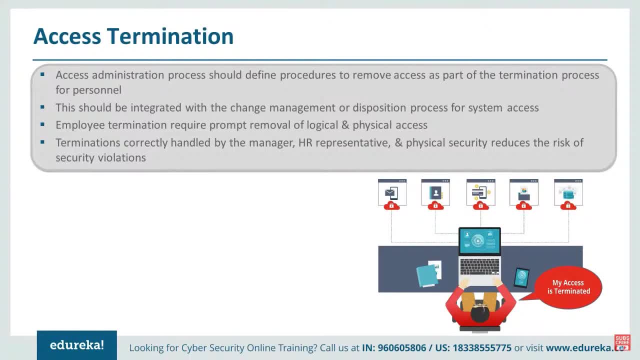 of keeping the logs up to six months in the hard bucket, So anytime anything can happen, so they can have it in lesser period and later on the older logs will be moved on to a safer storage location And the minimum period any enterprise will have maintained. 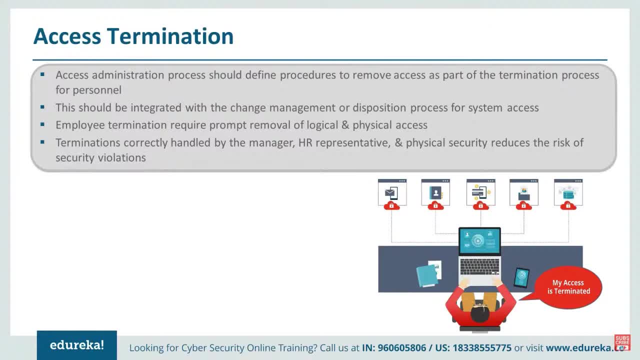 at least one year of logs for all the activities. So what's mentioned is the administrator purpose should be defined procedure. I mean the termination process will be taken care and the proper logical removal of a logical and physical removal of the access When the employee is out of the company. 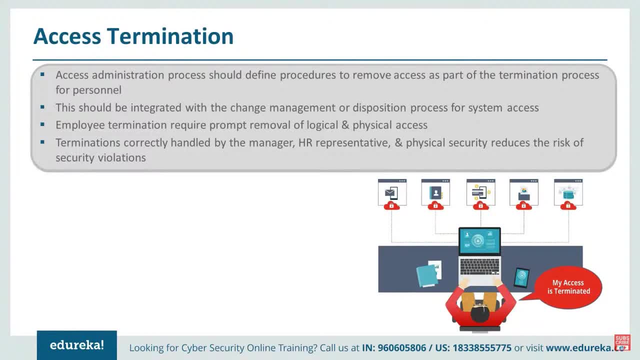 his access cards will be taken off And even if the employee did not submit his access cards, it will not be functioning when he comes back. So the termination thing will be handled in multiple teams: the HR team, the PMO team, the security risk team. 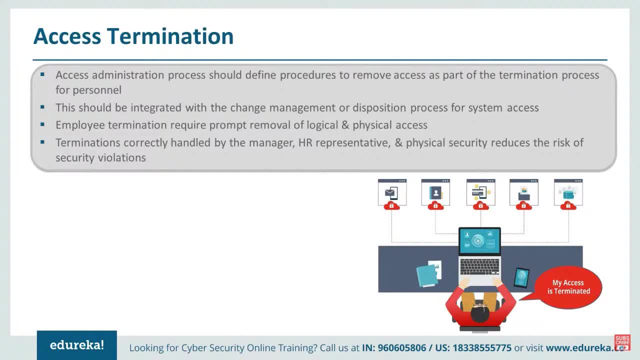 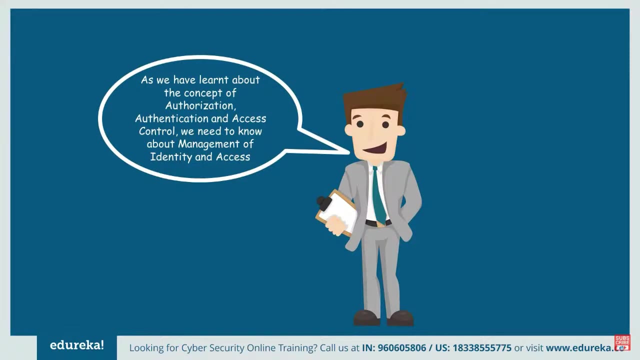 the administration team. every other team needs to be working coordination so that all the records and all the entries has to be terminated in the proper manner. So so far, we learned about what is authorization, what is authentication and access controls. We need to know about management of identity and access. 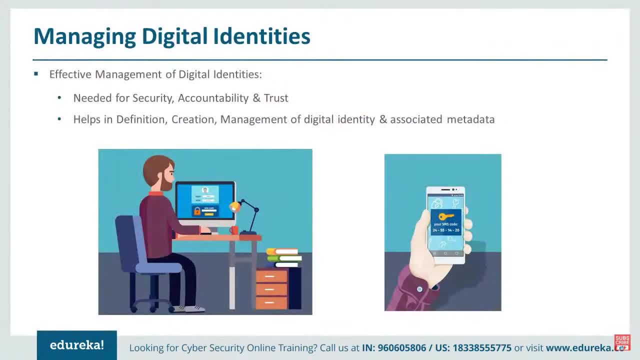 Now are we coming for the identity and access management part. So this is the picture. what it shows: a person is using a login screen. As usual, it shows a login page with the username and password. Below to the username and password screen, he sees a padlock. 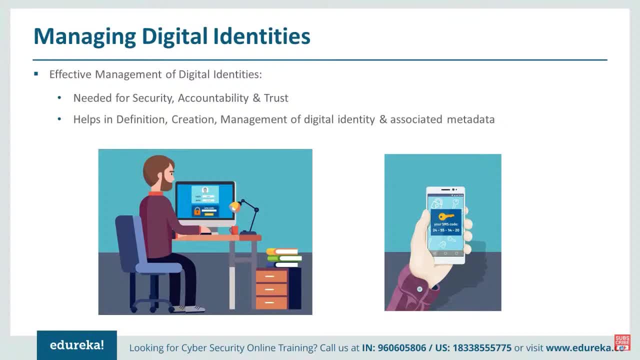 which also asks for a unique number or code. On the second picture we see that he received an SMS with the code 24541420.. Typically what it is, it is a one-time password, So the identity management is not only typically for the user account, anything digitally. 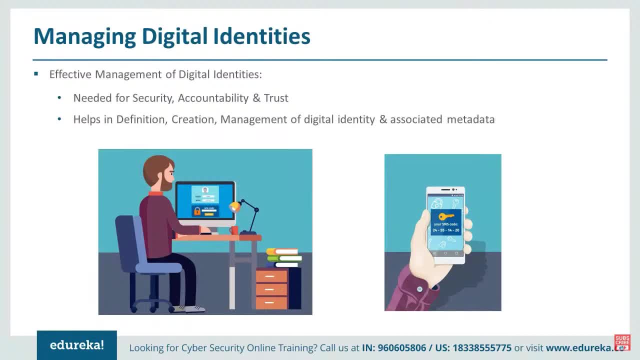 So this one? the user uses the multi-factor authentication. He uses a username and password along with the OTP and is getting into the network. So he's getting identified. What are the things getting identified here? The user's computer is getting identified. 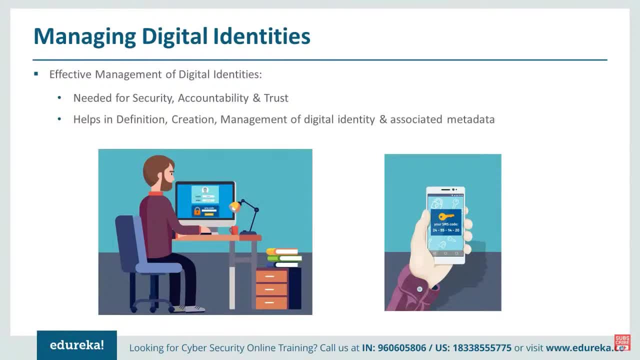 The user's name and password used for authentication and the phone number he used to receive the SMS. And if there is a mobile device management installed in it, the device in which the SIM card is present is also can be notified And at the time the computer's MAC address will be registered. 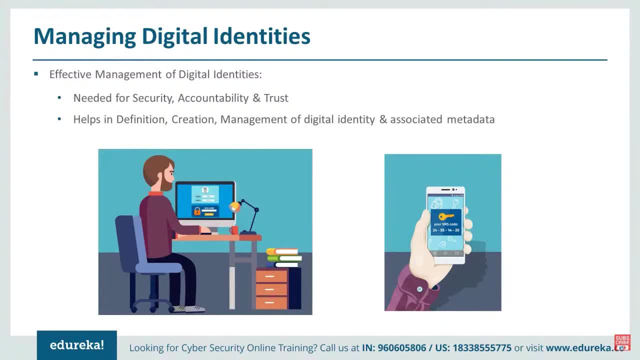 computer's IP address will be registered With the naming convention. we can identify whether it's a personal computer, whether it's a company-provided computer, what time he logs in. So with a single login session we can identify. we can collect so many information about a particular user. 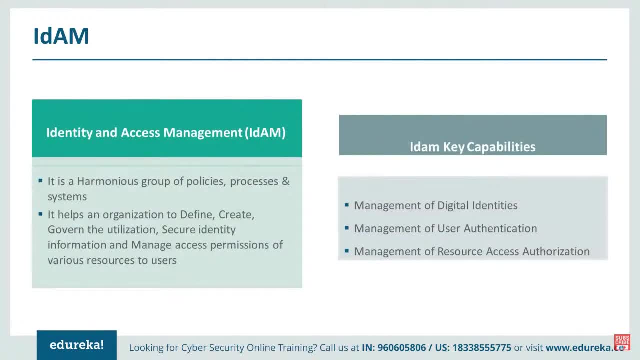 or identify the object. We can look into the. what is identity and access management? What are the key capabilities of identity and access management? Identity and access management is a harmonious group of policies, processes and systems. Harmony is integrated into policies. 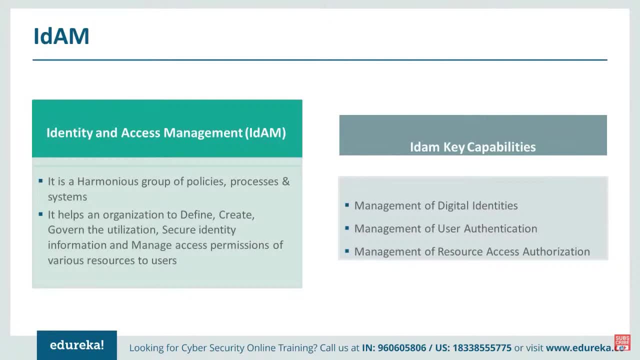 processes and systems. So it also helps the organization or enterprise to define, govern or create or identify the security information, manage access to the various resources inside the environment. So what are the capabilities? It usually helps in management of digital identities. 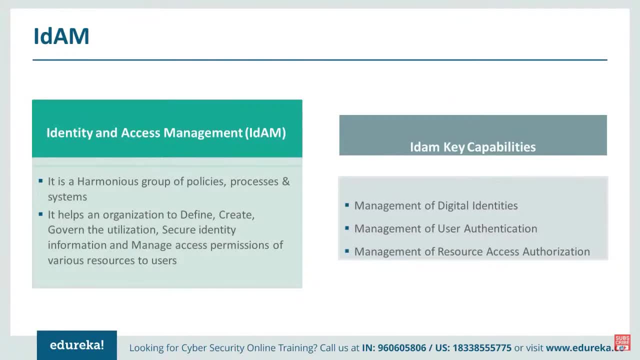 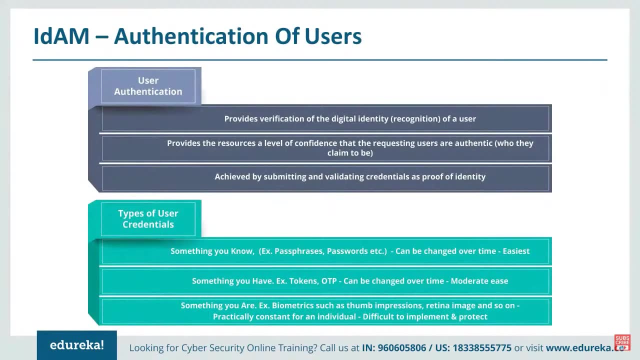 and also it manages the user authentications and it manages the resource access authorizations. So these are the three key capabilities of IDAM: User authentications. So it provides a digital verification or digital identity to the user. So what actually happens is when a user uses a username. 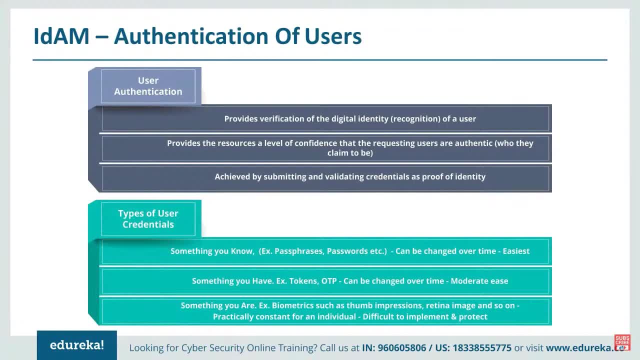 and password. he authenticates, he gets a digital recognition or digital ID, which also we can call as a session token or session ID. So the user authentication can be achieved only by providing a valid credential or a proof of identity. So, types of user credentials, what are the things? 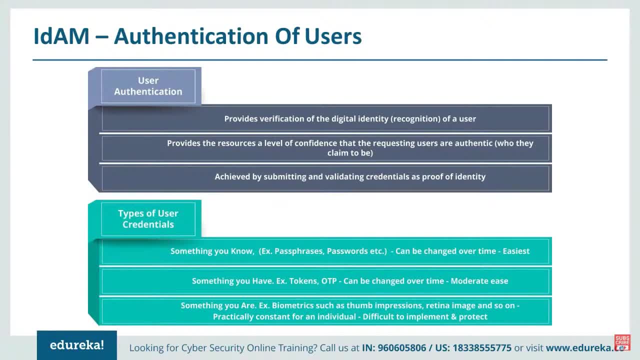 Something you know, what you know, that can be a password, a passphrase, anything can be remembered as easily, or anything which is not common, which is not unique. Only you knows that. So what you have, What you have, is tokens, OTPs, RFID, simple. 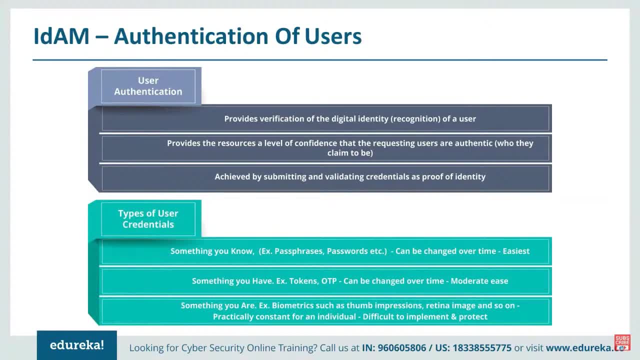 Your smartphone can be accessed or used as something. you have, Something you are, something you are. that cannot be changed. What you're born with, that should be always with you: Your retinas, your thumb impression, your image. Sometimes your face will change periodically when you grow old. 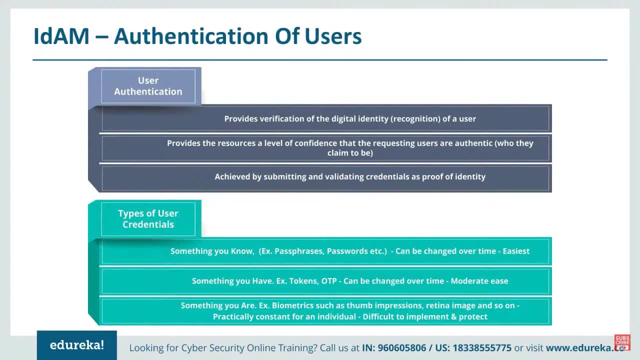 But the iris can, the retinas can, as your fingerprints. that will always stays with you most of the time, And what you do, something you do, that can be your signature, that can be your speech pattern, your the usage of words, or anytime somewhere. 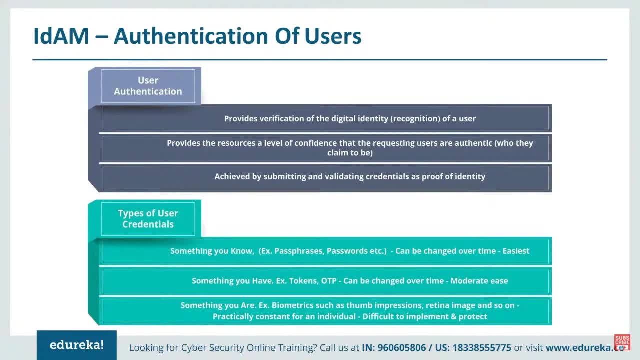 If people use have a tendency to use colors. Americans use different spelling for color- C-O-L-O-R, where in regular we use C-O-L-O-U-R to specify the same meaning. But the tendency of missing a U is also matching us. 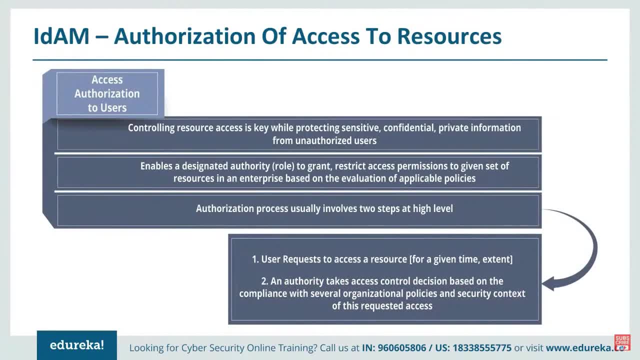 Something you do: Authorization of access to resources. what will happen is, once the authentication is complete, the controller reserves is the which decides whether to provide access to the confident information or the provided information. So as like the process which I explained to you before, 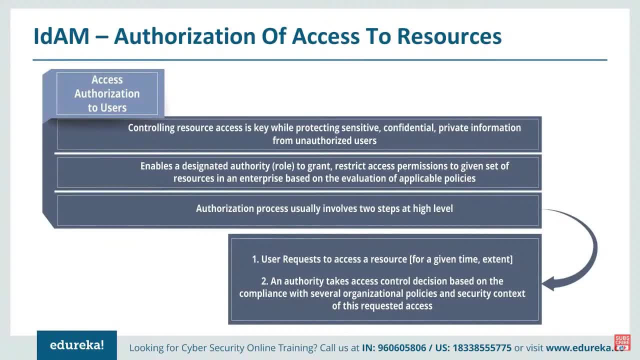 once the authentication part is done, the author is in part, where the user, the computer, the system will decide what are the objects, what are the resource, the particular, what the user needs to or at the time it's allowed to. 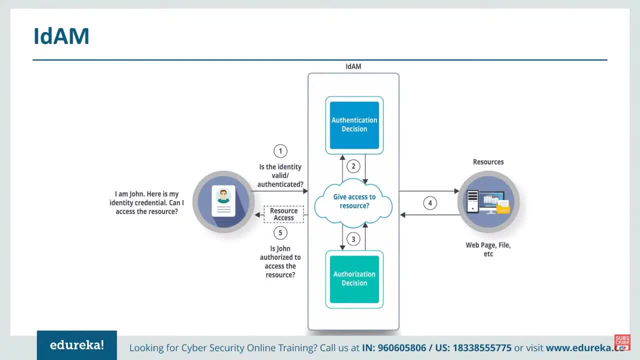 So this is a simple example how the IDAM workflow works. So the left- what we can see is Mr John. he shares his ID. This is John to the IDAM server. It will check initially. what will happen is it will check whether the ID is valid. 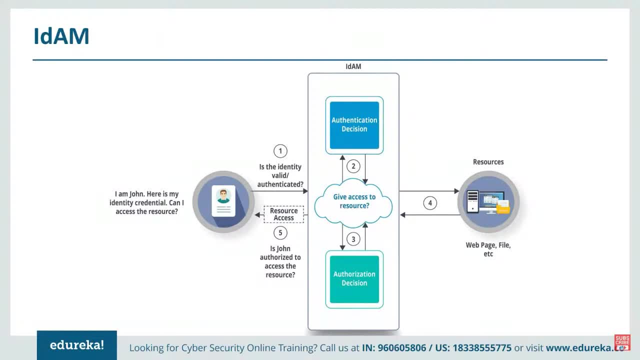 or whether it's authenticated. So it goes to the authentication dictionary, checks whether the he's authenticated or not and comes back. So once he's authenticated he'll be given access to the resource. So what is the life cycle of the IDAM? 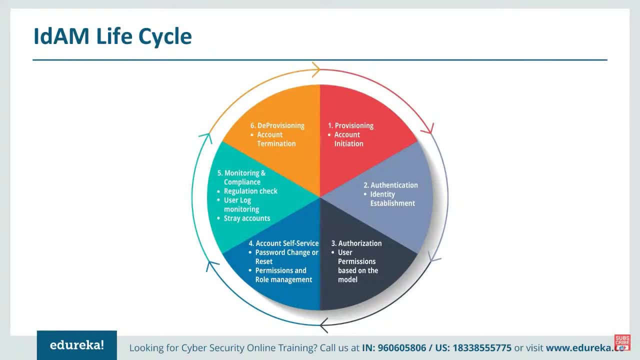 Provisioning of the account, I mean creation of the account, and second phase is goes to the authentication. So once it authenticates it establish a connection, secure session. So later on it authorizes whether the user is able to access particular model or object. 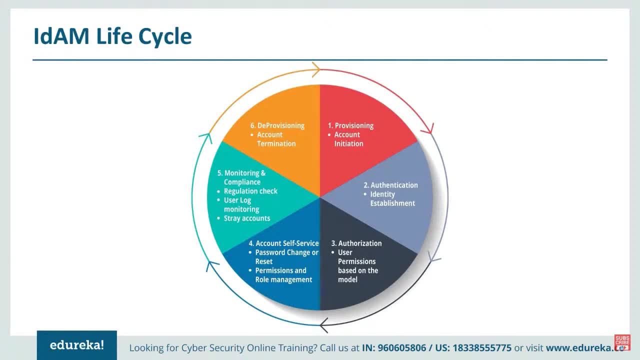 What are the other things a user can do? He can reset his password, He can request for permissions or he can raise a request or request for change in roles or change in assignment policies. through self-service With the IDAM, we can also monitor use of the resources. 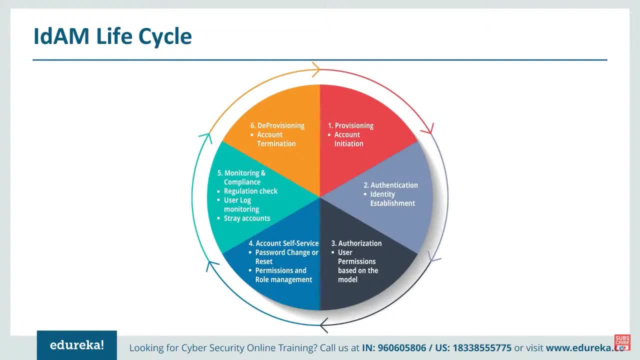 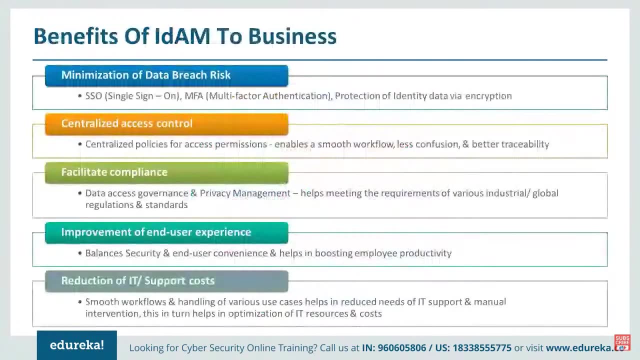 or any transaction happening digitally. You're using this session and also the termination of this account. This is the six components. This is the six stages of lifecycle of an IDAM. So what are the benefits of IDAM? two businesses Using single sign-on or using identity access management? 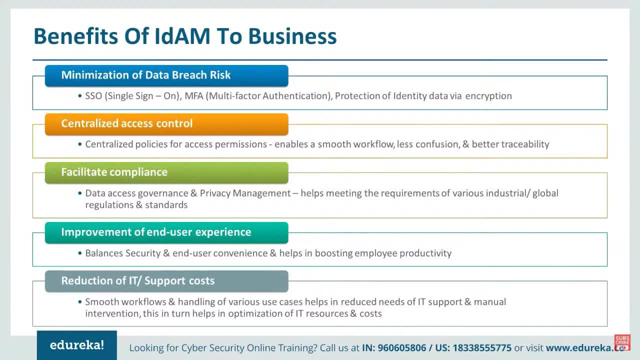 it minimizes the data breach. It helps us in preventing or protecting the resources from getting into the wrong hands. Only the simple concept of IDAM is providing right access to the right object on the right time. We need to give the right access to the right object. 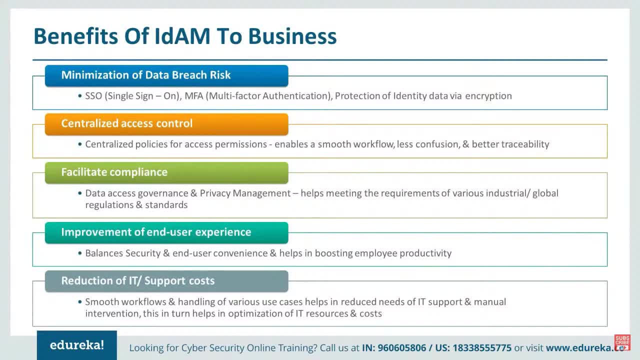 on the right time for the right user. everything to be on the right side. So, obviously, using a single sign-on or a multi-factor authenticated method in IDAM, it minimizes the data breach and minimize the risk of data breach, to be precise. 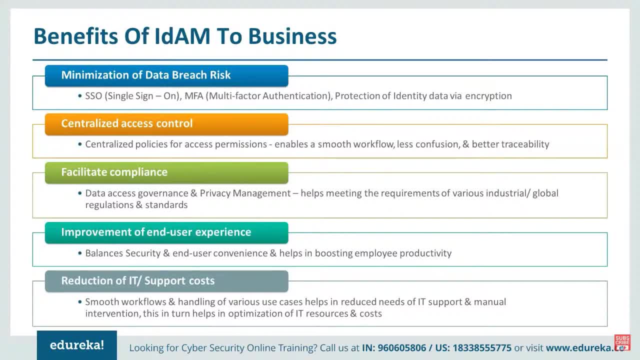 And this can be a centralized access control Instead of single computer. it can be in central location, Any DC can work on it, or we can install a separate server which takes care of the authentication and authorization part, not to load too much on the domain controller. 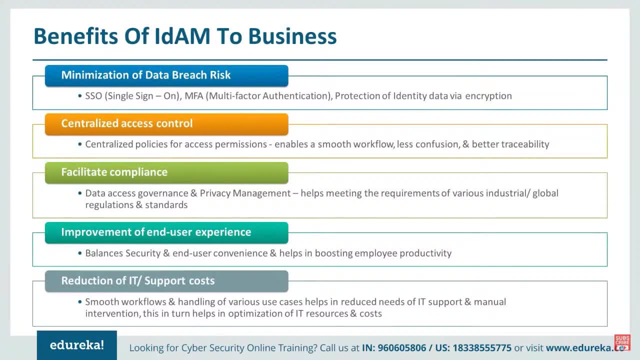 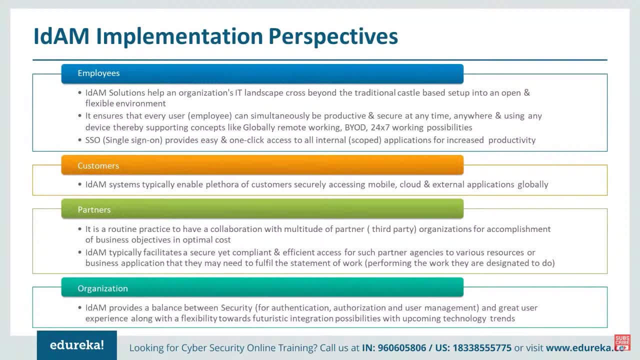 So also, as, like the DC, it can be centralizely managed, IDAM. it also helps the employees. What they can do is they can work on multiple devices, they can use multiple locations, they can use their own computers or they can have the concept of BYOD. 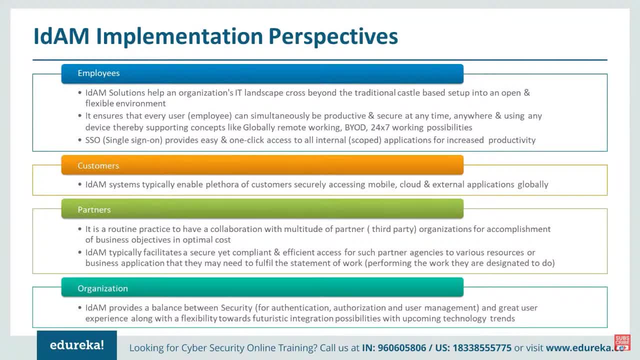 They can work anytime, any place. So also it helps us in getting the single sign-on. I mean instead of logging into the multiple application with multiple usernames and multiple password, when a single service will help the user to logging into multiple accounts. 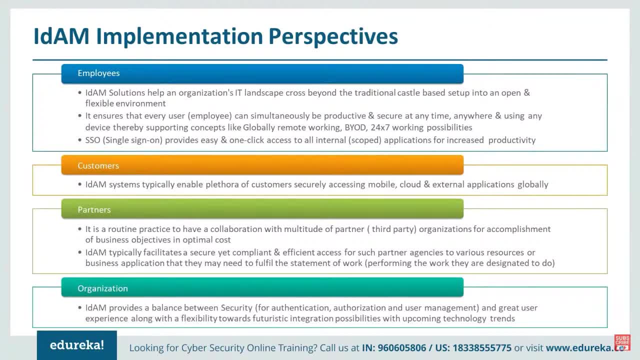 This is just simplifying the user experience, So when the user logs into the computer or the workstation with this corporate credential username and password, automatically he should be able to log into other services related to his work Instead of the user manually need to key in the password. 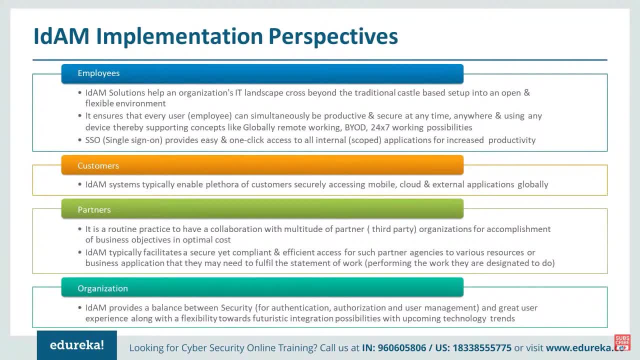 and username, So the identity access and management. it also comes in the Federation concept where a customer can use a third party resource or third party authenticator, For example cloud. if he needs to access cloud resource, he can use a cloud ID account authentication. 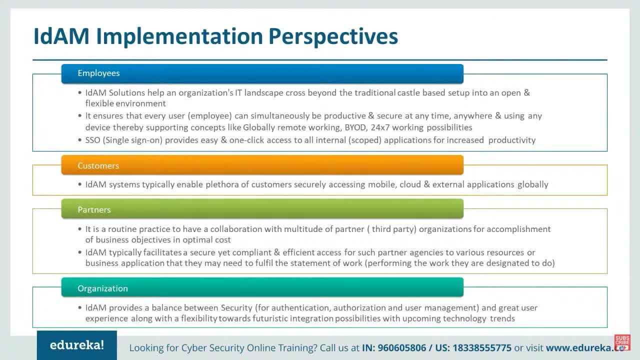 or a cloud SSO object just to authenticate And so he can access into the resource. So, for the partners and as well as the organization, IDAM plays a crucial role in providing the data security and also to the assignation of rights and responsibilities. 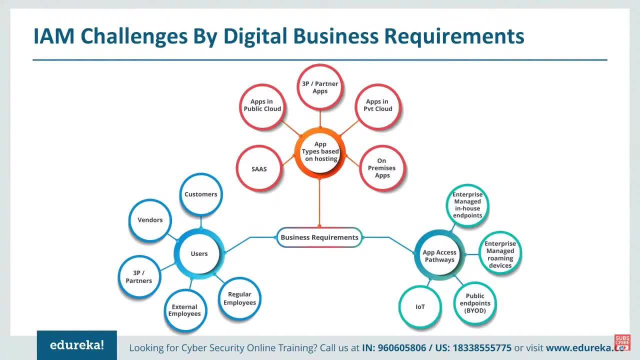 So this is a tree diagram which helps us in. what are the factors, What are the attributes which contribute the decision of IDAM? I mean typically the challenges faced by the business on using IDAM technology. On the left user may be communicating to the vendor. 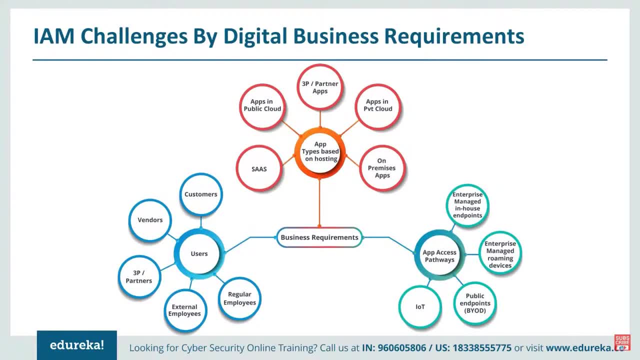 communicating to the customers or third party, external employees, employees, regular employees he may be, he needs to be communicated and his account needs to be authorized and authenticated across the multiple platforms. third party, 3p, third party- when it's in the user perspective, the user needs to communicate. i mean user interacts with regular employees. 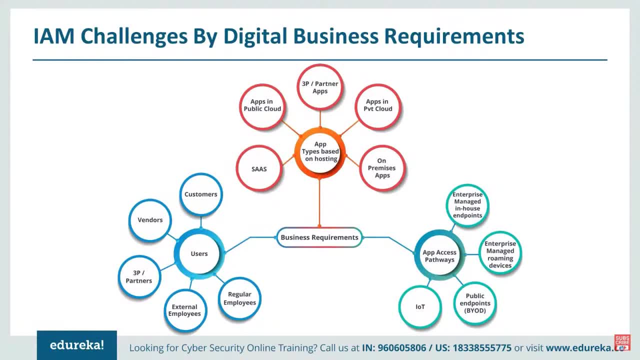 external employees, third parties, vendors, customers. as a user point, he'll be connected to multiple segments and where the user communicates with the business access path. it may be a in-house applications or in-house device, or it may be a public device, a bring your own device or iod. 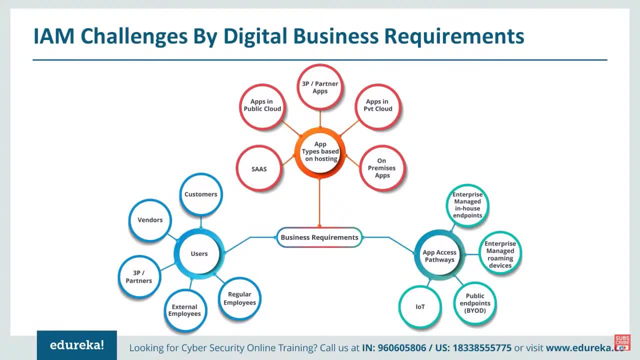 these are the device which are connected to the user, based on the business requirement and what again it goes on the software part, the user, the. towards the right it's an infrastructure and towards the top is the application: user, infrastructure, application. these are the three important things. what works on it? on the top it is a sas software as a service or on-premise. 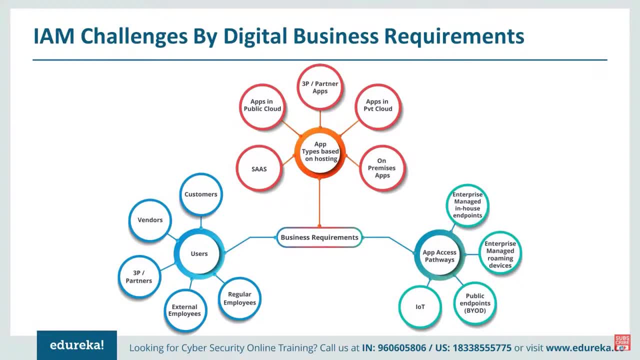 hosted apps, privately hosted apps, third-party based host apps. the devices, the user and applications need to be identified and authorized are granted access based on the business requirement. this is the complex. I mean. this is the challenges which are faced by. I am actually it. I am helps the enterprise to overcome these challenges. so what we see in. 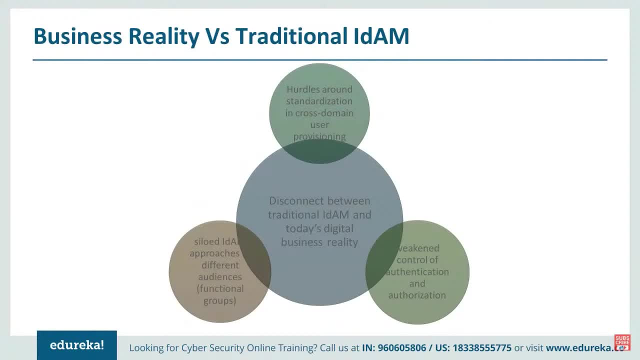 siloed item approach to different audiences. this is simply a previously: what traditionally, what we were doing previously and what word was happening in the reality. this simply a chart which express in it so what? what revolves in the center? it's technically disconnect, because what business things will not work properly in the reality. traditional concepts: 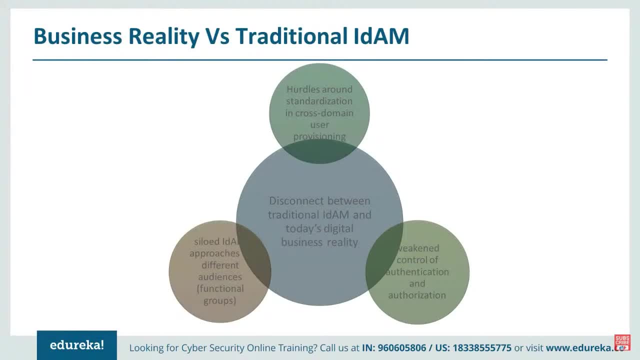 or the ideology. what we followed long back was not suitable for the right environment. typically, what it creates? it creates a disconnect between the identity and access management and the business reality. what also it does? it weakens the controls and it authorizes- I mean control of authentication. 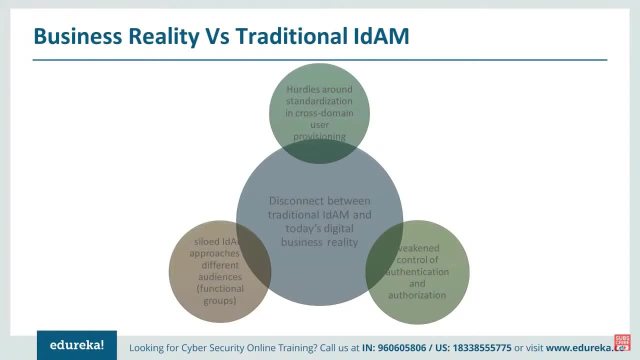 and authorization, the older traditional identity and access management. so for provisioning across domain access or cross forest domain and access that will not be working when it was not centralized or it was in the single concept or siloed item. so now getting the item centralized, everything into link it made our job so easy for 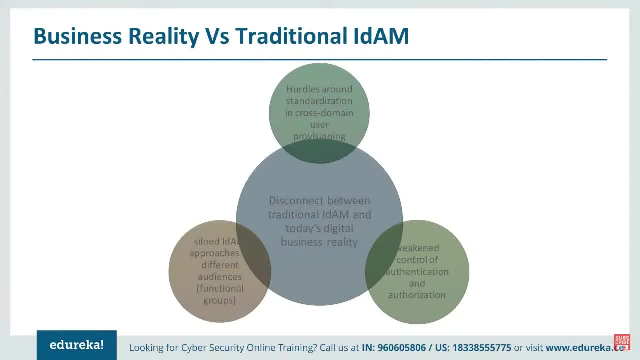 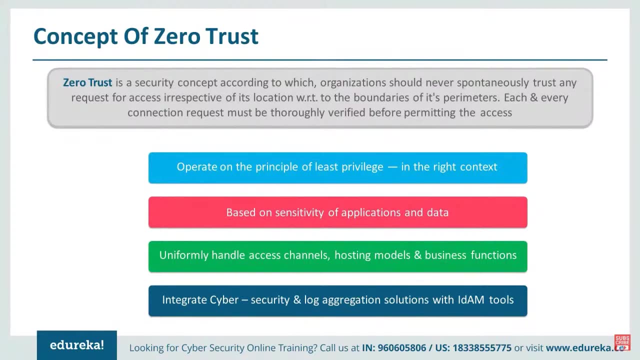 getting identified and accessed to the resource so easily across multiple platforms and multiple domains. so this is also one of the important concepts with the concept of zero trust. so zero trust is a security concept according to which organizations would never spontaneously trust any request from access. so zero trust is before investigating or before 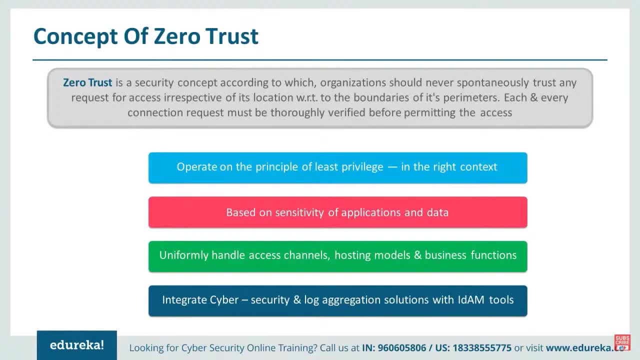 collecting the complete information or before understanding the actual need or actual purpose, any request will not be Solitiated. I mean it not be trusted. always work on the principles of least privilege and it will help us as a ensure the security of the sensitive application and the data. so what it says, the each and every connection request, must be thoroughly. 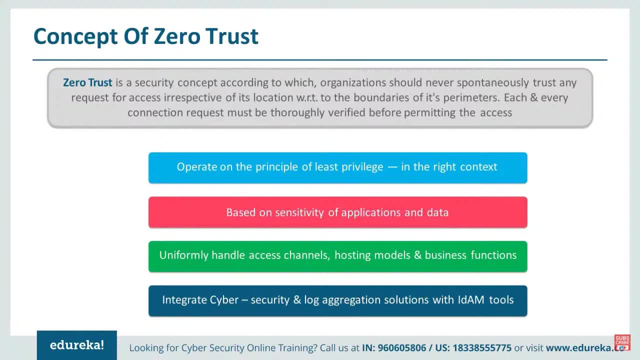 verified before permitting taxes. so that is how it accesses. so initially, when, after the authentication is done, based on the concept of the zero trust, no access, no rights will be provided. when we know about the firewall concept, what lies on the bottom, I mean very last rule will be block all connections. 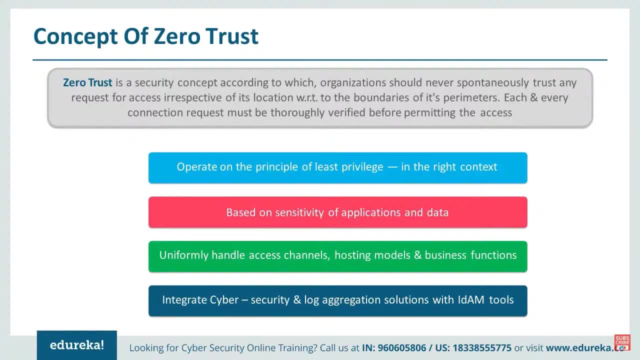 or terminate all connection. this is what actually has the rules that will be processed from the top to bottom. the bottom rule will be always block all not to provide deny access. This is the thing which is the last rule will be processing. So when we stack responsibilities, are rules above. 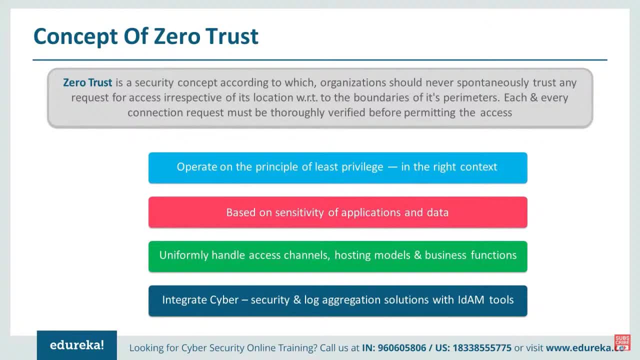 that the rules will be processed from top to bottom. above block, all apps I'll be giving access provide access only to MS Word. So this is the only rule which is above that I mean applied, so the user can use only the Microsoft Word. 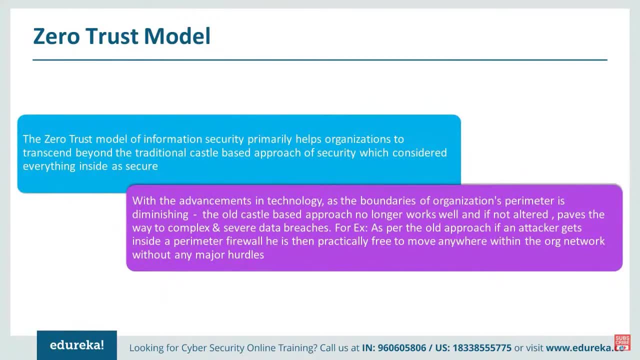 So anything else will block. the zero trust model of information security primarily helps organization to transcend beyond the traditional Castle based approach of security which considered everything inside is secure. So what initially happened is same. like a castle, We cannot think the peons, the workers, the soldiers. 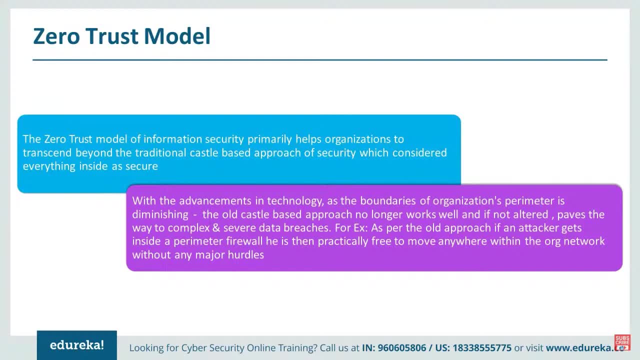 or the ministers who are all inside the castle. That does not mean that everyone is safe or everyone is trusted. So the same concept goes here. anything inside a corporate environment or enterprise environment cannot be treated as secure until and unless it proves it either identity or authenticity. 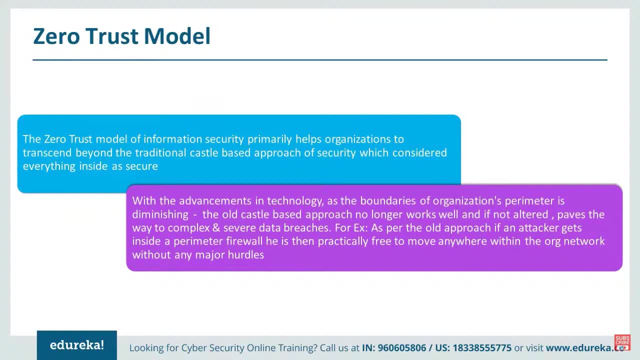 So it is always a concept of not to trust anything and everything. one more advantage What will be having is, when we don't trust anything will not be sitting idle or will not be comfortable setting up one thing: when we stop trusting and start suspecting. 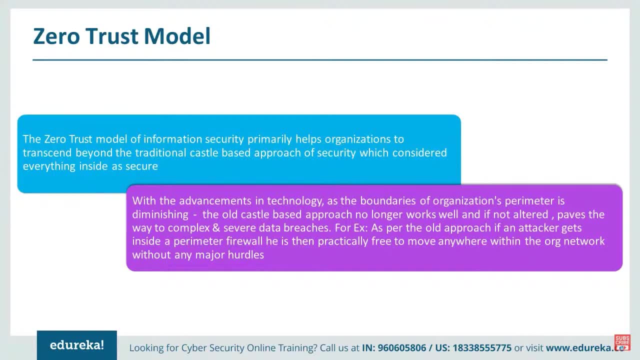 Anything and everything in the secret, because this cannot be applicable for other people, but the people which we, who we are in security field, is obviously we need to be more cautious and be more suspicious on any activity. Anything can be malicious if brute-force attack- and I can, because I can simultaneously block connections from a particular IP. 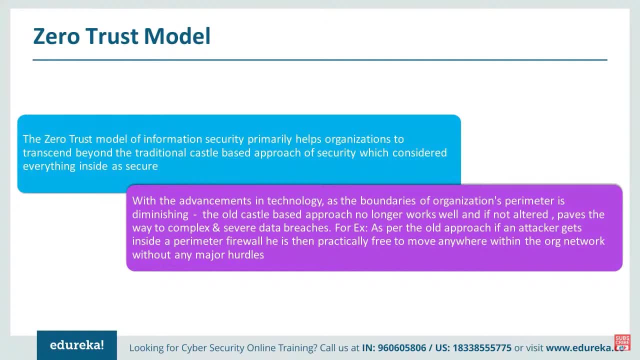 to be simply enough, I can provide access from a particular IP to the particular device, only to a particular port. But if he tries to connect to with the multiple Ports are three or four ports within a minute or within 30 seconds, I'll be terminating the connection. 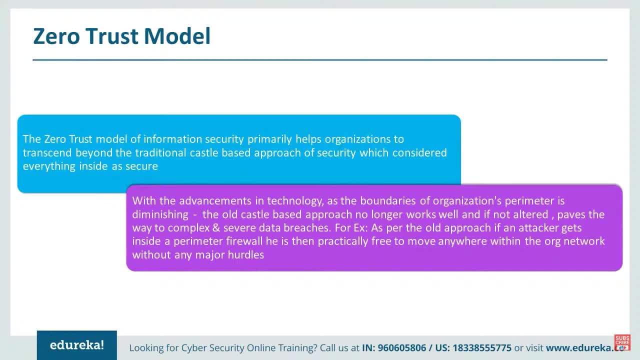 So, simply, what I'm doing is I'm just blocking the port scan. If a connection is established through a particular IP, particular port, that's okay. that as long as this session getting expired, it will be available and no disturbance will be hindered or no one will be taking care. 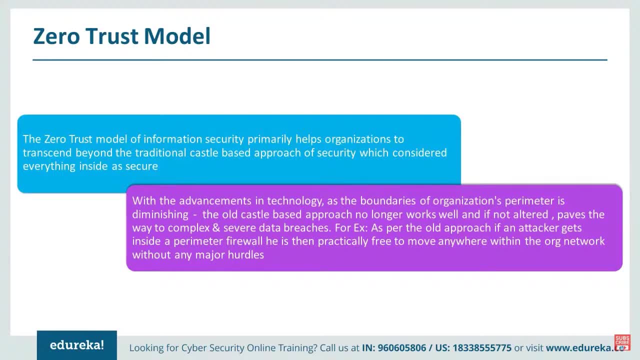 But the same thing if it scans for other port, are trying to connect in a different port one or two times in a minute, obviously the suspicious, the attacker. now they are not busting the attack. The 65,000 535 ports can be scanned in a single minute. 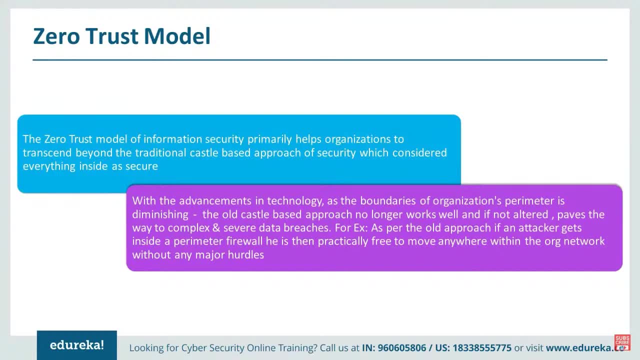 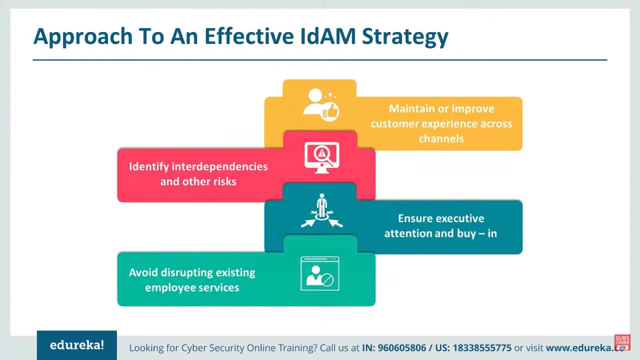 But if they does so, it will initiate the alert. So the scanning mechanism is already lowered down. So, scanning a port to permanent, two ports per minute, three ports minute, We can create the conditions. So, likewise, anything or any transaction will be monitoring and will be thinking in a way or seeing it in a way: how suspicious. 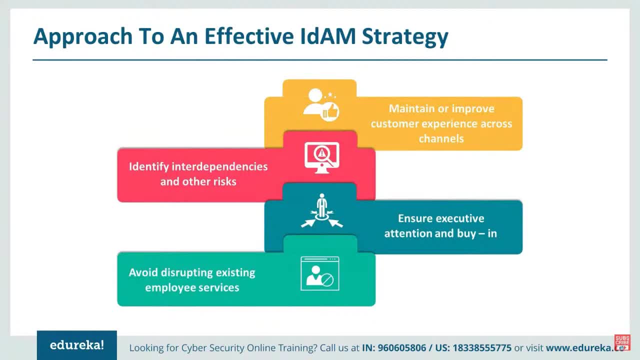 this particular behavior, particular action, can be lead to. what are the approaches for an effective item strategy? So what would be the thing? it would improve the customer experience across all channels, the all-channel channels, in the mean of being a cloud-based resource or accessing the resource from multiple domains. 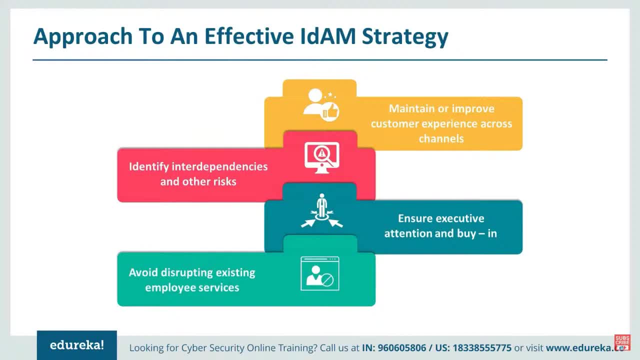 or accessing from multiple softwares. even so, there will not be any identity interdependencies. So, okay, there will be identity interdependency: one identifier will be linked with the enough rights and rules. This will not be applicable To others. every unique identity is unique. 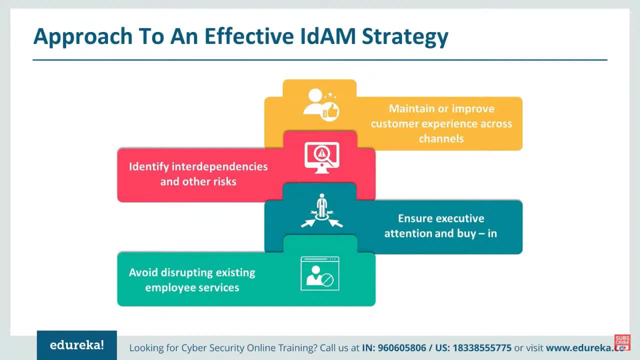 So also the attention is executive attention to buy-in. So when the proper item strategies in play, it will not give a disruption to the employee services or it will not hinder anything to the regular activity. two-point star interdependencies: One unique identifier linked with other things. 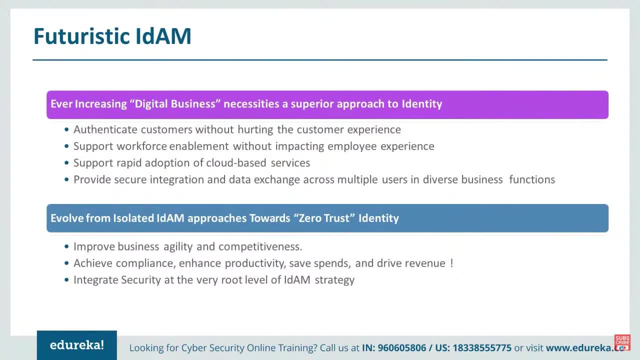 So what is the future of identity and access management? So the infrastructure, what we had before four years is not right here. Most of the time we need corporate adapted using cloud-based applications, some like Salesforce ServiceNow. so most of the companies which are up the cloud-based model software as a service. 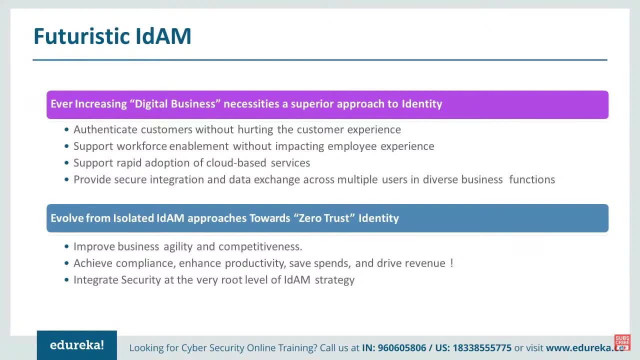 for accessing in to the cloud-based service. We definitely need a cloud-based authentication mechanism that can be routed to a in-house item solution or a cloud-based item solution. The authentication and authorization will not make pain to the customers. It should be fluid and it should be transparent. 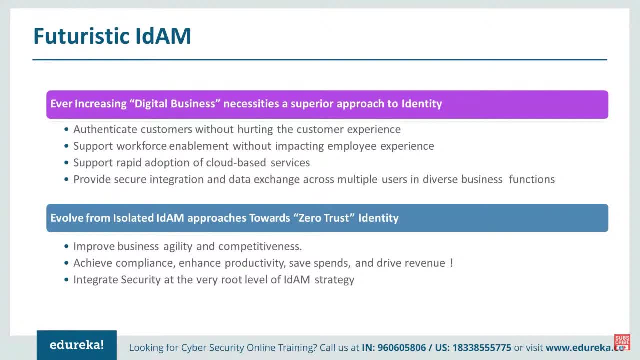 and it should be happening in the background. and lesser number of time, smaller fraction of time. It should support the rapid adaptation of the cloud integration between integration and data exchange between multiple business diversities. You might be seeing that you can use a Google account to log. 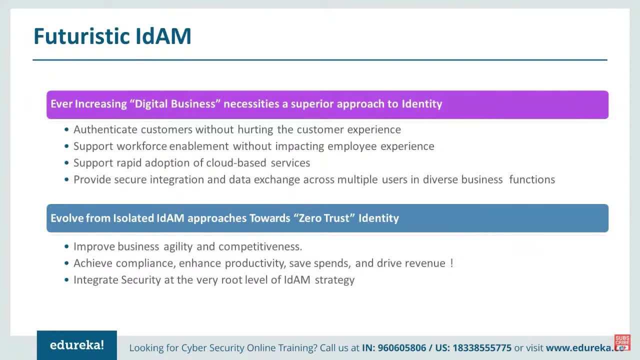 into Facebook, or you can use a Facebook account to log into Twitter, or you can use the Facebook account to log into Instagram, So single account can be used for accessing or logging into the multiple accounts. This is a trust model. will be also talking about the trust model. 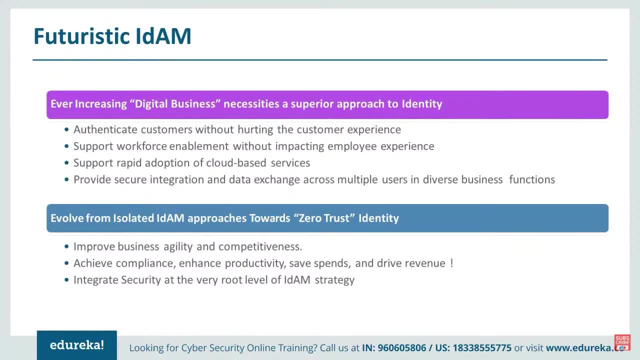 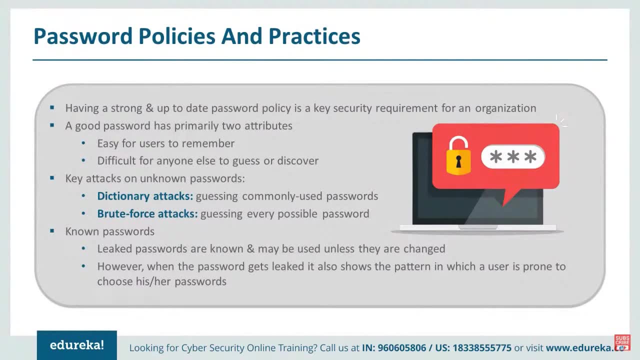 how it works and how the sample open ID OAuth method. those works. password protection So far. we already spoke about password. What is the best practice for the password? password should be kept secret. only then it can be called as a password. The password should be easy to remember and difficult for anyone else to guess. 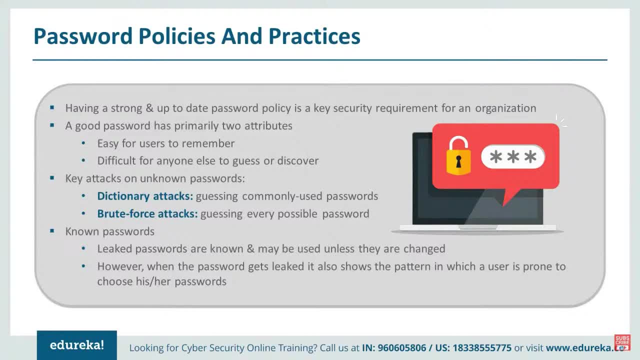 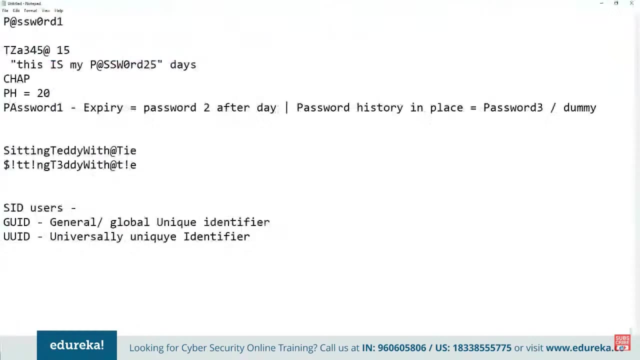 It should be easy for you to remember, but it should be very difficult for the rest to guess what exactly the password could be. usage of multiple combination of words, numbers and alphanumeric characters. special characters. Sometimes even people will have a tendency to code all 256 characters. 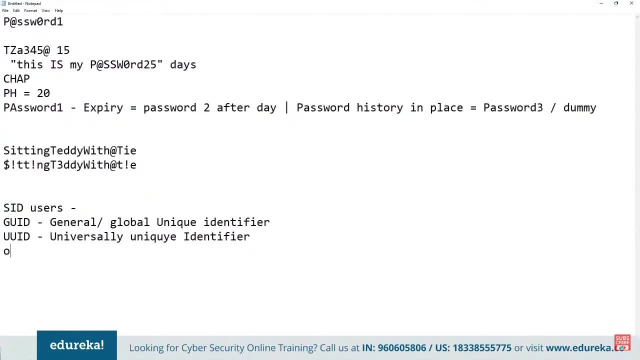 when you hold on alt key and type in triple one, It will give a different character. This is not exactly Oh, not even a capital O. You can just test it. open a notepad and hold on your alt key and type in 0 to 256.. 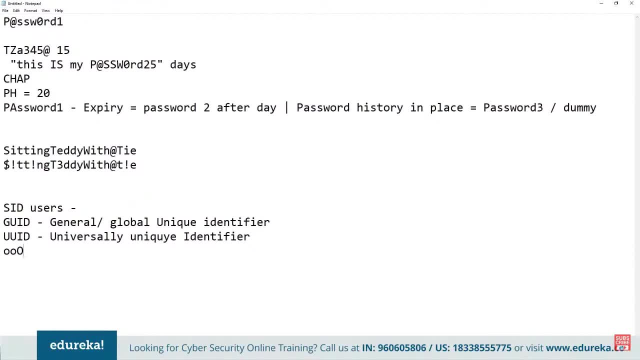 You should be getting a unique character that will not be usually available on your keyboard when I hold on the alt key and press 2 to 0. I'll be getting this block character. This will not obviously be on the dictionary mode when you use these kind of special characters. 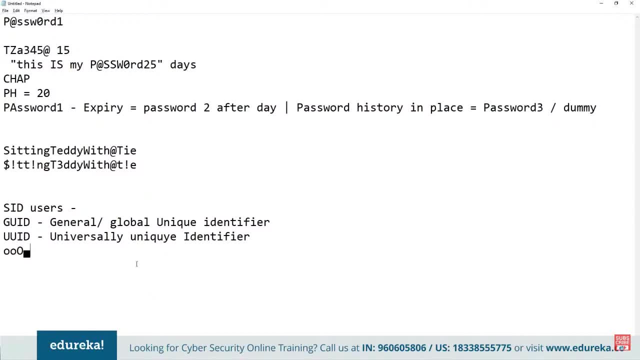 You cannot break into the password, simply test. I'll hold the alt key and press 1 2 3.. I'm getting the braces, but it's not equal: alt 2 2 3, alt 2 2 4.. So these are the characters which will not be. 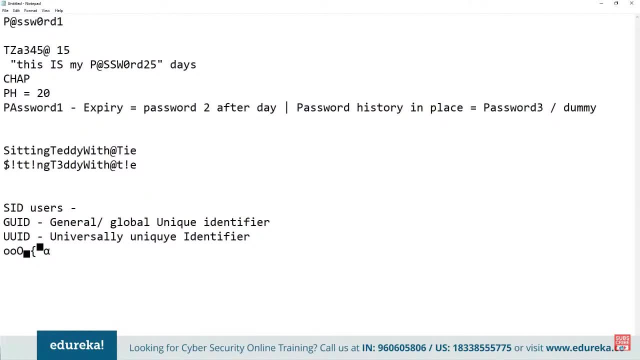 Usually used by the customers. What the pattern or the dictionary mode have is what are the key characters available on the keyboard layout. If it's a uk-based keyboard, the characters will be different. The us-based keyboard. using this base keyboard, This is different. 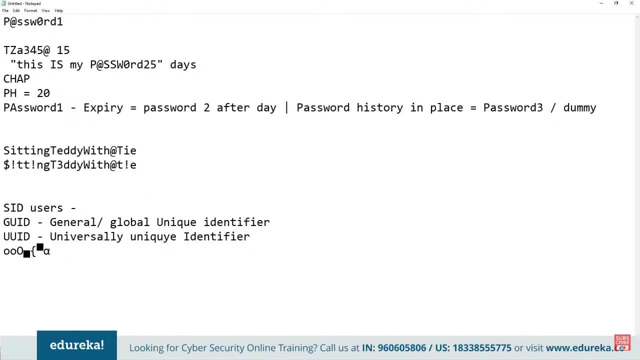 The French keyboard characters will be different. The Russian keyboard characters will be different, but using a combination of multiple characters or characters which is not in the dictionary or not in the brute force title, We can always say: secure that the password cannot be a guest. 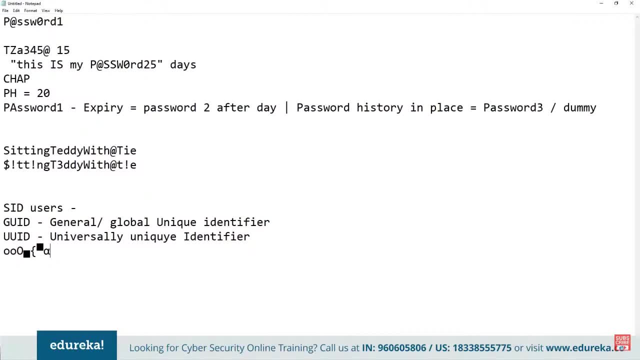 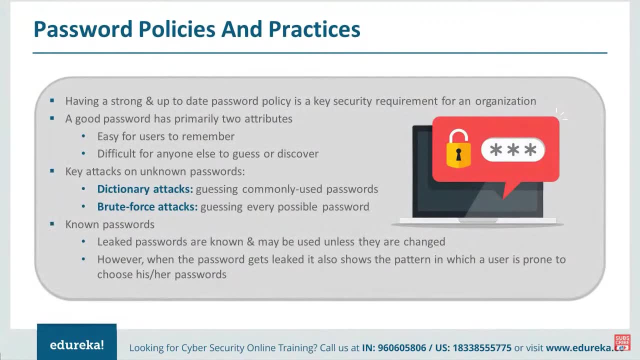 even when we type something in 001, password cannot be guessed and password cannot be used on the dictionary mode or brute force attack. You can also use the ASCII table to find it out. So what? let us test what happens when we try holding down the alt key. 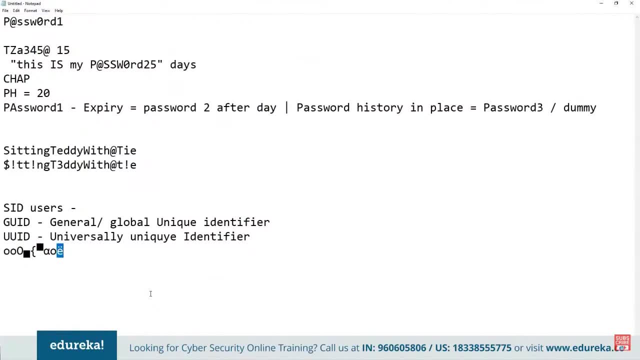 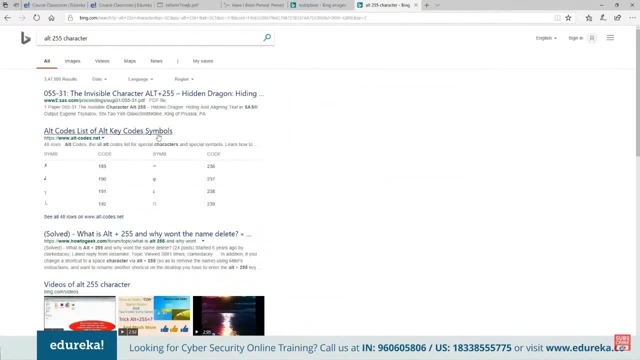 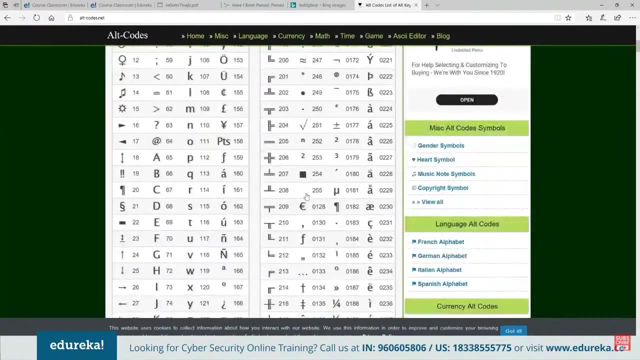 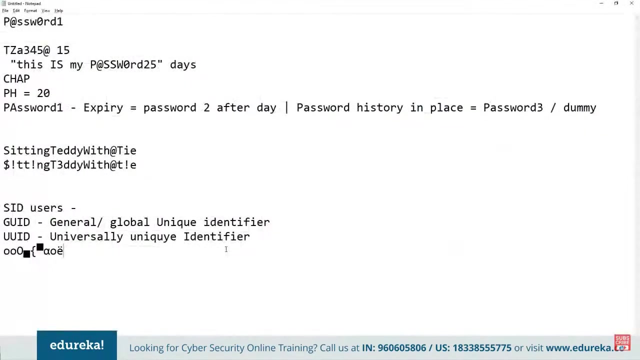 and 1 3 7, alt 1 3 7. based on my keyboard layout, It gives a different symbol, So I need to get this symbol. 0 1 3 7 says let's type alt 1 3 7 or 0 1 3 7. 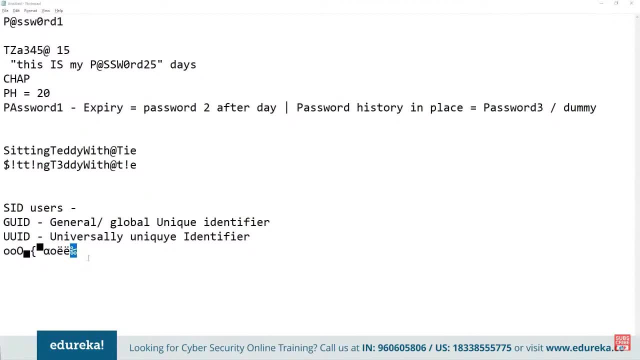 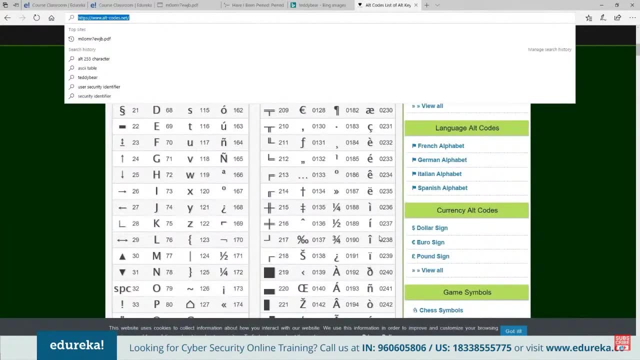 when I key in 0, 1, 3, 7. It gives me the same symbol. You will not able to find this symbol on any keyboard layout. You can simply refer to all codes: alt plus the 255 keys: 0 to 255 keys. 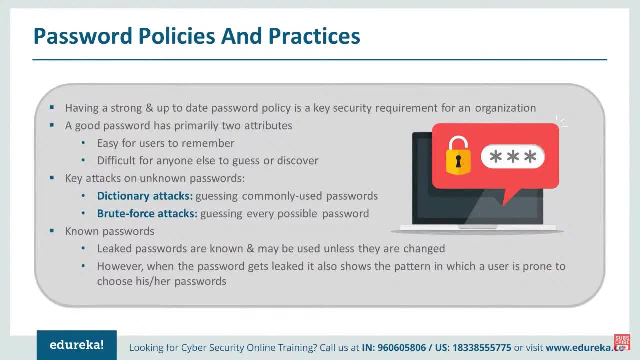 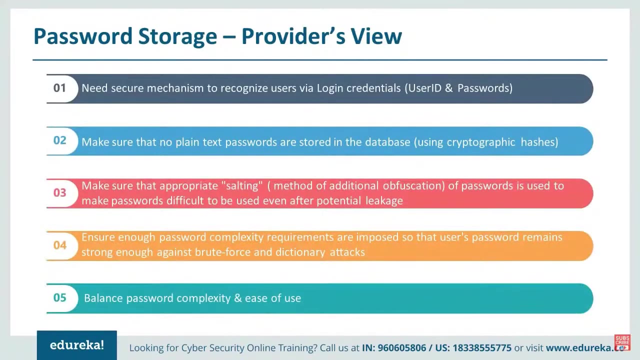 and not to use the known passwords In the past. It is common. when the password is available and applicable to any other user account, It is obviously useless to have the password, So we should be having a unique password or password remembering techniques or storing the passwords in any password wall: password storage. 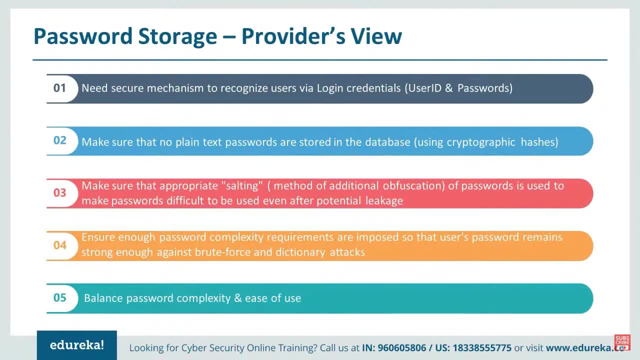 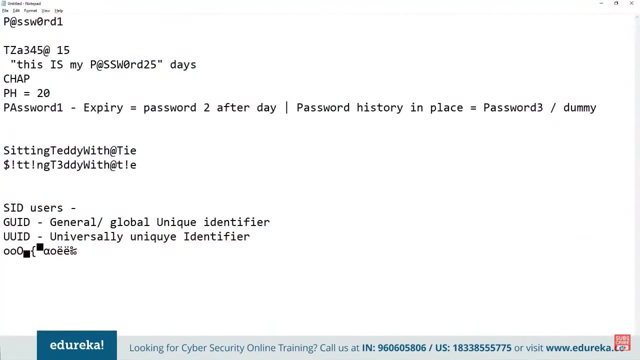 The password storage mechanism will obviously have a unique way or unique hashing mechanism. It also uses cryptography to store the username and password. It also uses a special salt, what we call a salt, adding a unique characters. For example, if my username is username and it, which will give a hash value of 1, 2, 3, 4, 5, 6,. 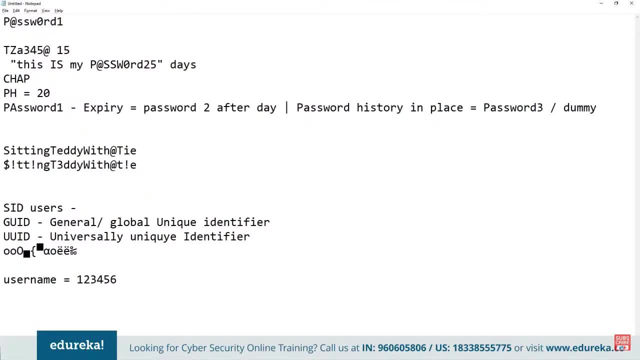 but salting is a special character. include along with your include. I can make this as a special hashing character. I can place this end of the username. Sometimes it may be inserted in between the username or it may be start of the username, or multiple hashing values will be introduced: multiple. 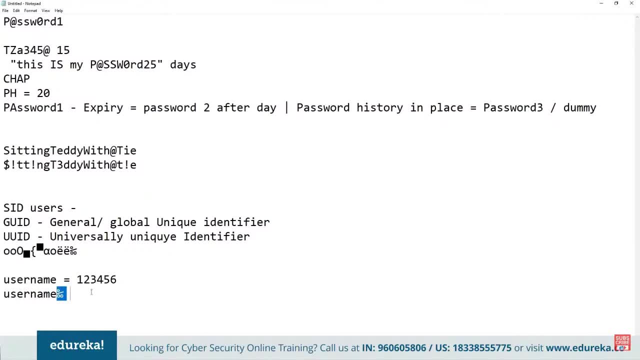 These are the salting values will be inserted. So when the salting value is inserted, I'll be giving a different hash value: 1, 2, 3, 3, 4, 5.. So this is how the hashes will be stored and this is will the hash mechanism also works. 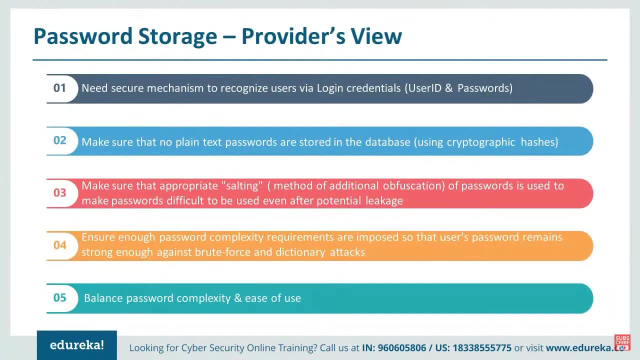 So it is not easy for a brute forcing the hash values and getting back to the original state. the usage of the particular salt value is determined by the time or multiple factors, the length of the string or the time of the input Method or the keyboard letter letter, anything that can be. 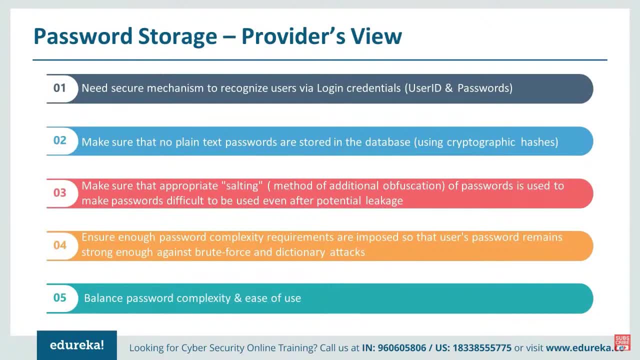 so it will just hash your username and password and store only the hash values. So reverse breaking here using a rainbow table attack to retrieve it back. It's typically pretty hard because most of the time the md5 values are broken and the list of values in md5 is already available. 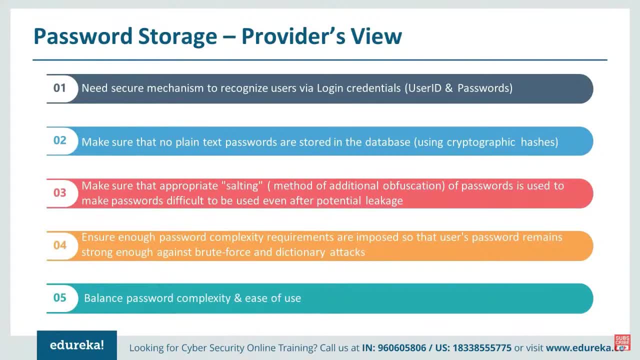 on the internet So it's available. But, as I mentioned before, the hash collision to you values can have the same hash values. I mean if you have data, I have one MB file or 10 GB have file. both are different but sometimes the due to the limitation of the hashing, the md5. 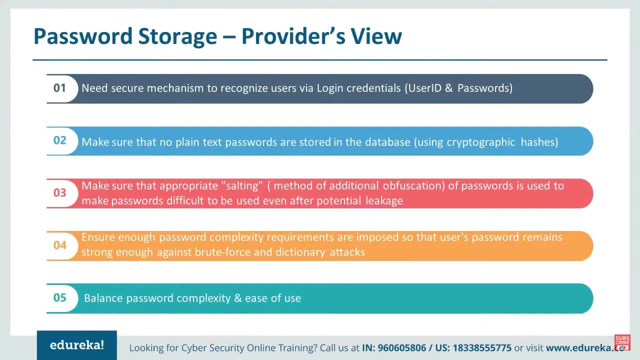 value may be unique, But what happens when the password, also password manager, also uses the same md5. We cannot match it because the older md5 is already broken. at same hash will be available for the multiple one. It is hard for us to identify what to key in. 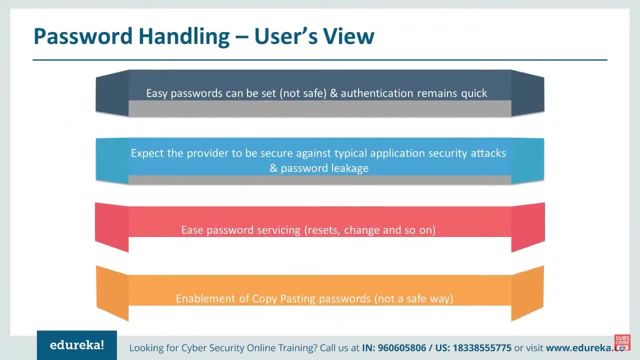 and how to retrieve it back. So what a user things on the password. The user things. when I have a simple password, it will be easy for me to get into it and I can remember it so easily. when using a simple password, It obviously higher chance of getting the account get compromised. 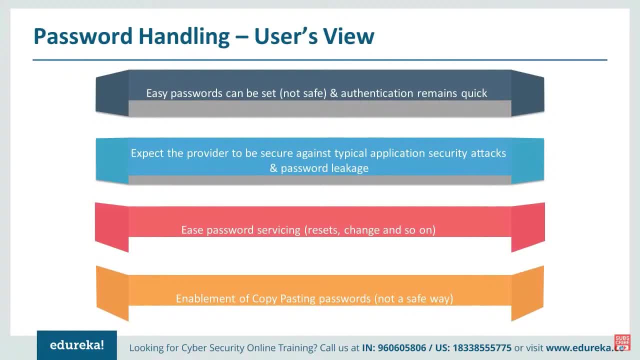 So whenever a password is provided to you, pin over a default password is given to you, Please reset it and use your own complex password and always do not write it down or do not share it down or do not disclose the password at any means. demo one. 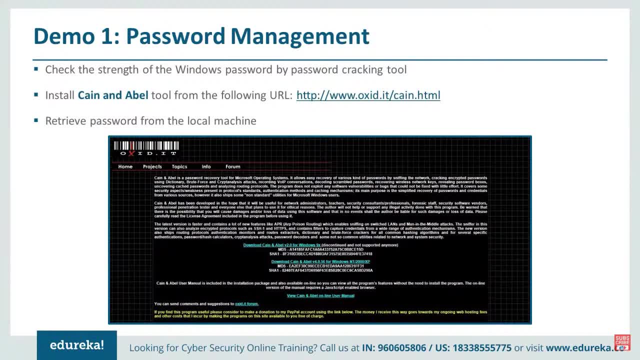 This is cane enabled tool. cane enabled tool cannot be run on a latest machine because it needs an older XP 2000 mission. This cane enable is a tool. It uses the dictionary and rainbow table attack, brute force attack to retrieve the password. but we don't have the latest one available. 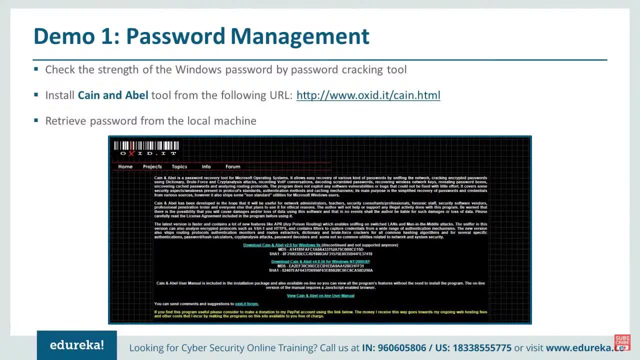 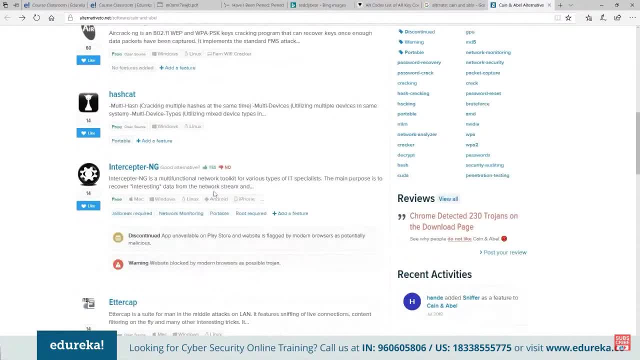 Someone has the older configuration file- I mean older computer- and they can definitely test it. Okay, the John the Ripper air crack ng hashcat intercept ng. These are not available for window based operating system. All the software seems to be Linux based. 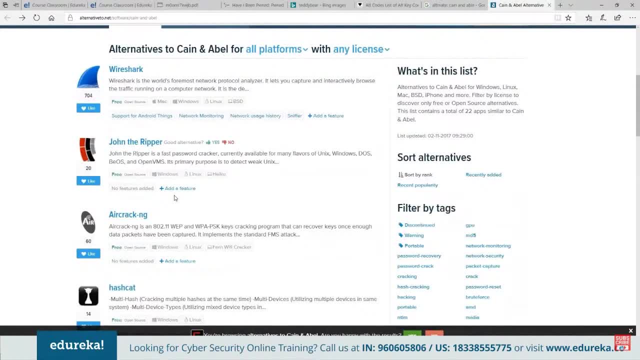 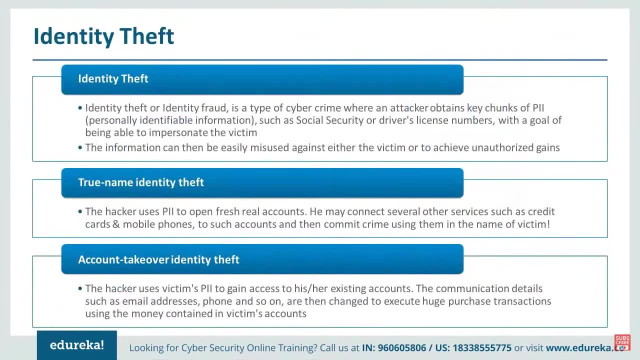 and these are the default tools which comes along with your call, your spirit. distro at our cap is one of the tool which helps us to capture the Ethernet traffic. So what happens when your password is compromised? your account is compromised. Obviously, the ID tip happen. nowadays people say: 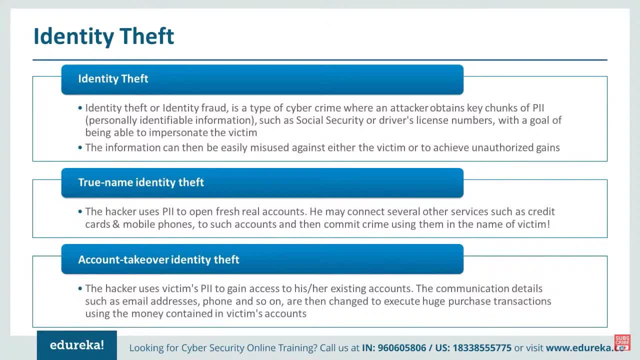 that my account got hacked after some vague or unwanted post on the wallpaper. I mean wall page. So nowadays we people see, keep on repeatedly hearing that my Twitter account Got hacked, my Facebook account got hacked. This is when one account is compromised, It obviously lead to other accounts as well. 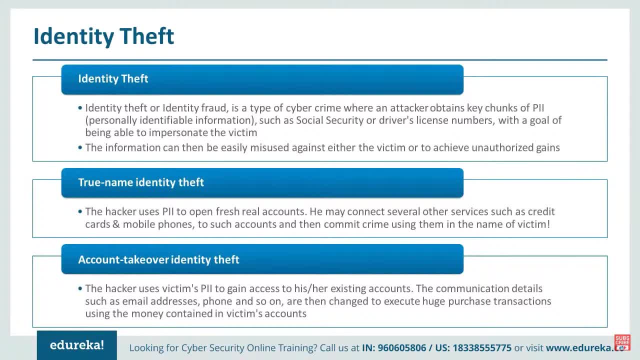 The attackers were so smart, He might be trying your username and password on multiple platforms. Not only he knows your Facebook password, He will not be sticking along with your Facebook and just digging what you did and what you want to, just to chat on behalf of you. 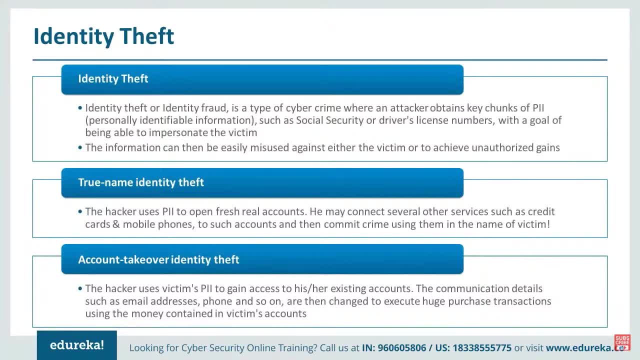 If someone has access to your account to obviously people think that you're the person working on it. when we have email address compromised, we might be having the telephone bills. your statements- bank statements are. most people might be configuring your email address as your password recovery mechanism. password recovery source. 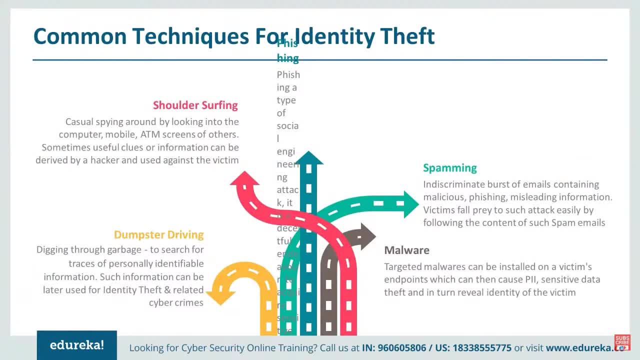 So, once so, what are the common methods? identity theft happens. shoulder surfing is simply watching from your back or watching from your side. What the pin number or what the password you key into the computer does is called shoulder surfing: fishing maybe emails or pop-ups. 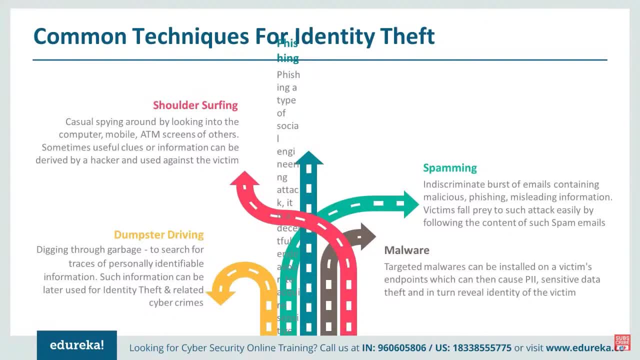 Which takes you to the wrong page, which actually resembles like actual login page- most fake Facebook pages or bank login pages which the appearance would be similar or close enough to the actual trusted side, But the intention is it will get the username and password in the background. that is called fishing, spamming. 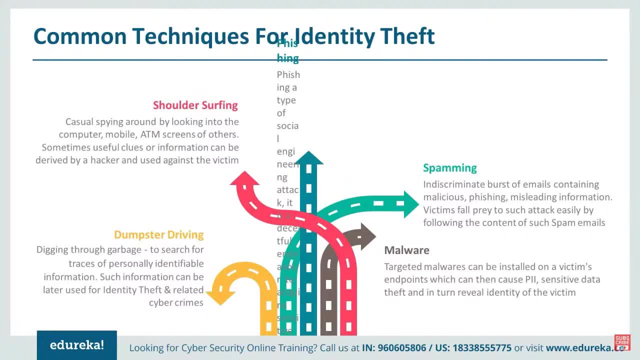 Also can be of the same. the spamming leads to fishing when we send multiple alerts. because when we craft an email for you, when you repeatedly receiving a particular type of email or particular time of form, particular type of information, what it says, for example, your bank account needs to be linked with your other card. repeated message. 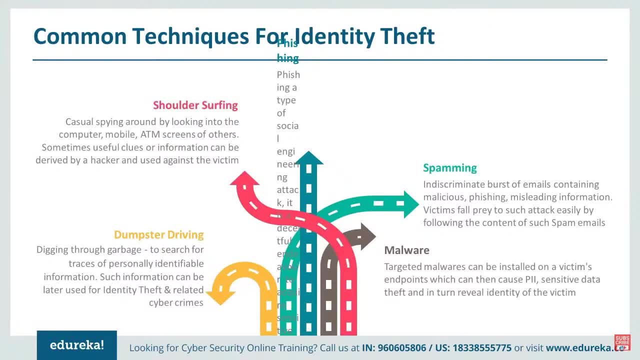 I'll be receiving one. the next email. your bank account needs to be linked with your other card. So one or other you might be missed, because when you keep on repeatedly seeing some information, you obviously have a tendency to remember the fact. Okay, I need to link my bank account with other card. 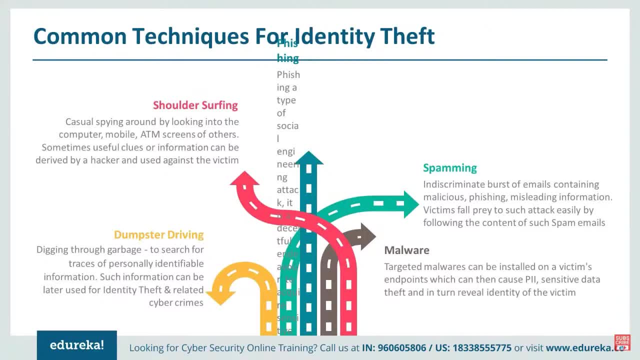 So, unknowingly or knowingly or without any precaution, you will might be clicking on a link And it will be taking to your page, which should also be resembling like a actual bank login page, But when you enter your key in your username and password, 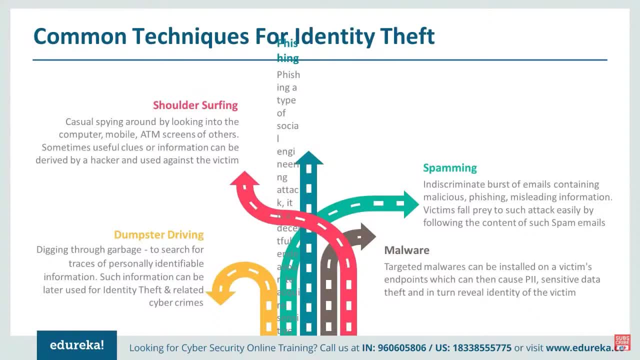 you will go nowhere. It will be diverted to some other page. But in such scenarios, whenever you come across any, you know that if you realize it later, even after a week- I mean even after a house- week is too long. Whenever a password is got into the actual server. 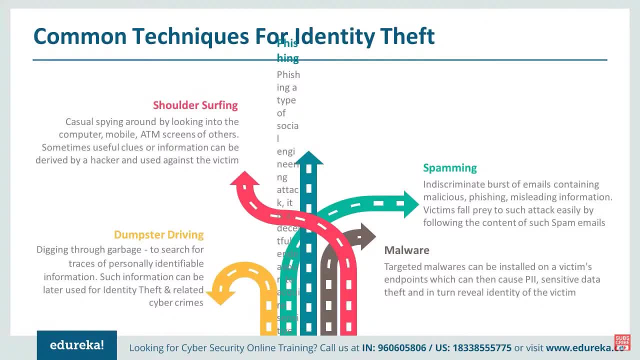 There is an automated process. when the user key in the username and password, the first thing the application will do is it log into the user account and it will change the password. So within hours or within minutes, when you realize that you lost your password, please go and change your password. 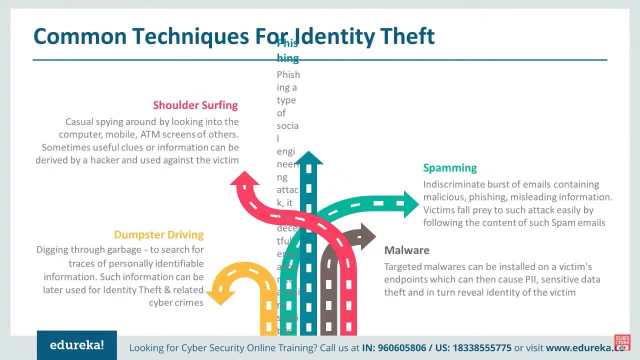 So the malware can also steal it. malware can be installed on a local computer. That can be a spyware, that can be a anything which can spy on you. It will collect your information. It can collect your password, logins, your personal information, anything and everything. so the dumpster diving is nothing. 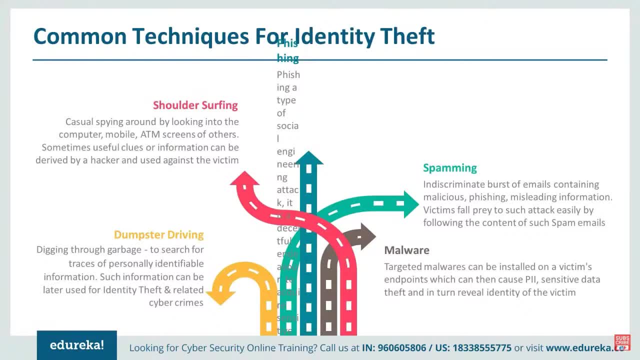 but just searching for your personal information. We can use Google for searching you. we can have a multigo network. multigo, That is a special tool available in Kali Linux That is a community edition. with this We can have a detailed graph of how a person is. who is a person is. 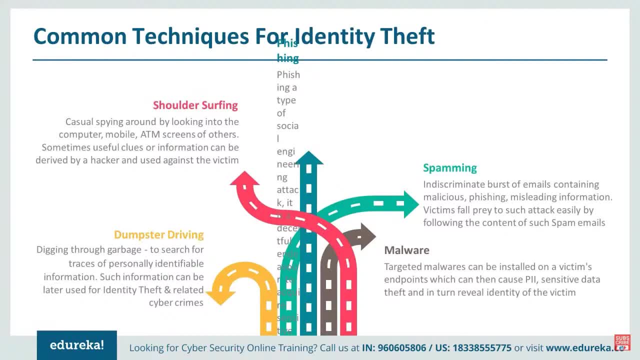 and what is this activity? with limited information, just with an email address and a phone number, We can track down a person. so that is more sophisticated tools and paid software is available on the dark Market that can be utilized for dumpster diving. even Google, simply Google. 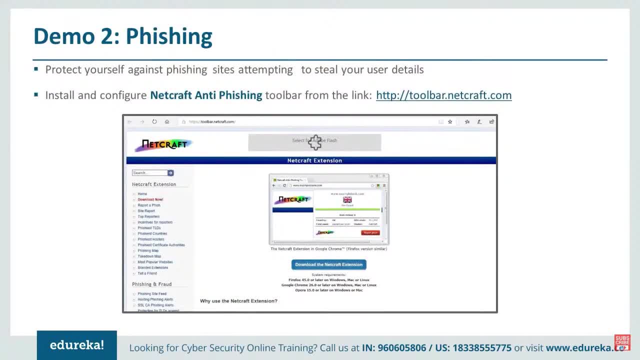 Can be used a netcraft. This is a simply a toolbar or an add-on which can be installed along with your Firefox or Google Chrome. So what actually does is when user visit a particular web page or website, it will alert whether if it's a wrong or malicious website. 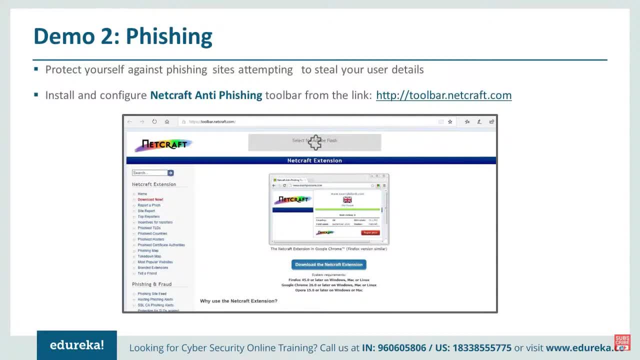 the similar toolbars can be available from McAfee, can be available from Symantec. Avast also has one of the toolbar but a user visit. even Google safe trust Can be enabled when a user tries to visit the wrong or malicious web page. netcraft seems to be not supporting on this one. 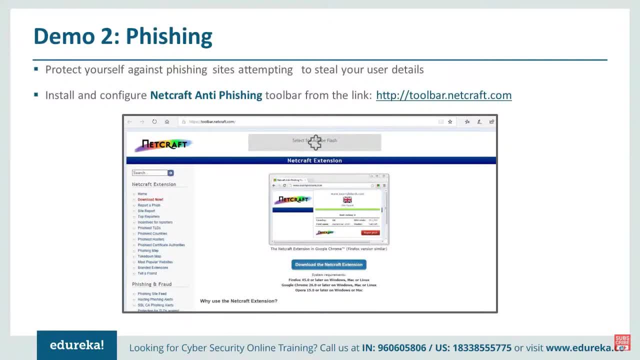 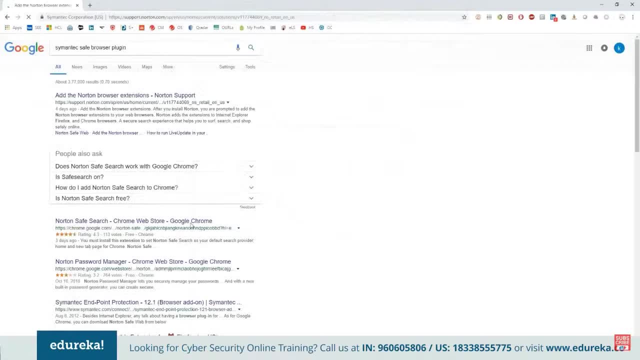 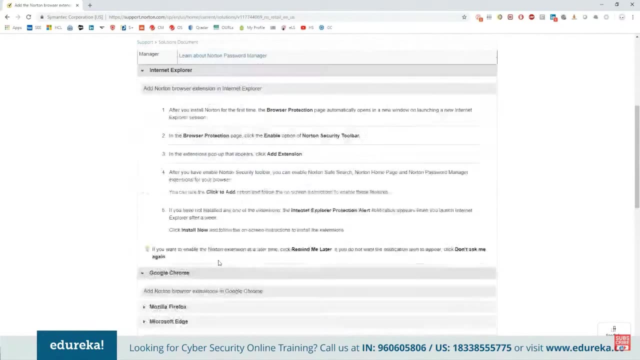 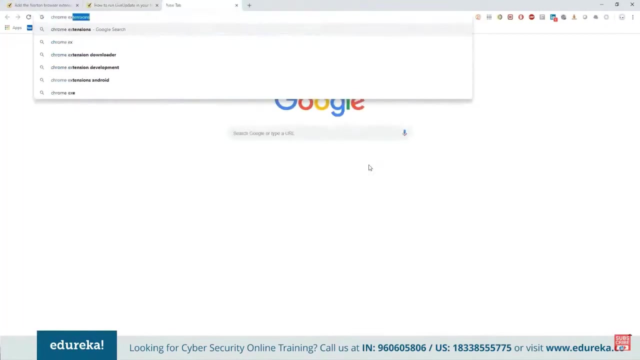 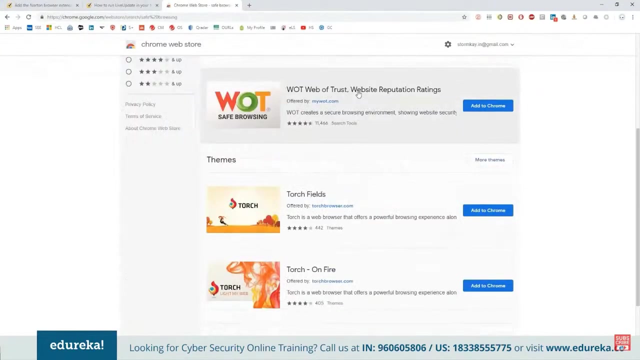 Let me try opening a different browser. I'll go with Internet Explorer. right now, I'm an edge. This is one of the safe browser extension. What it actually does is it needs to be installed using Chrome. So the web of trust is also one more well familiar tool. 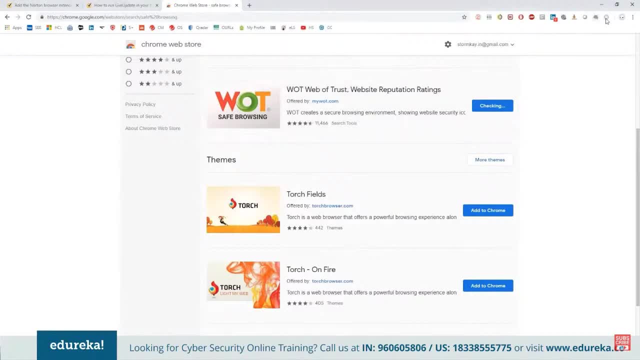 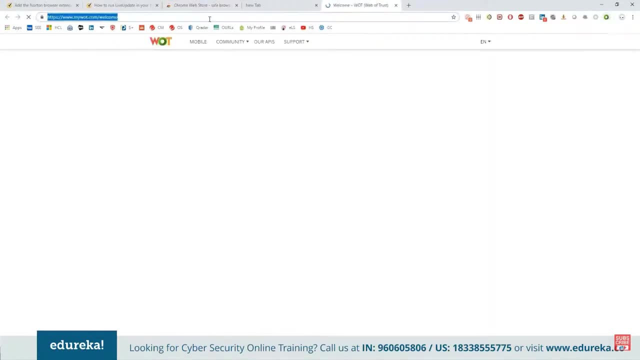 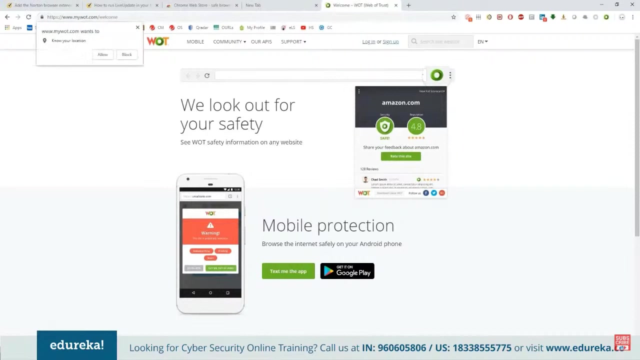 We can add web of trust and extension. It shows the web of trust icon. What actually does is whenever we type some URL. basically, I'm behind a web proxy, So normally I will not be able to visit any malicious website. Okay, I'll try checking it. 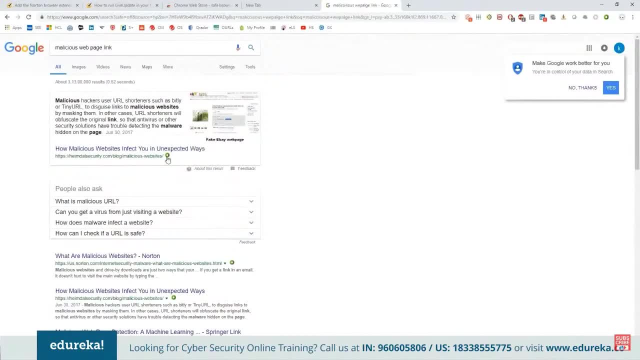 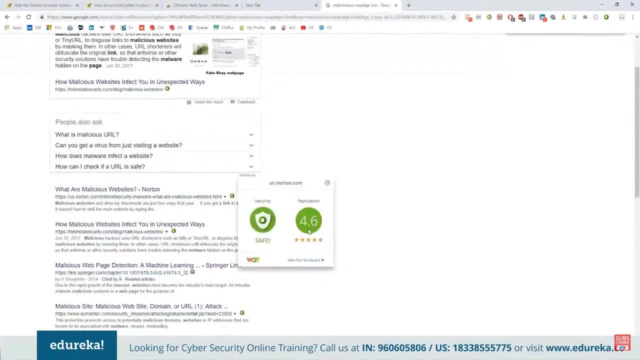 Okay, whenever we search or make any changes, do you see that the green button or green icon says that, whether the link is safe or not, if something is malicious, this site is good based on the rating from multiple people or multiple sources? it will let you know whether the URL which you are